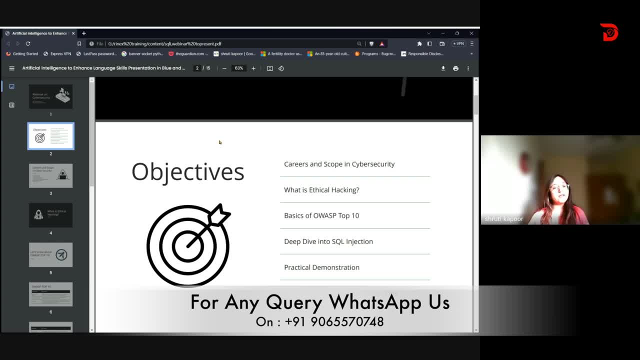 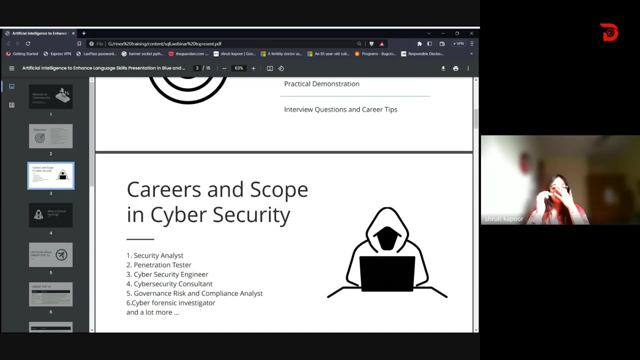 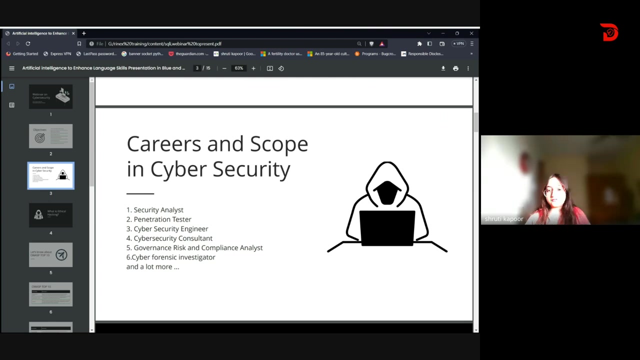 Like it's a very, very old ability But it's still very commonly found in applications, And after that we will do a practical on SQL injection And then I'll explain you some of the interview questions and targets which will be helpful for you. Okay, And after that thing you can ask questions and questions and I will try to answer your question. Okay, all right, So see, okay, so cyber security, like I said, is umbrella domain, So so, so, so these all are the entry level pathways. 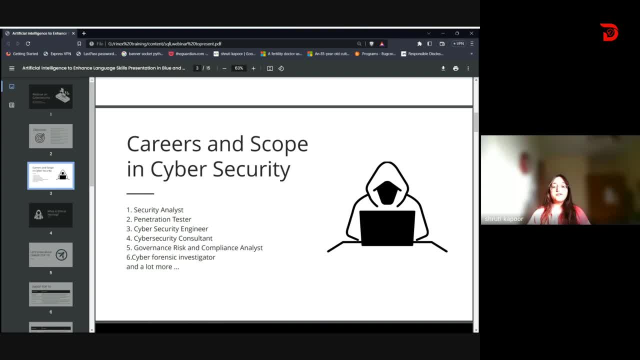 Which are there for the entry level people. Okay, So the first type of career which you can make in cyber security is of security analyst. All right, Okay. Okay, So the first type of career which we are discussing is a security analyst. So security analyst are the people like who are more into defensive side. Okay, So in cyber security we have basically two type of people. One are red teamers, others are blue teamers. 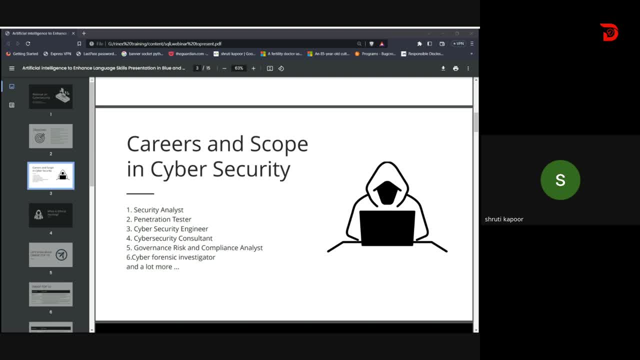 So the people who are into offensive side, they are known as red teamers. because they are, because they are doing the testing work, Okay. And the second type of people which we have in security domain, they are the blue teamers, mean they are into defensive side. So now see, so we have security analyst. So cyber security analyst are the people who are who comes under this blue team. Okay, this means their role is basically to safeguard the inside network. 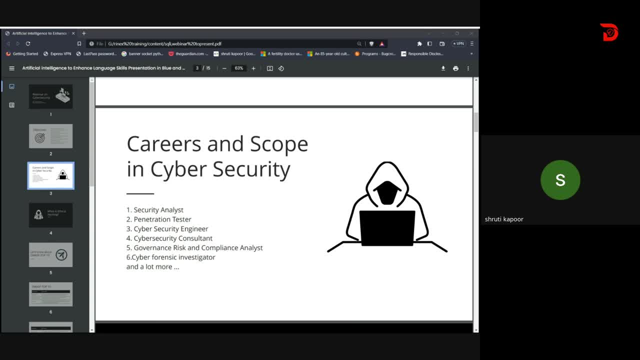 Of the organization. Okay So now, to be a security analyst, you like to. companies expect certain skill sets from you. Okay, So now the first type of skill set which companies are expecting is that you should have a graduation or a master's in cyber security or computer science, For example. if you have done BCA or BSc in IT or BTEC or MTEC, MCA, MSE, then you are eligible to be a security analyst. 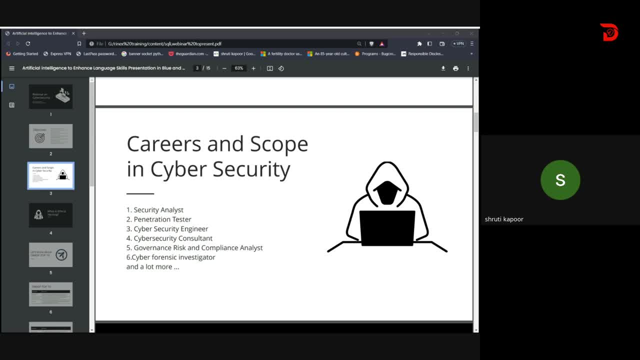 Now the second type of preference which company has for these people is that you should have certification in cyber security, like either you should have CEH or you should have any other relevant certification which will be helpful And like. so the certifications, they tell your credibility that whether you know some set of skills or not, Okay, So that thing is being decided by the certification. So companies have this thing as a criteria, Okay. 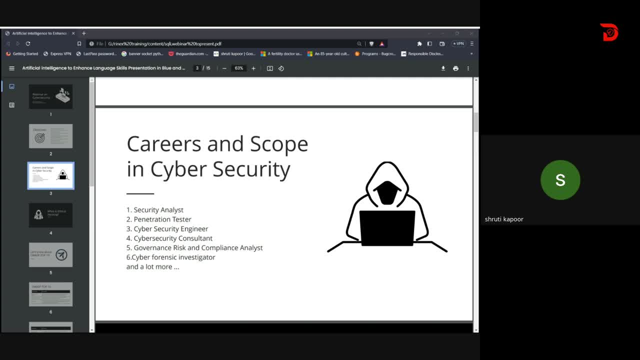 Now the third thing is that you should have awareness. Okay, all right, Jhanshat, Yeah, okay. So now we have another type of skill, which is the companies are expecting you to have some type of hands on experience in any of the same tool. So now, what is a same tool? So okay. so now see all the devices, all the network security devices, like firewalls. we have. intrusion detection system, we have servers, we have. 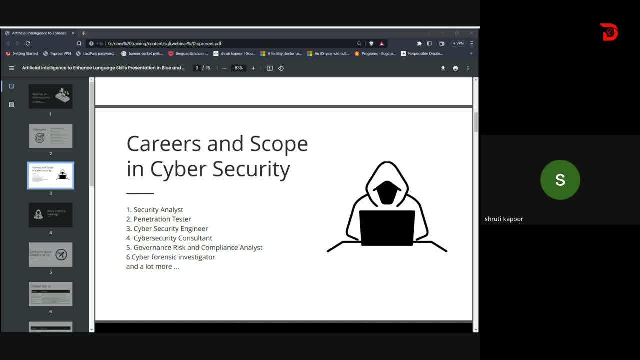 okay, so we have a lot of security devices and all these devices are generating logs. okay, so i hope you people know what are logs. logs mean records of every event or activity which is happening, right? so all these logs, they are being aggregated by this tool. so now the role of a 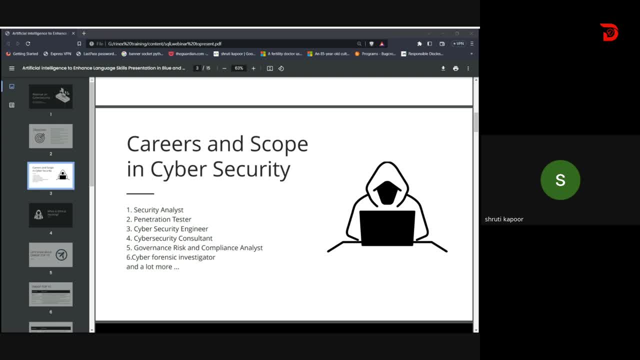 security analyst is to do the monitoring of these logs. okay, all right, so now. okay, so now see, it is very easy to to grab the role of a security analyst because- because there are only some things which companies figure that you should already know mean like you should have a degree. 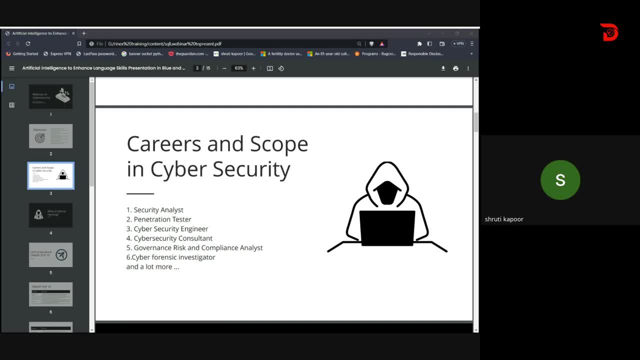 in computer science, uh, you should know basics of uh this soft tool, like how they work, and then you should have at least one certification in cyber security. okay, so, uh, is this first role clear to everybody, like what is expected from your end: to be a security analyst in any company. 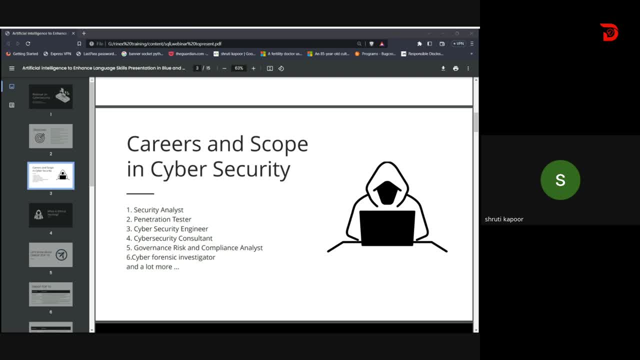 if it's clear to you, then please raise your hands, and if you have any question, please type in the chat box. okay, so now let's move on to second type of career, that is, penetration tester. so penetration tester, so they are the people who are testing the organization's website. 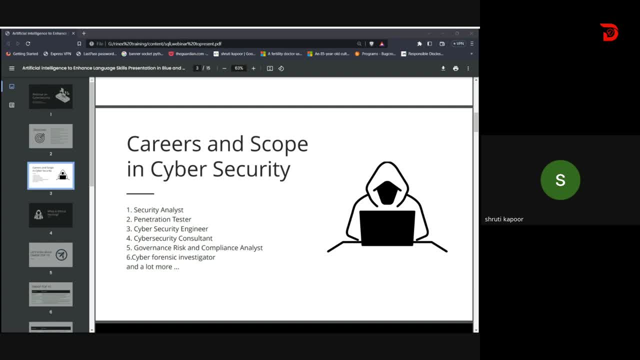 uh, android applications, ios applications, or or we have uh or we have network pen testers. okay, so the role of these people is to do the monitoring of the logs and then they are going to be able to do the penetration test. this means that they are penetrating inside the company's website. 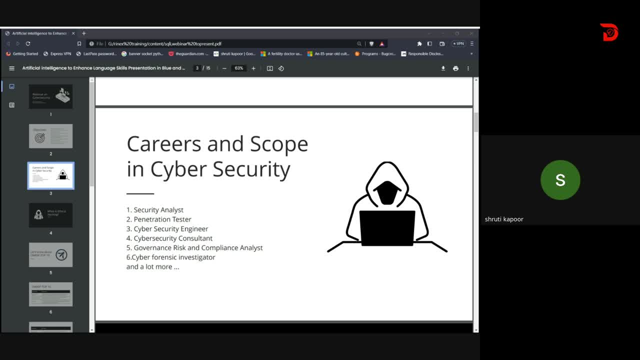 applications and networks, just like a real hacker, to know, uh, to know, uh like what all vulnerabilities are there into this, uh, the system. okay, so now, uh. so now for the skills of penetration tester. the first thing is that that you should have, uh, you should have- your graduation of masters. 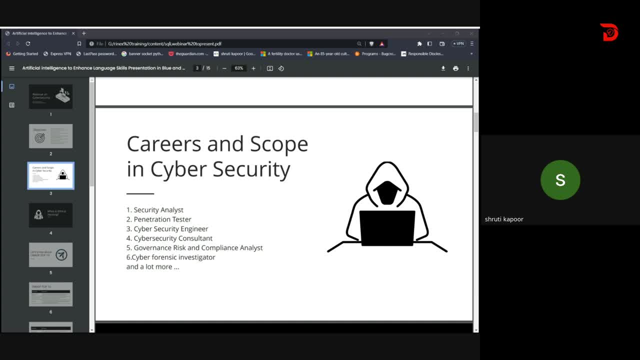 in computer science. now the second thing is that you should have some bug bounty experience. okay, so, whenever you will apply for any role in penetration testing. so companies, they ask whether you have experience in bug bounties or not, because that thing will give you an adder, no matter whether you are getting duplicates, but still uh. but still uh, companies. 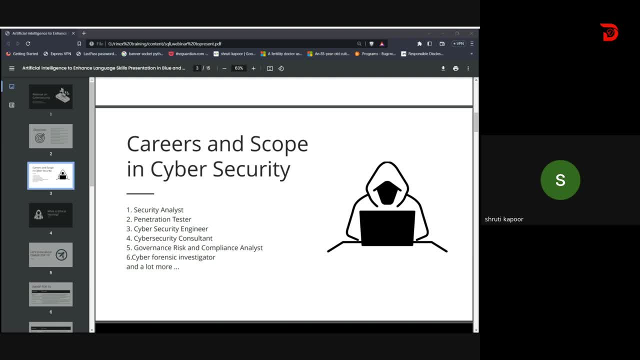 expect that you should have some hands-on in finding the vulnerabilities. now the next thing is: uh, you should. uh, okay, so, okay. so now to be a pen tester, uh, you also require a certification which will prove that you are good at finding the vulnerabilities, for example, ejpt or oscp or cpent. 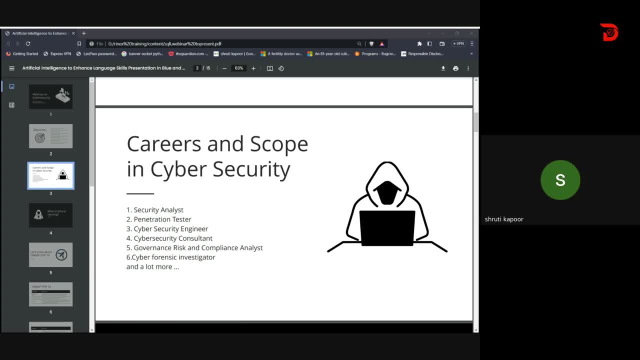 okay, i mean any certification which is giving you certification, uh, on the basis of how is your practical approach in finding the vulnerabilities? okay, all right. okay, so here are some questions, uh, which people are asking about how to start a career in cyber security. okay, see, okay, so these, 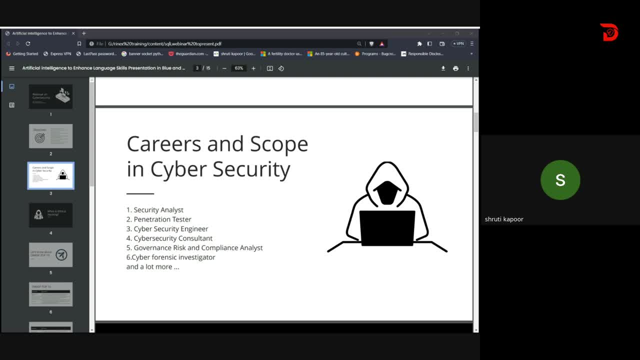 questions. i will answer at the end, but for this thing, i am only telling about these rules, okay, so don't worry, i'll answer each and every question. okay, you just please wait on for some minute, because then our objective will not be able to get completed. yeah, so guys, uh, keep your questions. 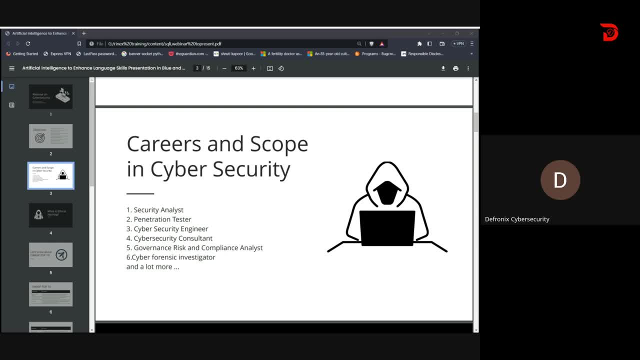 ready, uh, for the end, right at the end, we will be taking a q a session for you specifically so you can ask all the questions that time only, so that we don't waste the time in that q? a. okay, so there will be a separate session at the end of this webinar. thank you, correct, see, you can type. 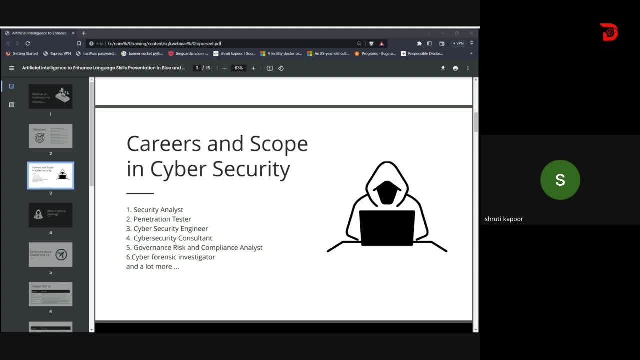 your questions here. so at the end we'll try to answer your questions, okay, so you first focus here, like what we are discussing. all right, so now the next type of career is cyber security engineer. so there are a lot of people- i mean, there are a lot of students- who ask me this question. 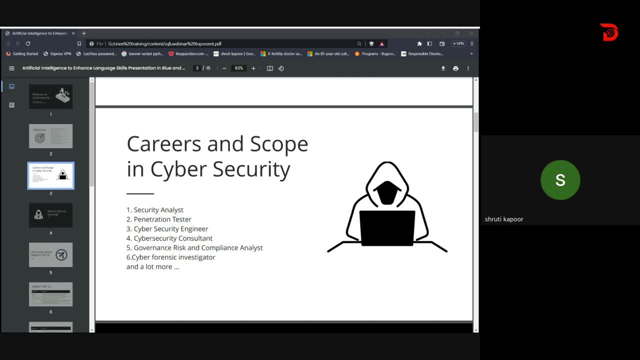 that? what are that? which coding language should we do to go into cyber security? see, to do so. cyber security is a universal domain in itself. so to be a security analyst, you do not require coding skills. but when we talk about cyber security engineer, now to be a security engineer. 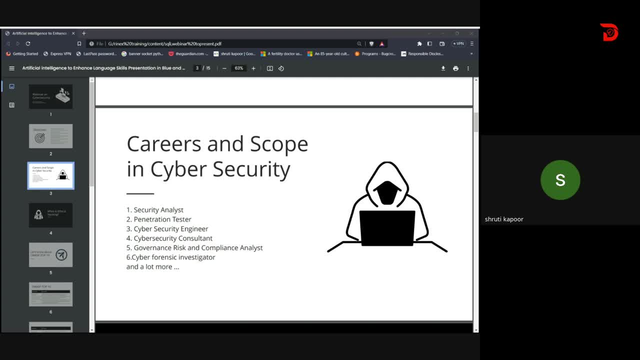 companies expect that you should be proficient in coding languages. okay, because the role of cyber security engineer is a broad role. okay, so there it may also happen that some tasks, uh, so so they can be a penetration tester also for a company and they are also involved in creating. 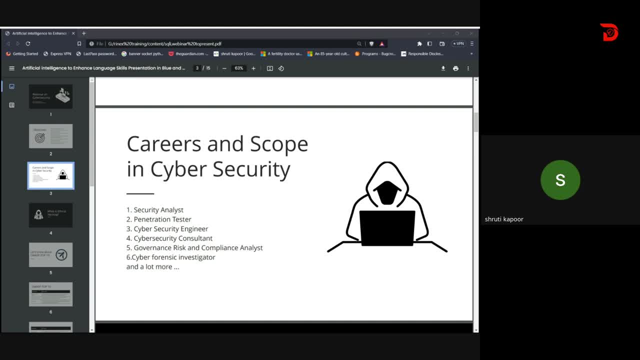 cyber security engineers. so that is why it is expected that whenever you apply for a role of cyber security engineer, you should have your b tech degree or m tech degree, or you should uh. along with this, you should have good knowledge in the programming language. okay, and your projects. they are important when you are applying for the role of cyber security. 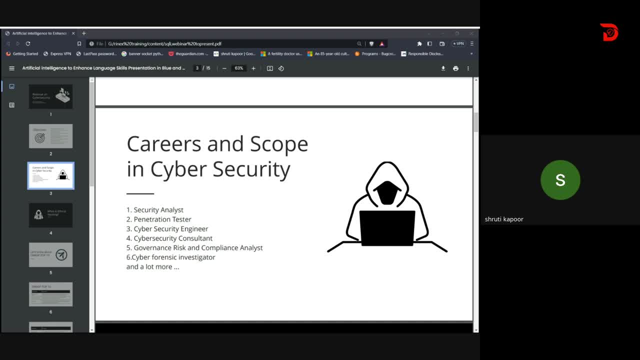 engineer. okay, all right, okay, so i hope this is also clear, okay, uh, so now we have cyber security consultants, so they are the people who are a part of purple team. so now, what is a purple team? like i mentioned before that, we have mainly two type of teams. 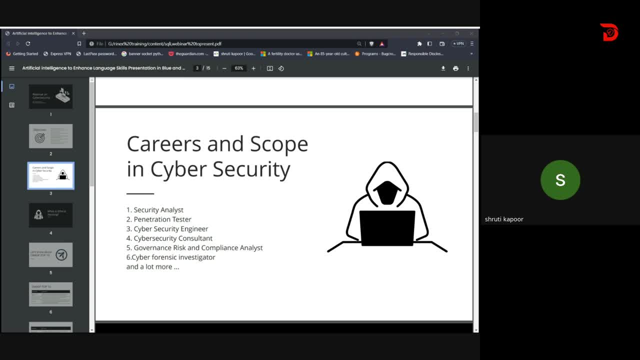 red teams and blue team. right, so red team are the offensive people who are basically doing the testing work, and blue teamers are those people who are doing the defensive work. now, this purple teamer- as the name is telling purple color- is made up of red and blue, so they 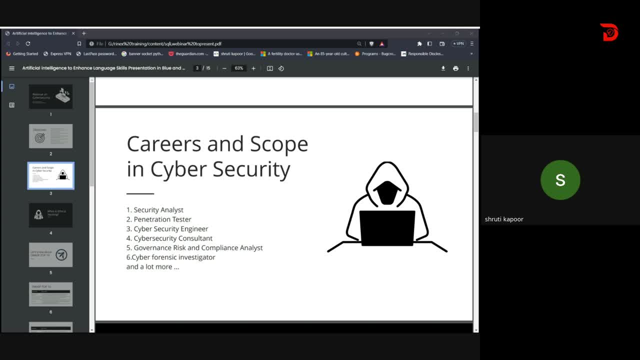 are the people who are working in both the domains according to the tasks given to them by the company. okay, so, so it depends on the type of role company is giving to them. for example, if company has a testing work, they'll give that to the consultant, or it may also happen that the 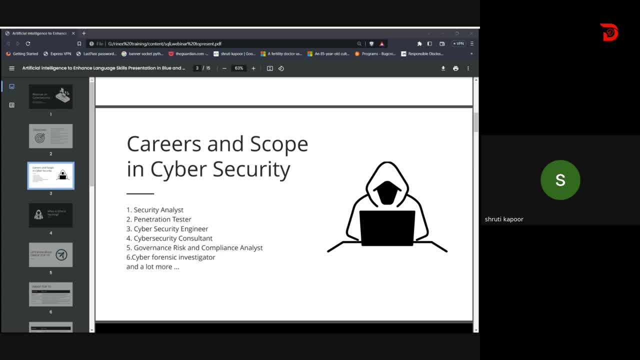 consultant has to create the advisories or the reports. so to be a security consultant, you should have a good technical writing skill too. okay, so now we move on to the next type of domain, and that is governance, risk and compliance analyst. so now, governance risk and compliance analyst is also a career which comes in this. 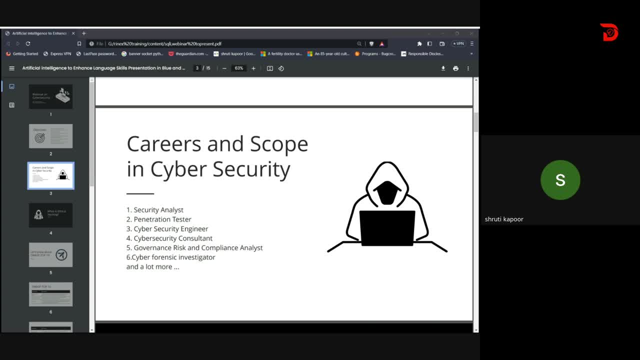 cyber security, and here you only require at least one certification, and iso 27001 auditing certification. uh is yeah, yeah, it's done by most of these students- to go into this domain and along with this, you should have your bachelor's, uh, or masters, in cyber security. okay, so see most. 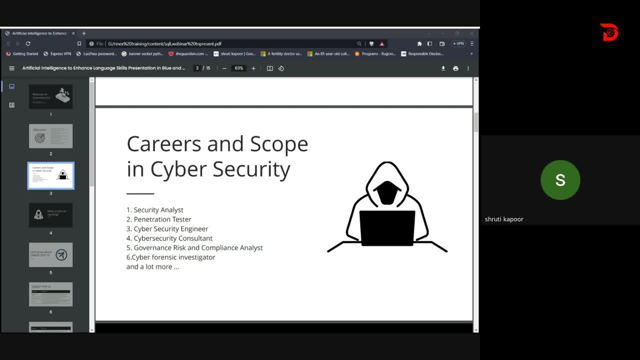 of the things are common, but there is only only change in the certification or the type of projects or language or some some hands-on experience. that thing is differentiating one role from the other. role, okay, and now we have cyber security forensic investigator. so there are, there are the people who are doing the forensic investigations. so 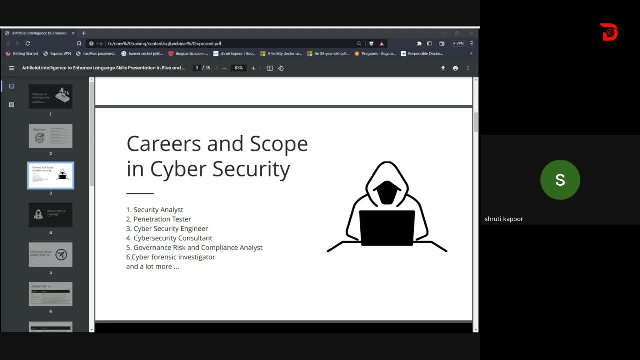 to be a forensic person. uh, you, yeah. so same thing goes for here, and you should have your degree in computer science. along with that, you should have certification or some experience making township in this forensic domain. okay, all right now see, the hardest of all is to be. 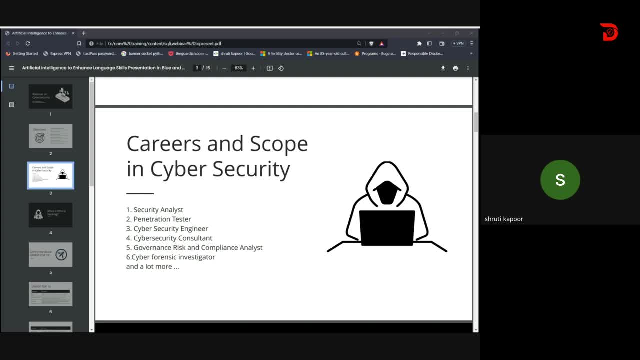 a penetration tester because companies they expect a lot from pressure when they apply for the role of penetration tester. okay, all right, so now we are moving ahead to the next slide. uh, so um, if you have understood something new, then please raise your hands, and then i'll. 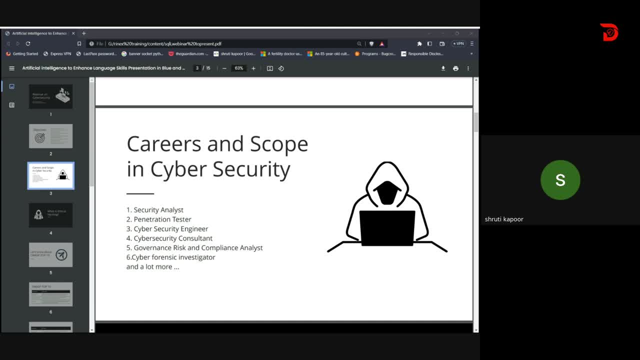 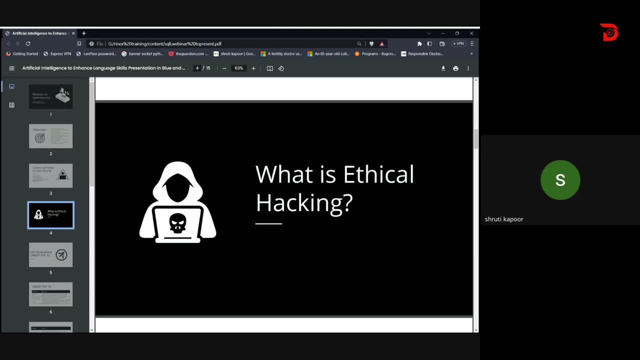 move on to the next slide. okay, that's great. okay, so now i am moving on to next slide. okay, so now we'll see what is ethical hacking, so what? so first they understand what is hacking. so hacking is a practice where the unauthorized access of a system is being taken by the hacker. 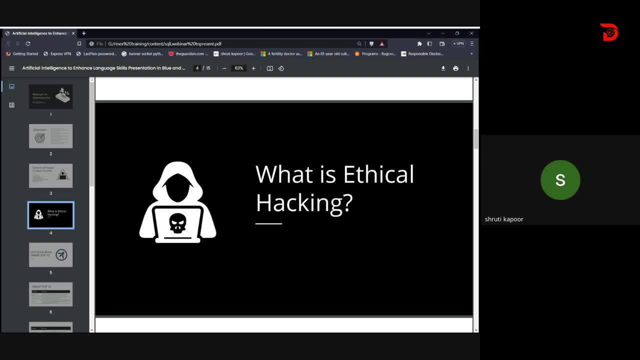 and the person who do this thing is known as a hacker. okay, here the unauthorized access has been taken. so now, when this hacking, when this access is being taken for a legitimate, valid or ethical cause, now this thing is known as ethical hacking. okay, and what is and what is the meaning of ethical cause? this means when we have the new. 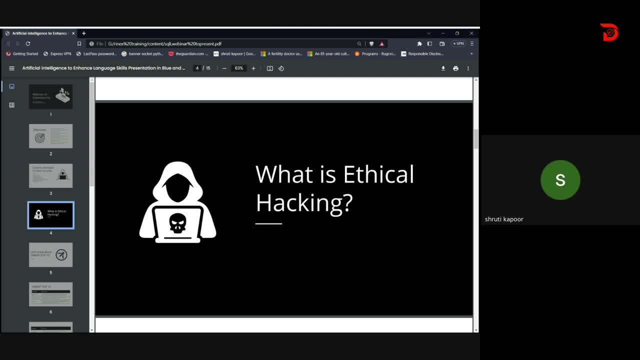 permission of the owner of the site, because we can't start randomly testing any website. so first we need to have the permission that the owner of the site or the company's manager want us to start. then only we will begin the testing work. so when the testing or hacking is done, after the 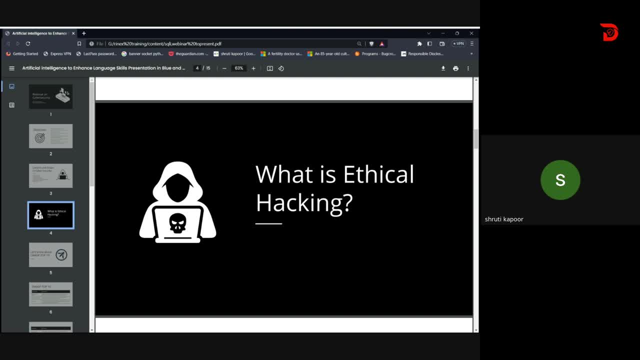 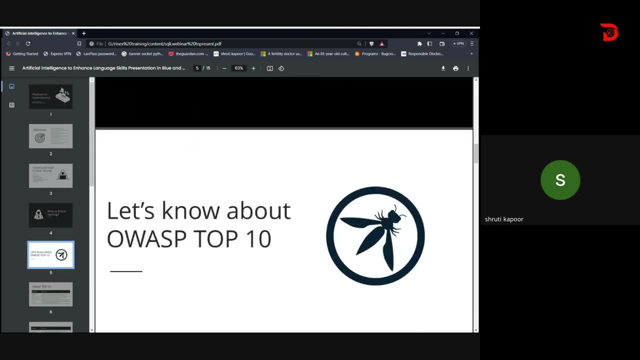 permission set is being taken now. that thing is known as ethical hacking. okay, so now let's move on to the next concept, which is over top 10. so first, okay, so, have you ever heard of over top 10? please raise your hands if you have ever heard. okay, so do you know what is over stop 10? have you ever heard? 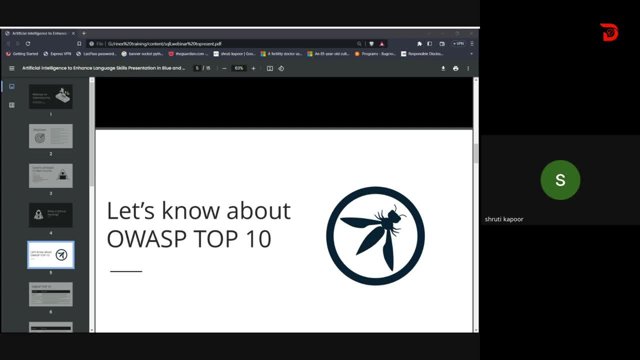 thing. no, you can type in the chat box if you have heard the. not heard, because we are going to discuss it anyhow. so now okay. so now we'll see what is OWASP top 10. so, but what is OWASP? OWASP stands for open web application security project, so 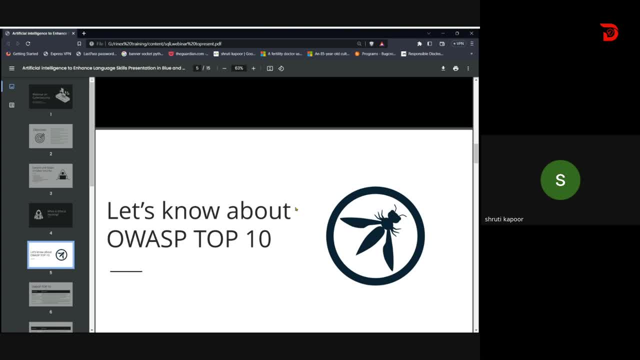 this is our group of people, means organization which is only working on security research and assessments. so this OWASP, so this. so after every two to three years, this OWASP is releasing the list of top 10 most commonly found vulnerabilities which are present inside the web apps, because the main 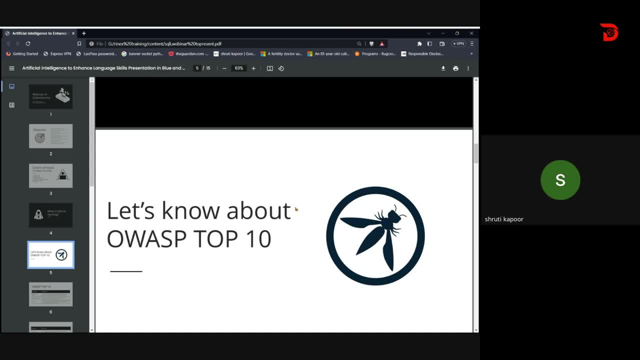 motive of OWASP is to raise awareness to the developers that so that they should, they should follow the secure coding practices and they should that whenever they creating the application, they should parallelly test for the vulnerabilities, if they are existing, into the system. okay, so that's why. so by 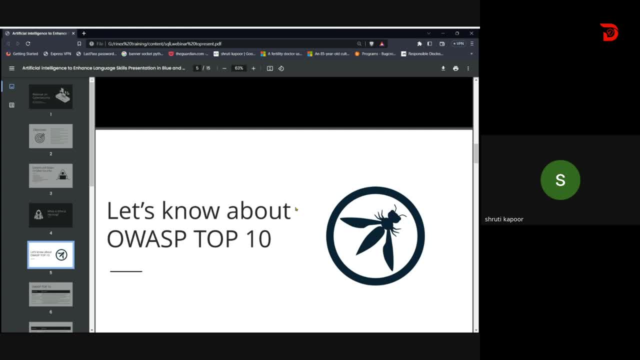 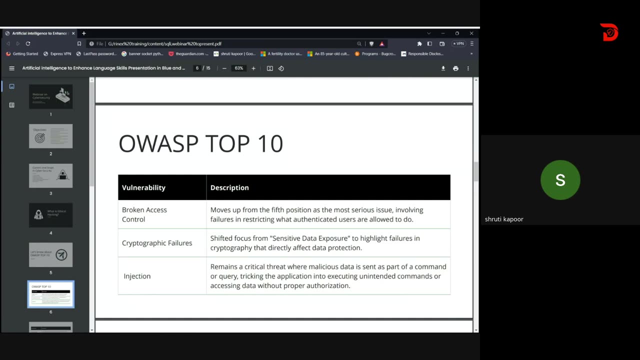 this intent and notion in the mind, this OWASP has. OWASP is releasing top 10 most commonly found vulnerabilities after every two to three years. okay, so now? okay, so now. these are these. these are some of the vulnerabilities which are there in OWASP top 10. so the first is broken access control. then we have cryptographic. 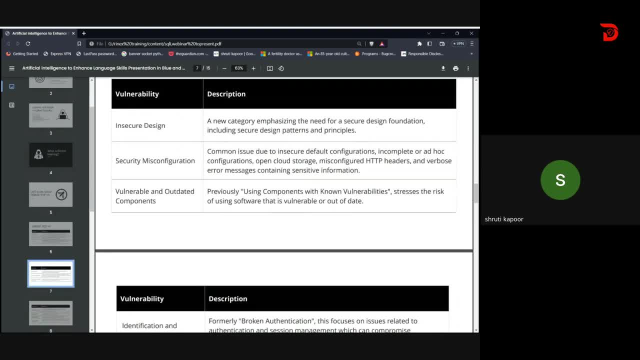 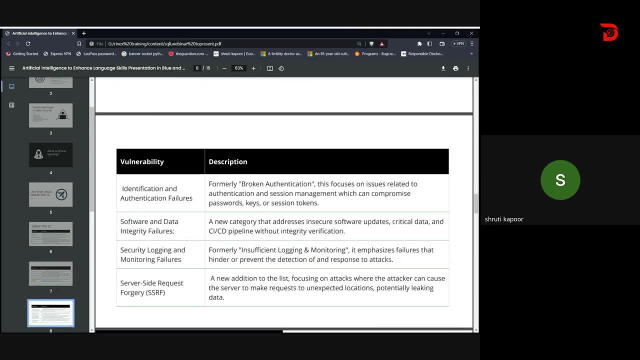 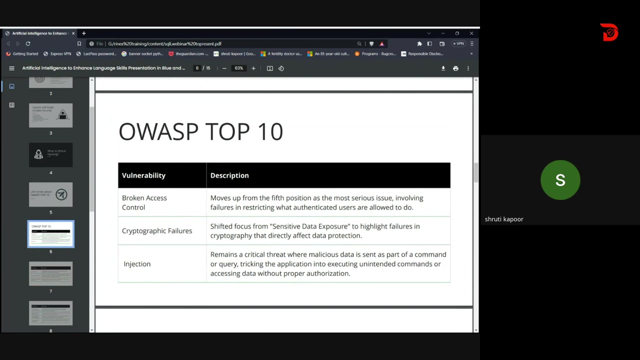 failure. then we have injection. we have insecure design, security misconfiguration, vulnerable and outdated configuring, so we have all these vulnerabilities. We have identification and authentication failures, software and data integrity failures, security logging and monitoring failures and SSRF- OK, All right. OK, so till here, have you understood. 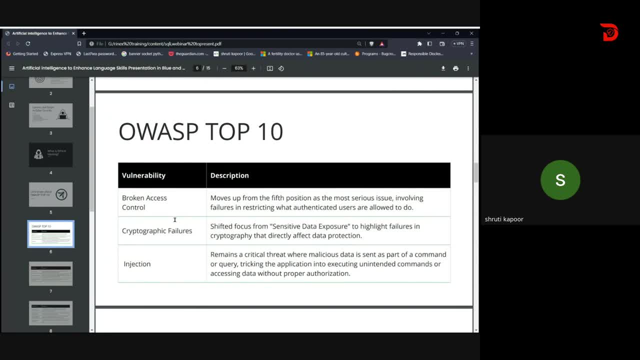 Now. now I'll explain you what all these vulnerabilities are and then we'll deep dive into SQL injection, which is one of the part of injection vulnerability. So if you have understood this concept, please raise your hand so that I can know that you have understood. 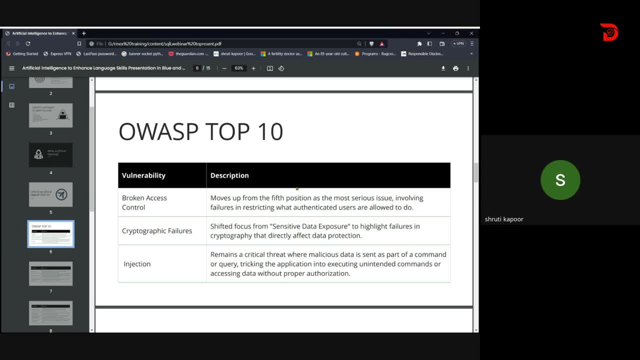 So now I'm proceeding. So the first is broken access control vulnerability. So I will explain you this vulnerability with the help of a simple example. Suppose you are in your university and you are accessing the learning management system of your university. OK, And now your faculty has the permission to upload the content. 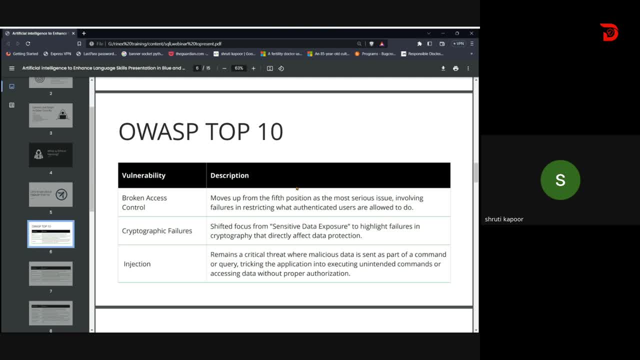 She has the permission to manipulate your attendance. OK, And now you are in your university. Now you can only view the attendance and you can only download the content to read. Now, for example, if the website had some problem because of which you are able to upload the content and you have the right to change your attendance too. 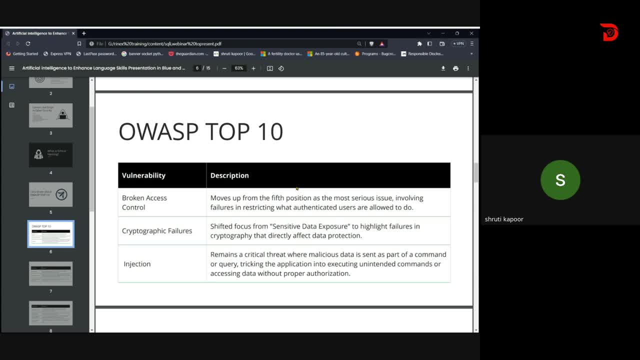 So that thing is a flaw, It is a weakness and it's a vulnerability. OK, So this type of vulnerability where you are able to access those things for which you are not able to access? OK, So this type of vulnerability where you are able to access those things for which you are not able to access. 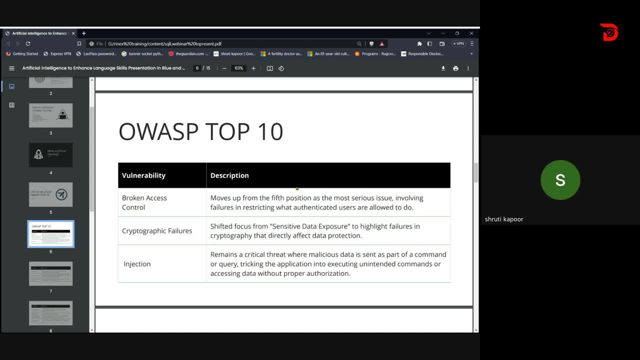 OK, So this type of vulnerability where you are able to access those things for which you are not able to access, So that thing is known as broken access control. OK, so in this broken access control vulnerability, we are discussing both right for vulnerability, where we are dealing with the access, that, who are the that that, what authenticated persons are allowed to do what things? 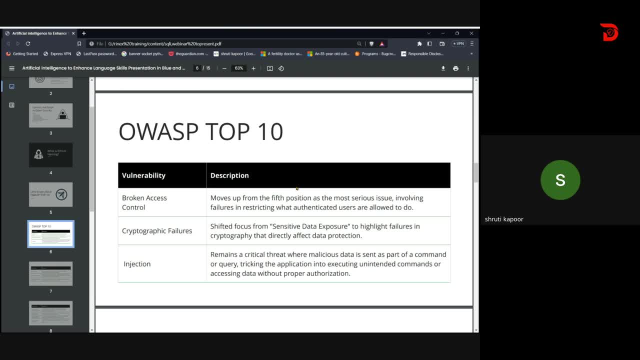 So this thing is there and this vulnerability which is broken access control. OK, So now the second type of vulnerability is cryptographic failures. So here, so earlier this vulnerability was known as sensitive data exposure, but now its name is converted to cryptographic failure. 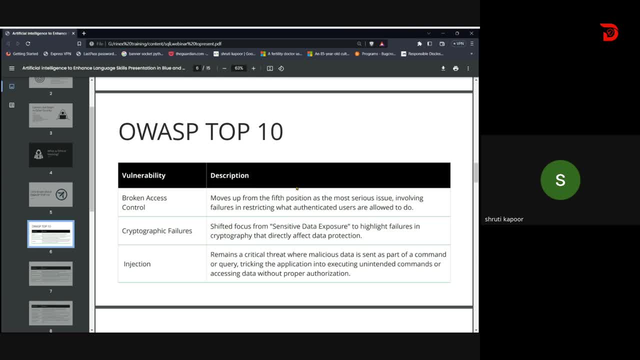 So we know that. OK, so we know that. what is cryptography? So it's an art of converting a data to non-readable format and then to convert it back from the non-readable form to a normal form. OK, so here, basically, we deal with two functions: encryption and decryption. 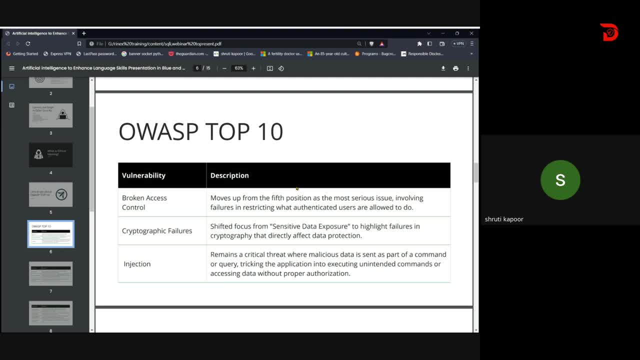 Now encryption: we are converting the data from normal plain text form to our encrypted format or a non-readable format to maintain the confidentiality. So I guess everybody knows that Entire base of cybersecurity is laid on two, three things. They are confidentiality, integrity and availability. OK, so so the CIA is like a sun. 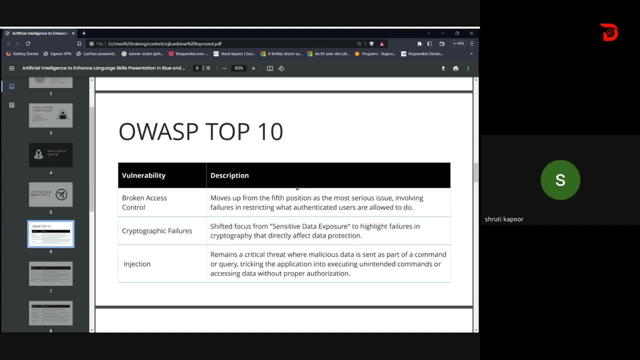 At the center and all the vulnerabilities. they are revolving around the CIA. OK, so now. so now the so, now, what's happening in this cryptographic failure? So, in order to prevent- OK, so, for example, if there is a website and that website is storing passwords and passwords are, and to store the passwords, strong hashing function has not been applied- 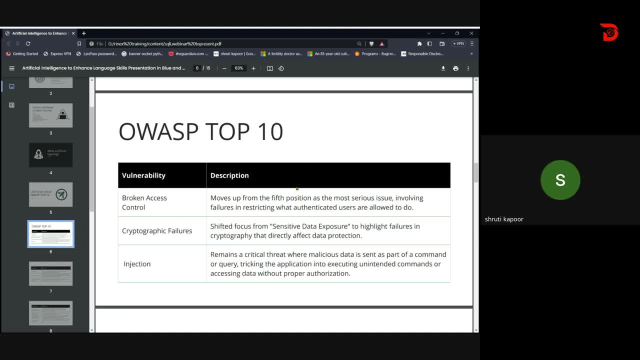 Or if the site is Running on HTTP and not on HTTPS, OK, And there are a lot of things which are there in this cryptographic failure, vulnerability, But I guess, basically, it's clear to you, It's clear to you all, that please raise your hand. 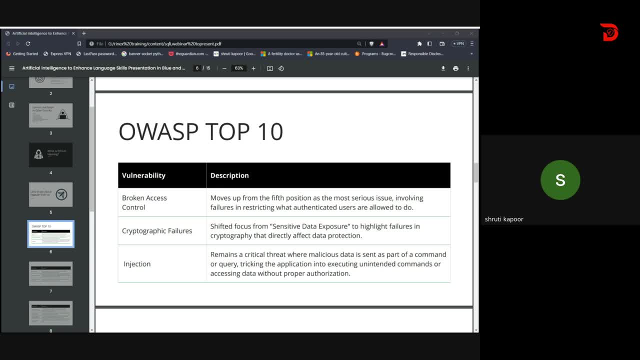 OK, so somebody is asking who wants to stop Any time to do it. OK, so the recent to 20, 20 months. OK, so now the list for the 2024 of our stoppen has not been released. All right, 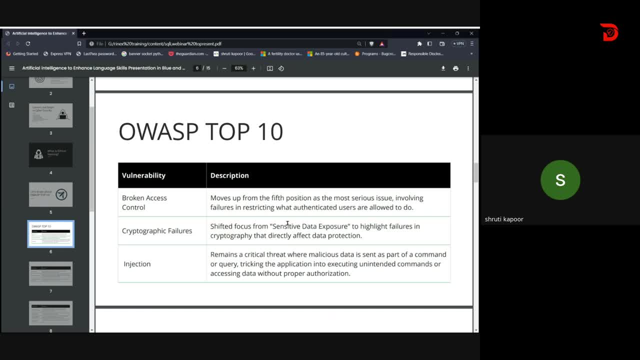 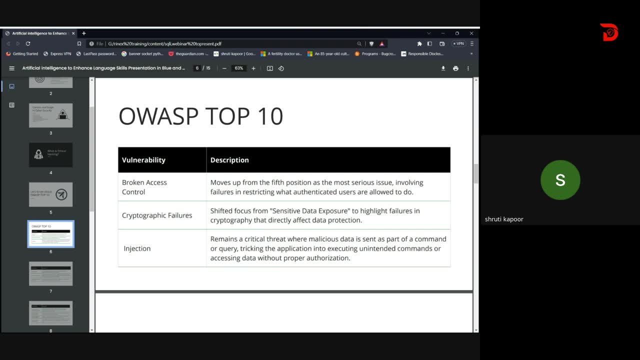 OK, So okay, yeah, so i think i should continue and then question will discuss at the last. now the next vulnerability is injection. so injection in itself is a broad category of vulnerability. here we have a lot of vulnerabilities, but the concept of injection vulnerability is same. 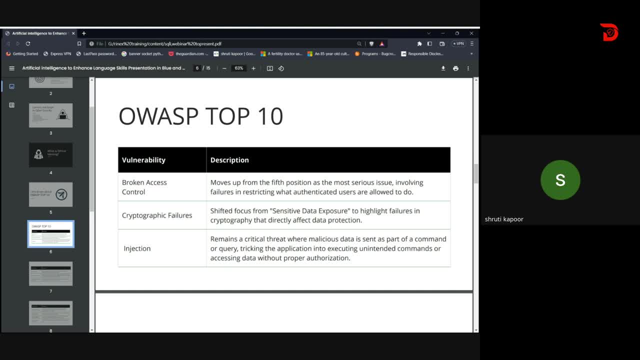 in every type. so now, what is the meaning of injection? okay, so now let's understand this with a very simple example. uh, so you, you are ill, for example, and you went to doctor. now doctor is: uh, is injecting something inside your body. okay, so that you will get recovered soon. so, so so. 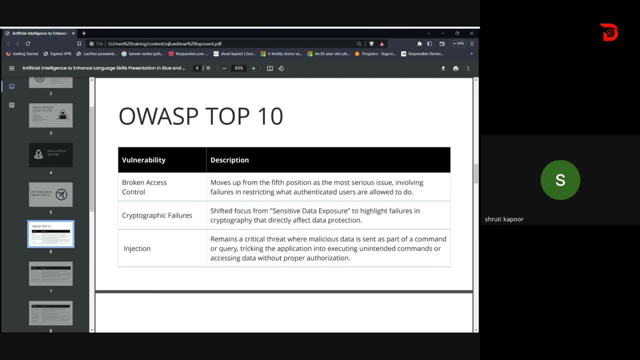 the thing which is getting inside your body and uh, and now your body is reacting to that vaccine, right? so in injection vulnerability, what is happening? we are injecting, we are inserting some payloads or some code or script inside the entry points of a website. now, what are entry points of? 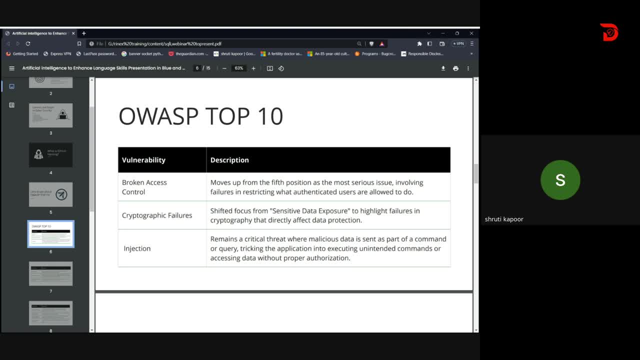 a website. so entry points of the website are the points from where you can enter, like you can enter something. for example, if you talk about search bar, you can search something over there, right. when you say forms, you can type something in the forms. when you say comment section, 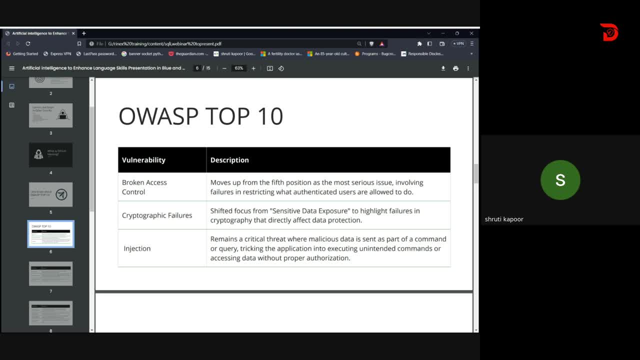 you can type something in the comment section, right? so they all are the entry points. so now in injection vulnerability, the attacker is is looking at all the entry points, right? so you are injecting all the items and you are Strangtel, and you are right now injecting all the items and you're disrupting the integration process in this will act as: 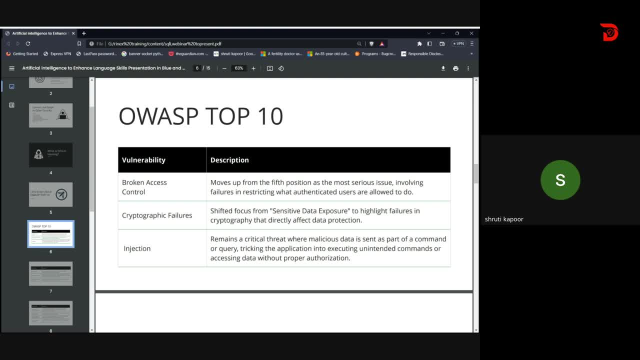 if you can produce這些 ALLATRA INJECTIONS, the person who is thought a legitimate one Now here. you can see that. so it's a critical threat where malicious data is sent as a part of command or query and where the application is getting. 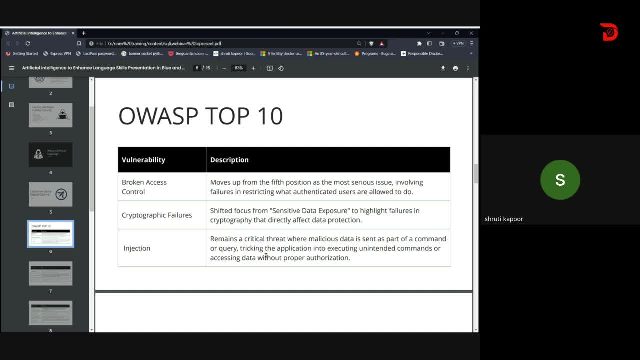 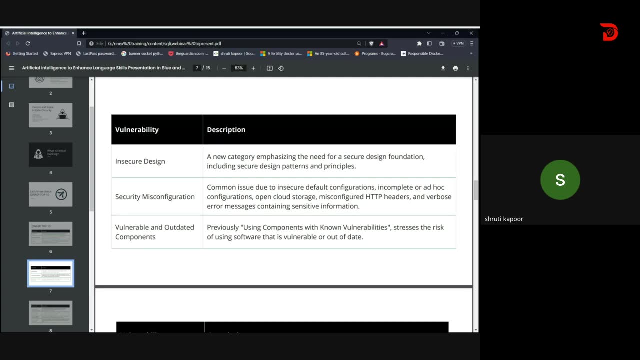 tricked and unintended or malicious commands may get executed without the proper authorization. Okay, so I hope it is clear to everybody. So now, okay. so now let's move on to the next vulnerability, that is, insecure design. Okay, so, okay. so now let's understand this, also with the 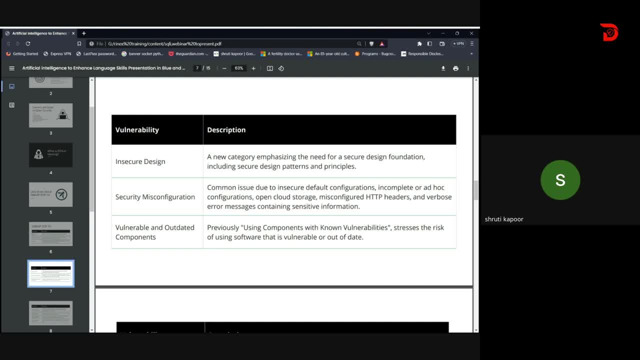 help of a simple example. Suppose you have bought a home. okay, and you have. okay, you have bought a home, and now you have applied, and you have, you are using CCTV cameras outside your home. You have a security guard also, which is which you have kept to safeguard your home. You have mean, like you are. 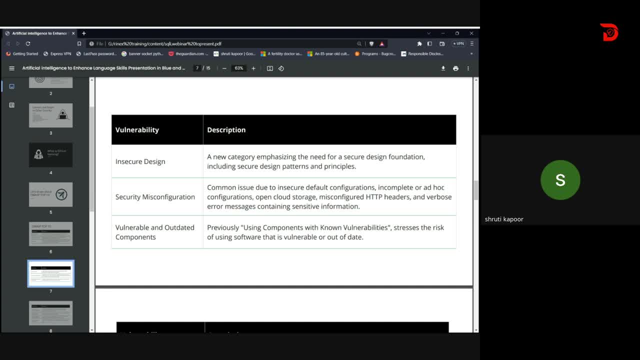 trying your best to protect your home. You are trying your best to protect your home, You are trying your best to make your home safe, but now, in reality, what's there? so there are some secret stairs inside your home which are connecting your home to some, to some random area which is not a. 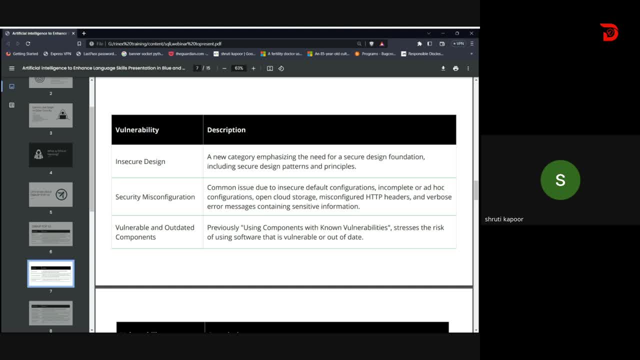 part of your home. Okay, so now? so now, such type of flaws, where the problem is with the design, So those type of vulnerabilities, they, they come under this category, which is insecure design. So here, in order to avoid these problems, the developer should follow secure design practices and 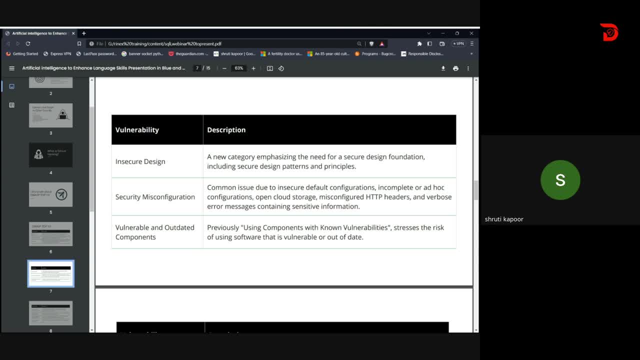 principles. okay, Alright, so I hope this vulnerability is also clear to everybody. so till, here are the people with me. are you getting now the next type of vulnerability, security misconfiguration. So, as the name is telling, misconfiguration. so here we are discussing is a large amount of small, small issues which are like. So which are the vulnerabilities which are? 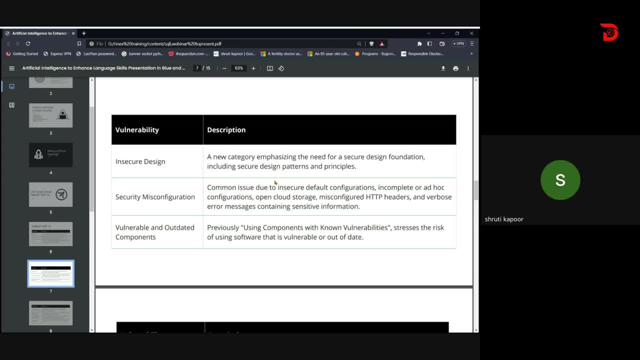 so which are creating a big, big impact or which may cause a big damage to the organization. For example, like if we have bought a router and a router is running on default passwords- okay, so now what may happen? that some unauthorized person can also enter the default id and password. 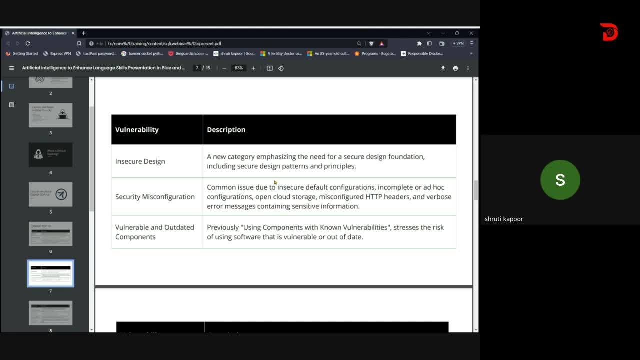 or to connect to a network. okay, so this is a problem and such type of issues, they come under security misconfiguration. So this is a problem and such type of issues, they come under security misconfiguration. that these issues- I mean their implementation- is simple. but but when they're not implemented, 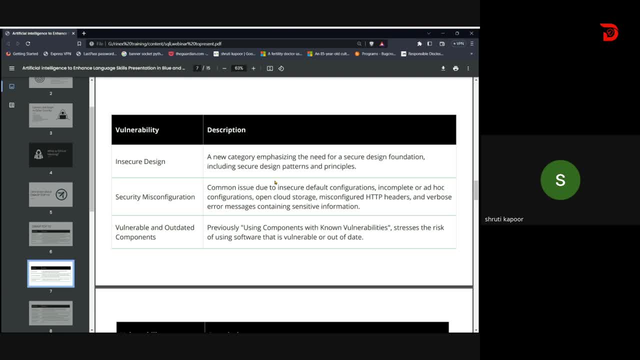 properly means when they, when they are not configuring a device properly. now, Yeah, so now uh, this is uh. this is a dangerous type of thing and and can have a huge damage on the organization's network. You can take the example that there is a company who is using 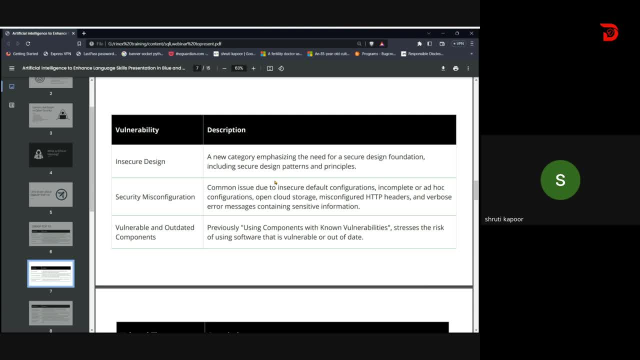 a router or who is using IP? uh, or he is. who is using cameras? okay, Whoever uses IP, can those cameras and those routers. they can simply enter default id and password. default id and password, like admin, admin, and they can also access the cameras which are there inside the company. 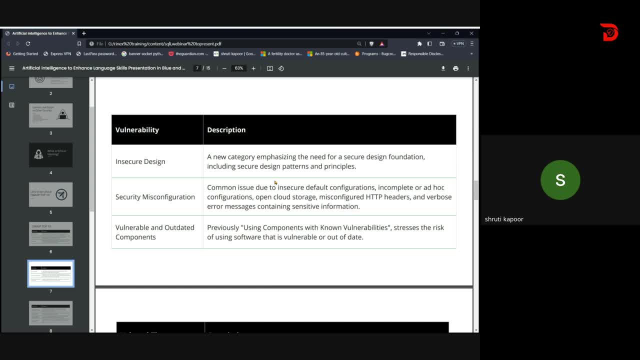 to monitor the employees, okay, so it's a sensitive vulnerability which need to be taken care of. so that's why. so that's why the default credentials should be changed whenever some new things are being bought. so here we have a lot of vulnerabilities which come under this. 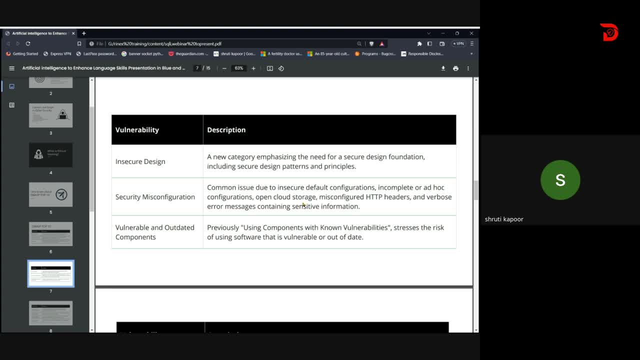 broad category of vulnerability, which is security misconfiguration. okay, now we will move to next vulnerability, that is, vulnerable and outdated components. so, as the name is telling that, here those, those components of any application which are outdated and vulnerable, they can have like so when a vulnerability is. 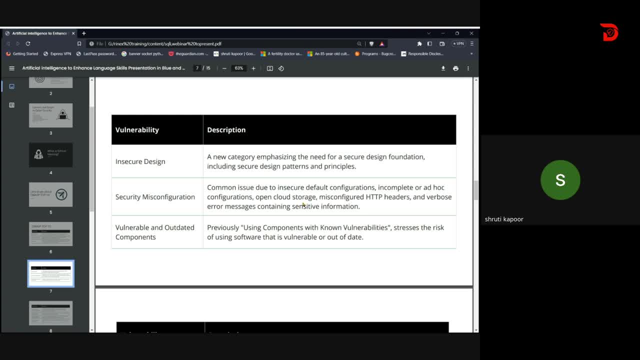 being exploited now, it can have a huge damage or huge impact on the organization's network. okay, so, for example, if, uh, if there is a company and that company is using uh old python version for its applications, okay, and now, for example, and that python version is uh python version. 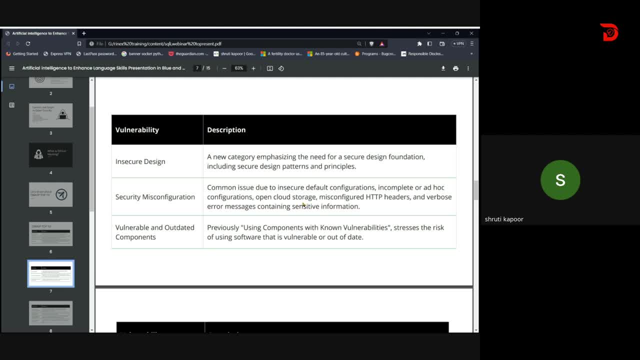 has a vulnerability, that is, rc remote code execution, uh. so what may happen? so attacker can control uh, the control the application from his place. okay, only because the version of python was vulnerable. so that is why it is recommended that whenever any update, uh is being is being. 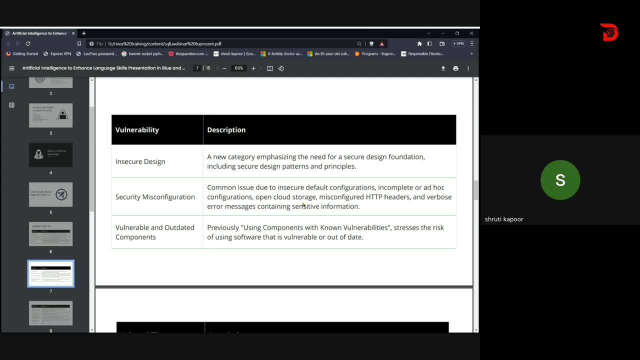 launched by the company that we should, we should update and upgrade our systems at that moment of time only. okay, all right, so here you can see that. so this is addressing the issues which are stressing the risk of using software that is vulnerable or out of date. okay, so i guess it's also clear to everybody. 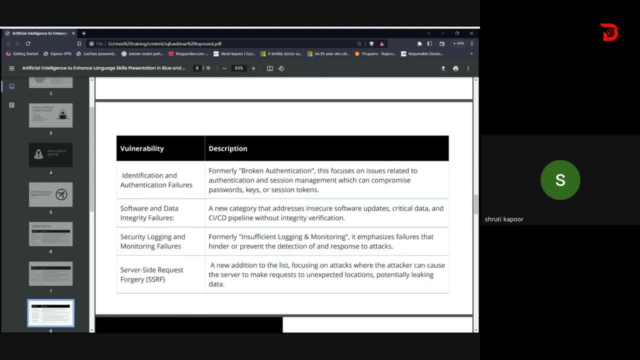 so now we are coming to next one, that is, identification and authentication failure. so, as the name is telling that this, this little harm, was properly Strahd in mind, okay, so, yeah, so it's also very broad category, we uh. so it may also happen that uh. 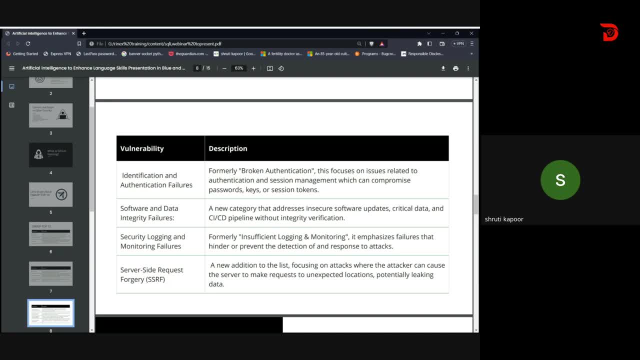 that there is a company and that company is using two-factor authentication to safeguard its website. okay, and now attacker is bypassing 2fa. there is some problem with the 2fa implementation, or there is some problem with the, or there is some problem with the open authentication. 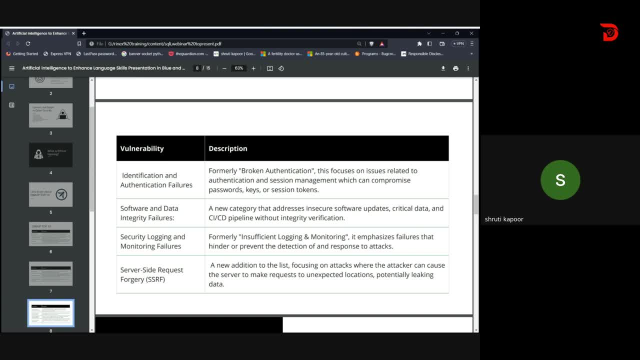 which is being used, okay, so. so such type of issues are being discussed or are being addressed under this broad category of vulnerability. now comes security, now comes software and data integrity failures- okay, so it's a new category which is uh, which is recently addressed, and the and this vulnerability is uh. so here also you can see that uh. so here we are discussing. 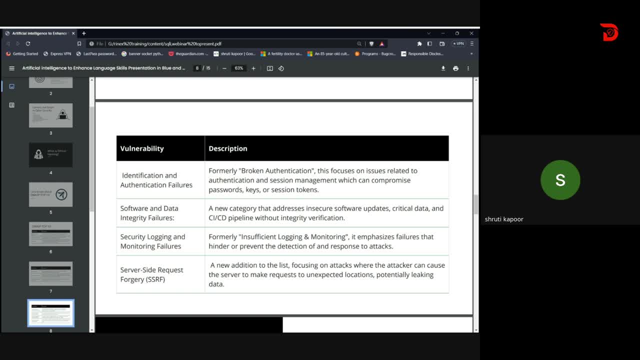 about the uh critical updates, for example, if there is a software update and that update in itself is not a secure one. okay, so such type of vulnerabilities? they are discussed under this category, which is software and data integrity failures. so what is integrity? meaning of integrity is that the data is from the authentic or a genuine source. 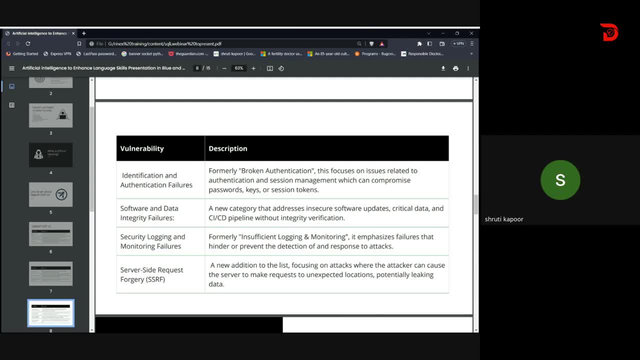 okay and whatsoever we are. for example, if i am sending hello to my friend now, my friend should receive hello as a message. it should not be the case that there is some person who came in between, who has intercepted the communication, and that person is sending by, okay, and now my friend is feeling that that i sent by, but in reality i sent hello, so it 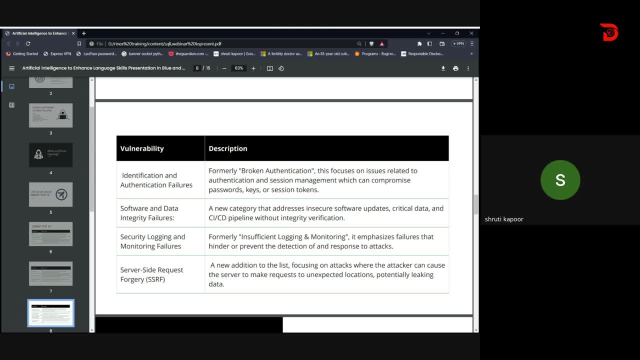 is an integrity failure issue. so such type of issues, they are addressed under this category of vulnerability, which is software and data integrity failures. now, the next vulnerability is security logging and monitoring failures. so, uh, okay. so now, uh see, it is important for every company that they should enable this feature of log logging. uh, logging, log generation. 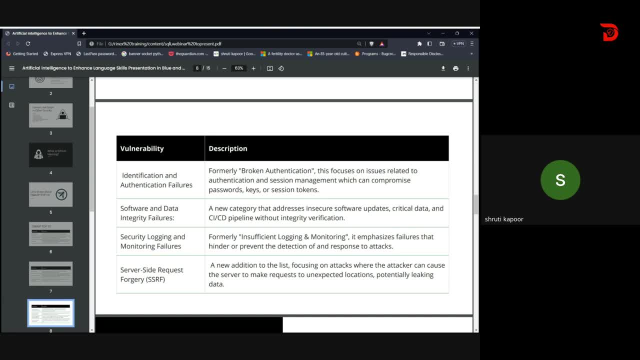 and log monitoring, because, uh, because logs are the records that at what time, from what ip, what person tried to do what. so all these activities, they have been tracked as a log. okay, so now, uh, for example, there is a company and now they do not have, uh, the mean they. 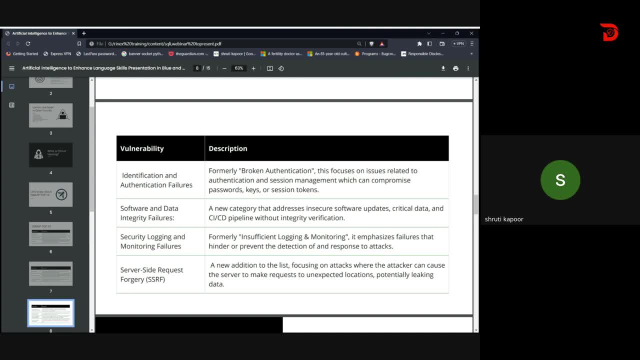 do not have a setup to capture the log or to monitor the logs. so now, when this thing is not there or if it's not properly implemented now, it is very hard to detect the attacks. it's very hard for the blue team guys to uh to to provide a proper response against those. 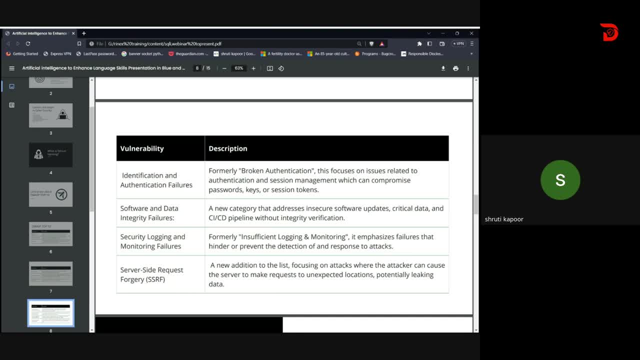 attacks. so such type of vulnerabilities, they are addressed under this category. so they are not protected from the security of the data integrity failures, which is why this address under this broad category, which is security logging and monitoring failures. okay, now the next one is ssrf, which is server side request for dream. and now what's happening? 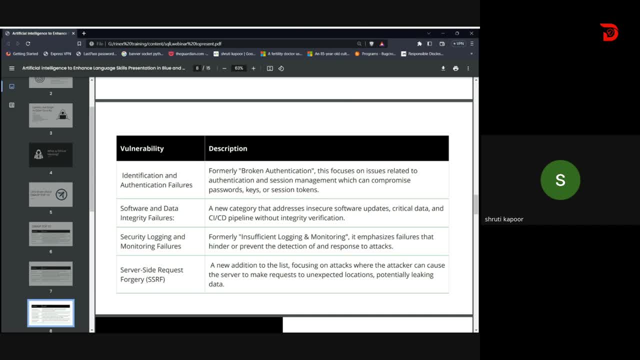 in ssrf and ssrf, the attacker is forcing the server to make requests to an unexpected location. okay, and because of that thing, i mean a lot of data can be leaked or disclosed to the attacker. so these are the top 10 vulnerabilities which are most commonly found in uh in web applications. 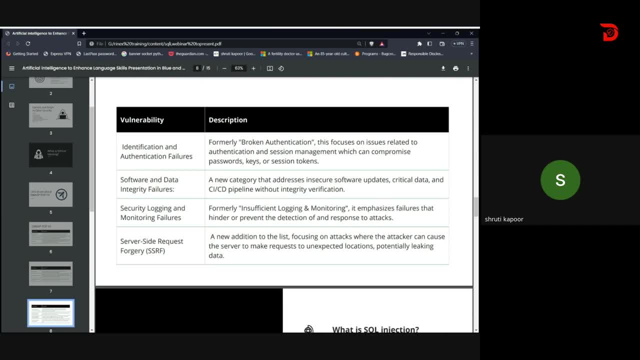 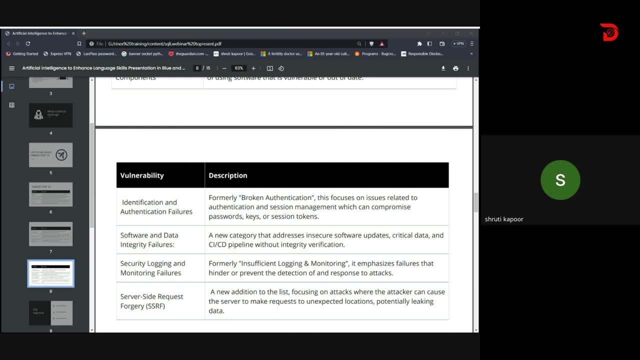 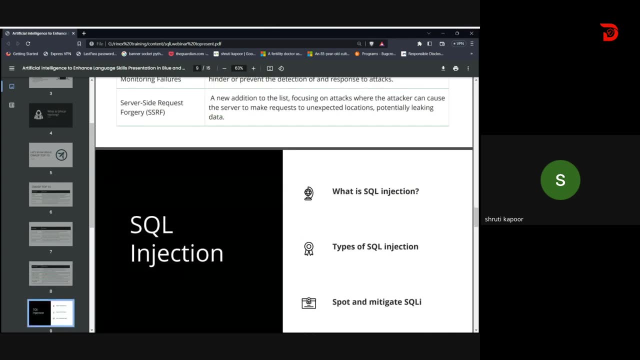 okay. so i hope you people understood this thing. anybody having any confusion, please, uh, raise your hands. if you have any doubts or problem, or if it's clear to you, then please write. it's clear to you all, right, so now? okay. so now let's come to sql injection. 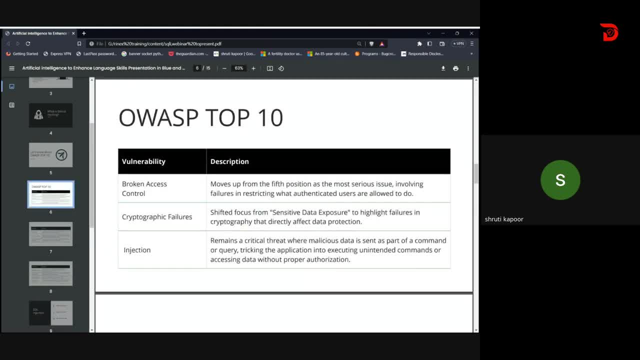 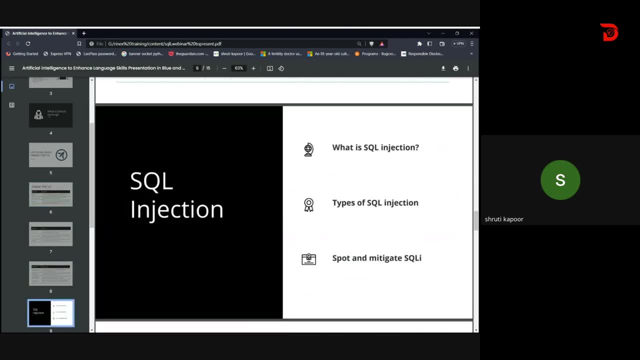 okay, so there i explained you that injection is a broad category of vulnerabilities, and so the okay. so now, today we will discuss about sql injection. so now, what do you mean? okay, so now, what is the rule of sql in our date, in our web application? okay, so i'll explain this thing. um, just give me a minute. 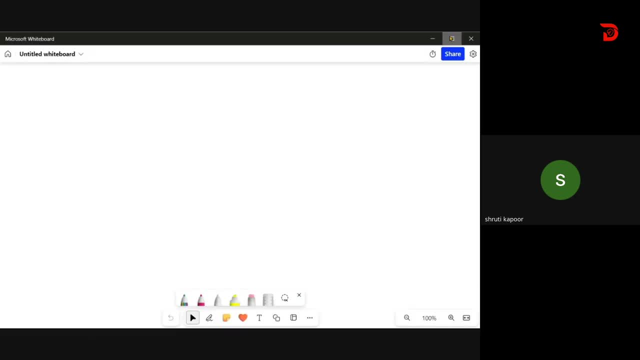 and i'm sharing my whiteboard. okay, okay, that's great. okay, so here you see, uh, okay, so this is a form. okay, uh, for example, it's a login form and here and here you are trying to log in. okay, so you are entering your username and you are entering your password, and it's a submit button. 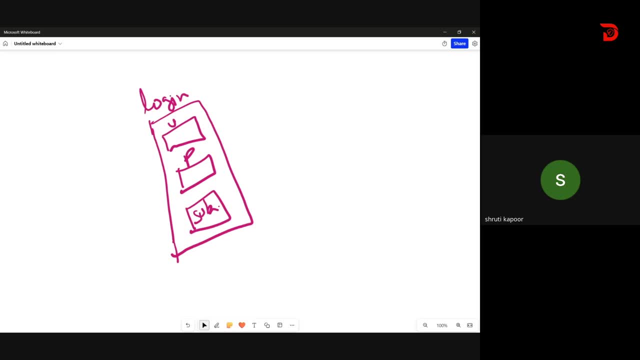 okay, so now. okay, so now you can do login when you have already signed up, right? so when you have created the account. so after creation of the account, you have the access to login to the site. so now you are trying to log in and and what's happening? so you are trying to log in and what's? 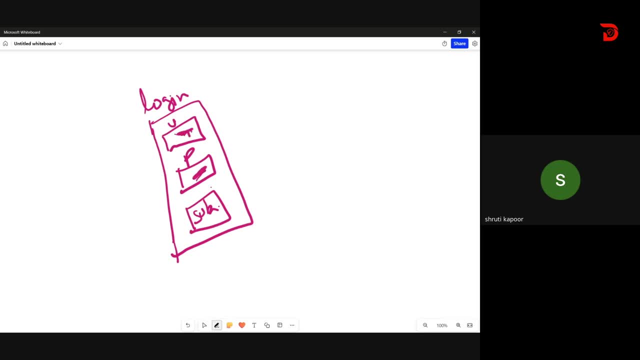 happening. so you have entered your id, username or password, okay, and you may press the submit button. so now your request mean your data package mean they are going to the server. they are going to the database server for the verification that whether the id and password which is being entered, 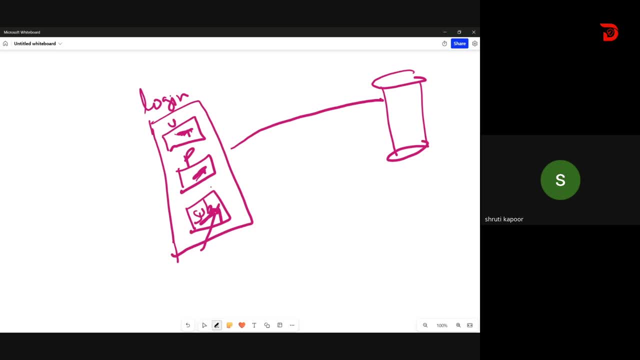 by you is correct or not? okay, so now database. so inside this database server, this database server, we have databases, okay. i mean, here we are having some tables, we are having the records, okay, and and there it's there, that serial number one. this is the username and the password for this person is: 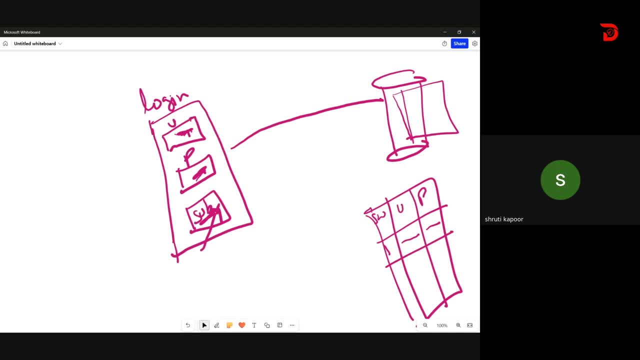 this password. so now, when you are entering the correct combination of id and password, so now this is being validated, okay, because, yeah, now it's being validated, and now the server is giving you the response, and now you can, and now you can uh see what like, uh, where the site will take you to, okay, so, so this is a role of database insider, uh, these. 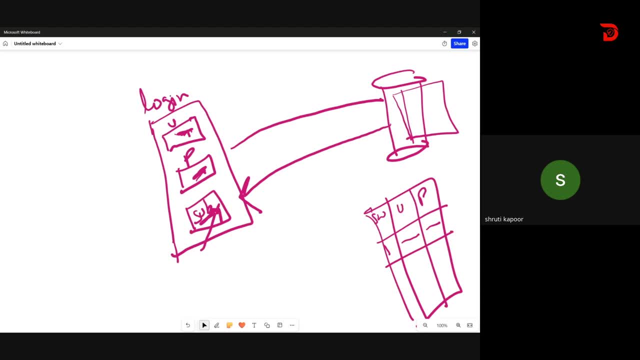 web apps. so now, okay, so now we have, we have tables of many types for the, for storing of the information, and and all these tables they are, so they are stored in the database. so now, sql is a language which is used to retrieve data from the data servers. okay, so, uh, yeah, so the role of sql. 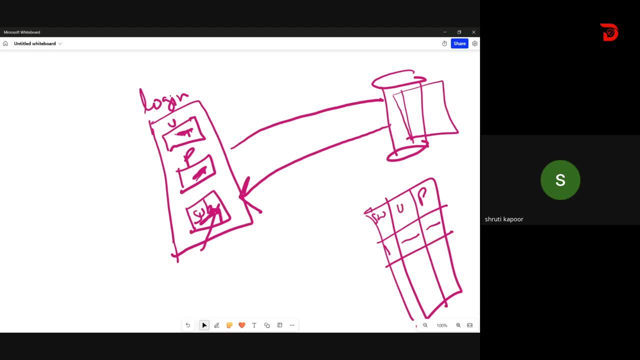 languages, to extract the data, uh, to extract the information from these servers and to insert the information into these servers. okay, so now in sql injection, what we are doing is: we are trying to, uh, so here we are entering something, malaysia, something, some malicious payloads, we are inserting. 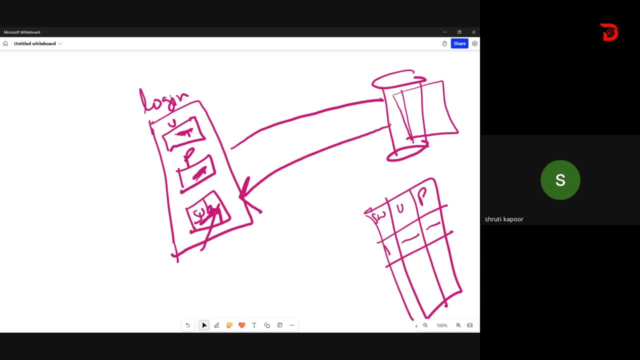 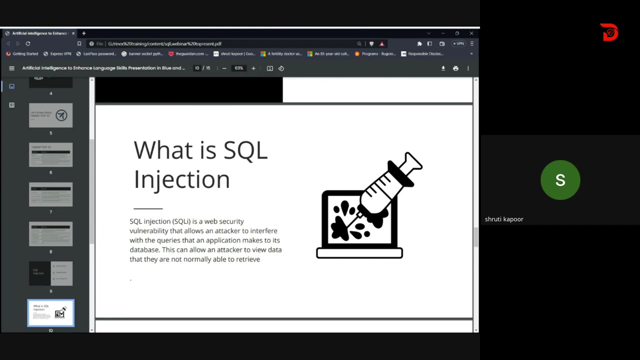 inside the input fields so that, uh, so that the sql query will get disturbed and and and the application will give us something sensitive which it is not normally given to us. so that thing is there in this sql injection vulnerability. okay, so now i'll all right. so now you can see here that sql injection is a web security vulnerability. 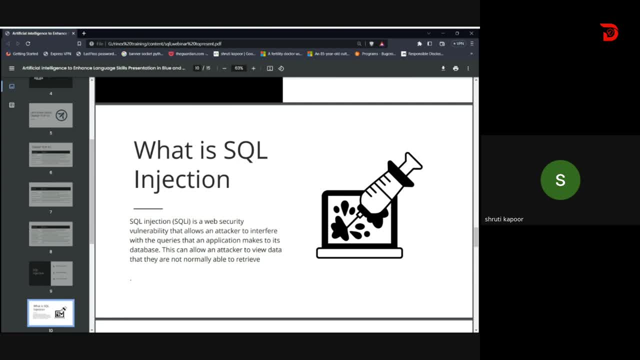 which is allowing an attacker to interfere with the queries that an application makes to the database. like i explained you that in the sql injection we are entering something uh malicious, because of which our sql queries, uh they, so they- have got changed and because of that thing the attacker is able to see that data. 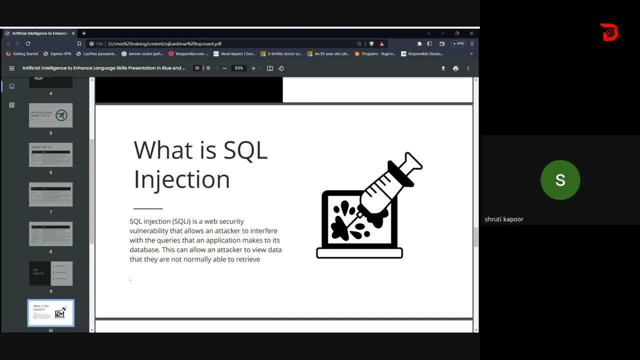 that data also, which he should not uh get that okay. so, for example, if you have entered something malicious and you are able to access id and password of each and every person which is uh which has done the sign up into the form, so such applause are there when we talk about sql injection vulnerability. so now we have basically three. 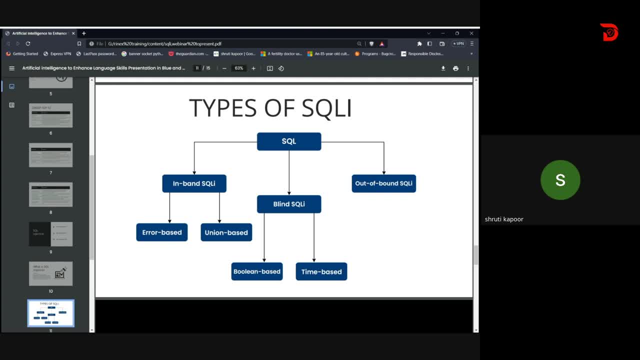 types of sql injections. first is inbound, then we have blind, and then we have out of bound sql injection. so now, what is in the sql injection? so now in england, sql injection during the payloads in the entry points, and then your web application is giving you results there only okay. so now that. 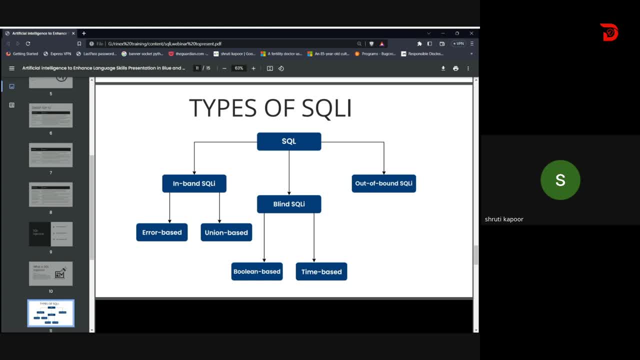 thing is inbound sql injection. so this inbound sql injection is basically of two types. one is error based, second is union based. so now what is happening in error based? so now, for example, you have entered something malicious, some malicious payloads, you have entered in the uh in the input fields, and now your your website. 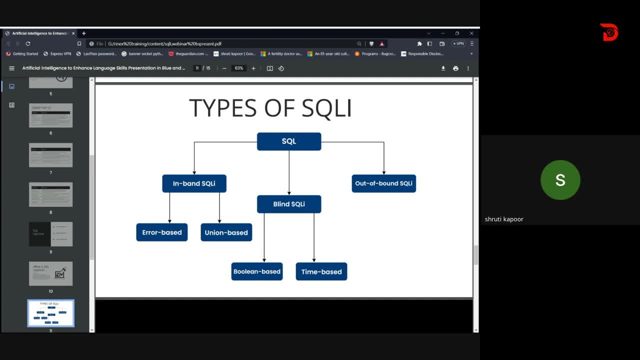 is giving you the error, okay, when it's giving some sql syntax error or some different error is giving you. so now this means that it's vulnerable to error based inbound sql injection and that's all what's happening. okay, and now the second type of sql injection, which comes under: 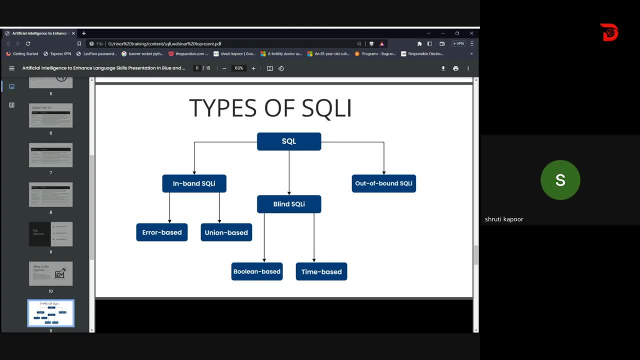 this in van category is union based, so now in union based sql injection. what's happening? so here we are helped by union operator. uh, like more, two or more sql sql queries. they are being combined when the result of multiple sql statements are being combined, and then, and then we are waiting. 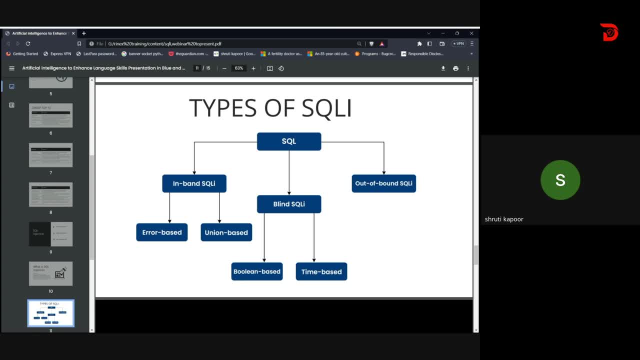 for the results. okay, based sql injection vulnerability, so they are also very broad in itself, uh, okay, so i'm only briefing you out about these vulnerabilities because they are very broad in themselves and we can't discuss, uh like, a lot about them in just an hour. okay, so now we have a blind sql injection, so in blind. 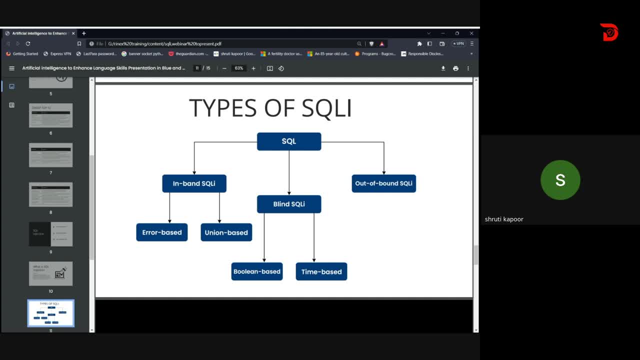 sql injection. what's happening here? so here, for example, i'm entering the payloads and neither i'm getting error nor i'm getting any result. so now i will, now i will craft my query in such a way that, uh, that i will ask my server, uh that, whether this thing is there or not, in order to understand. 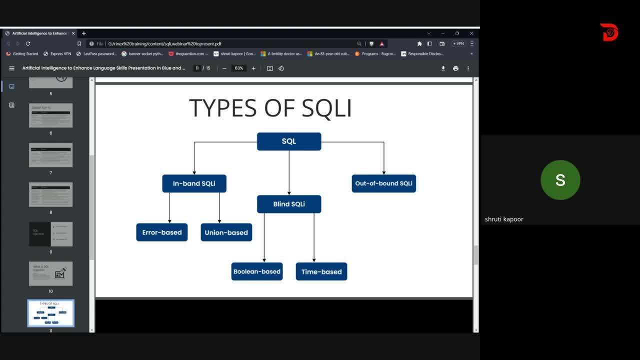 the database structure. okay, so here we are, we want to understand database structure, and for that thing we are, we are crafting our payloads accordingly. okay, so till here are the people getting. okay. so till here are the people getting okay. so till here are the people getting getting all right. okay, so now this blind sql injection is also of two types. the first one is: 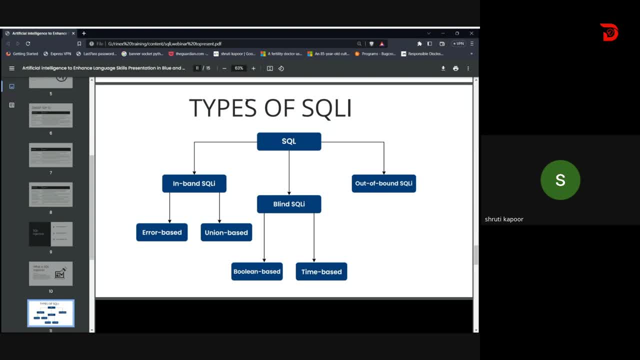 uh, the boolean base, and then we have time base. okay, so now, uh, so now what we are doing in boolean base? so we are using the boolean operators like or or and to know the database structure. okay, and now we have time-based sql injection vulnerability. so here what's happening? 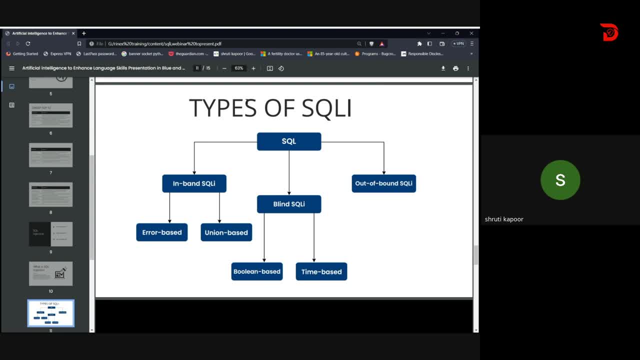 we are using, uh, we are using. so here we are asking, uh, okay, so i'll give you the example for this thing that we are so here, uh, for example, uh, we are asking the server that if the first character of the administrator's password is an, a, then wait. 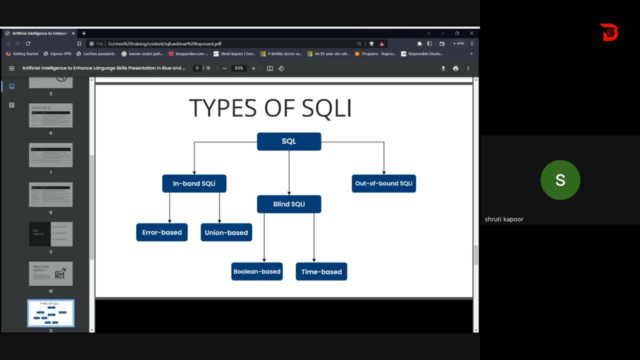 for five seconds or wait for six seconds, okay, so here. so here, like this we are. we are asking the server to understand the database structure, okay, and now we have out of band sql injection and now in outer band sql injection. what's happening? so here we. so here the attacker. 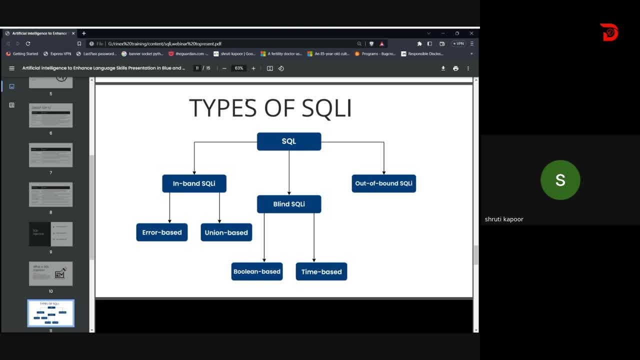 is not getting the result onto the same web app. neither he is able to guess by trying blind sql injection payloads. so for this thing he will redirect some of the responses to uh to some different server or to some different uh website, so that he'll be able to understand. 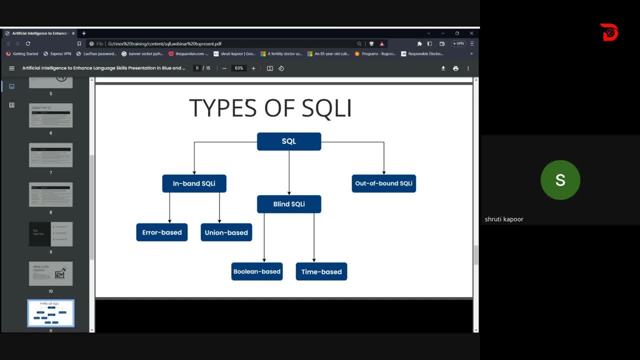 uh, the structure of the database. so, uh, okay. so now this out of bound sql injection is least commonly found, mean it's very hard to find this vulnerability, but it is, but it also has the same impact like these vulnerabilities. okay, all right, okay, uh. so now let's uh understand that. what is the impact of sql injection? 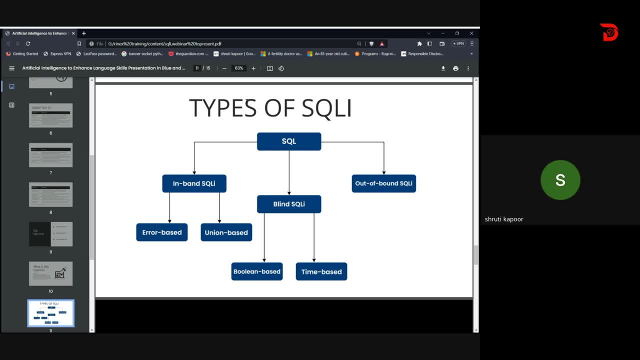 okay, so now this sql injection has impact on uh like on confidentiality to integrity to and on availability too. okay, all right, so may so be. a help of sql injection, sensitive data can be revealed. uh, we help of sql injection, data can be changed and we help of sql injection, we can delete. 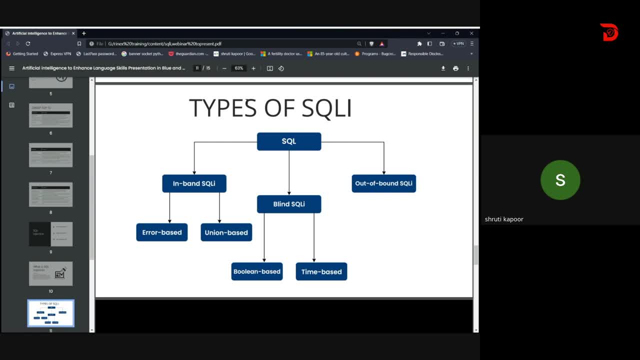 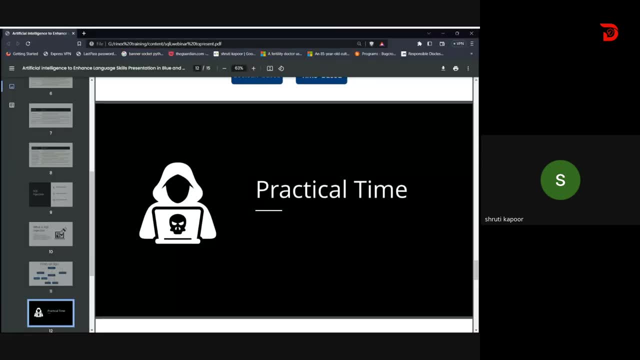 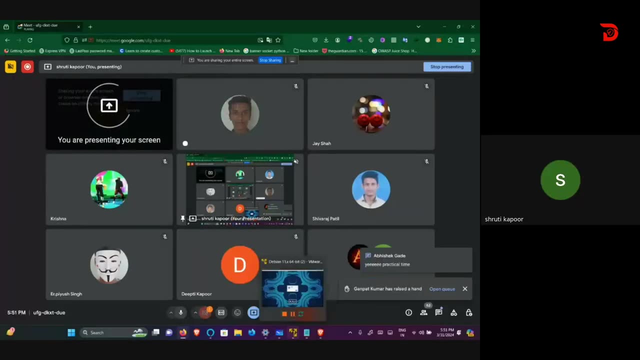 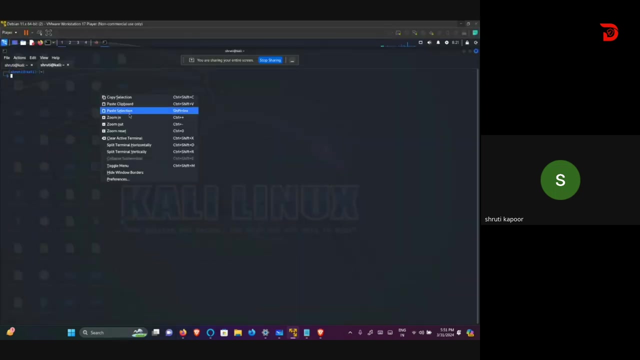 some of the records from the table. so that thing is also happened. then our website is vulnerable to sql injection. so till, here are you people with me, are you getting? so? now let's do a practical and sql injection. uh, okay, so now i am sharing my sally. okay, so can you see my screen? um, i guess it's visible. okay, all right, okay, uh, so for this, 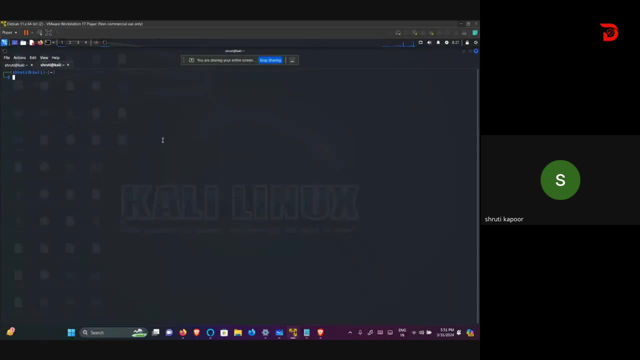 practical. uh, okay, so see, there are two ways to find sql injection. this is the manual way, where where we are. so here, so in the manual, what we are doing we are. so the first thing is we are searching for all the input fields, whatsoever are there, and then we will insert the malicious payloads. 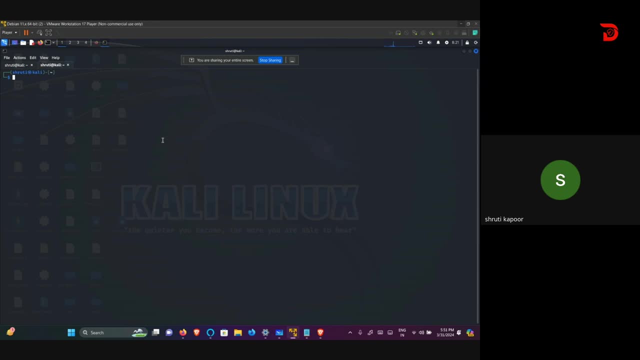 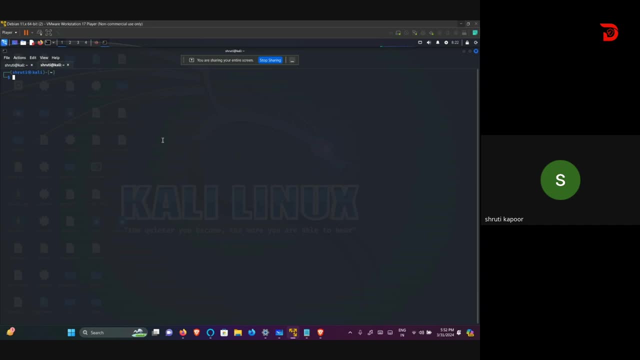 okay, so this is how we have to go on. okay, but for today's session, i'll show you a tool which is sql map. so sql map is a tool where help of which we can automatically detect and exploit the sql vulnerabilities. okay, so it's a very simple to use tool. uh, and it's very 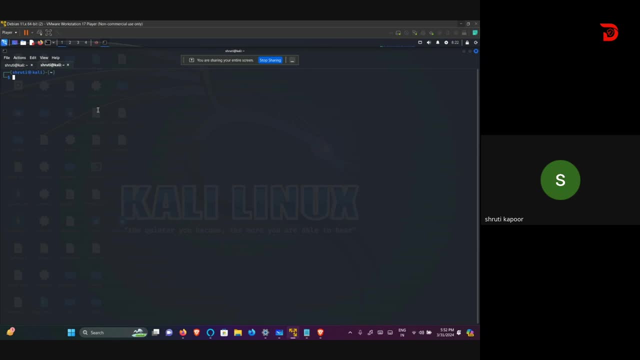 yeah, and it's a very good tool, so we help. so this sql map is giving you a lot of features. okay, so now, first we'll see. uh, okay, so now, whenever you want to know features of any tool, you need to type sql map and then dash dash help. okay, so whenever you type sql map, dash dash help. 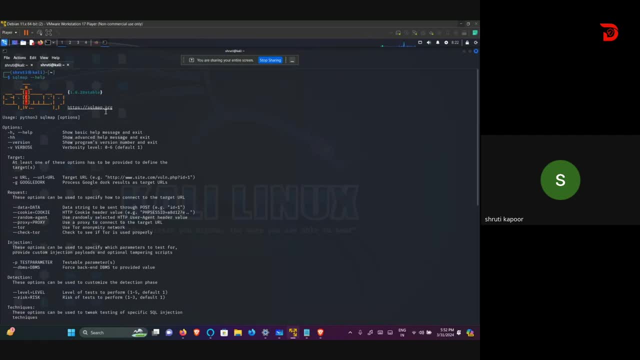 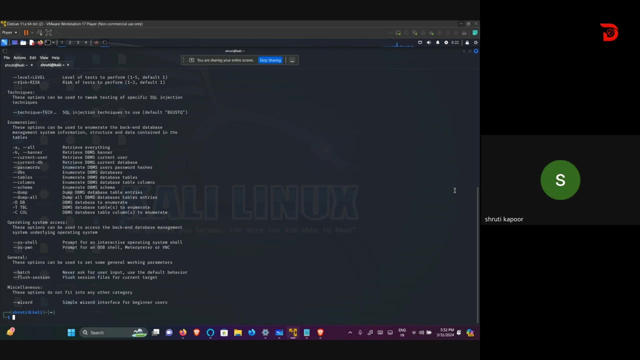 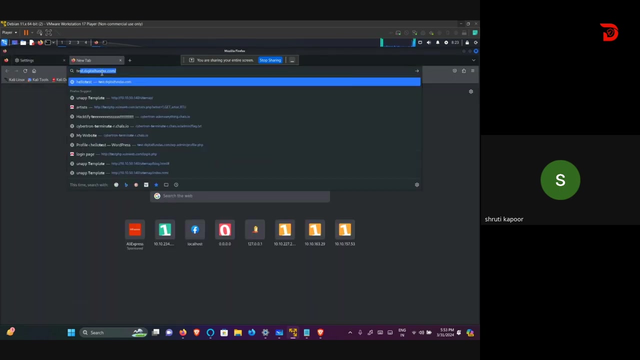 now you will be able to, to understand that what all functions this tool can do. okay, all right, okay, so to keep a practical session simple, we we will be testing on a web app that is a vulnerable web app, which is which is testphp.1 web. okay, so now i'll show you. okay, so we will be testing on this app. 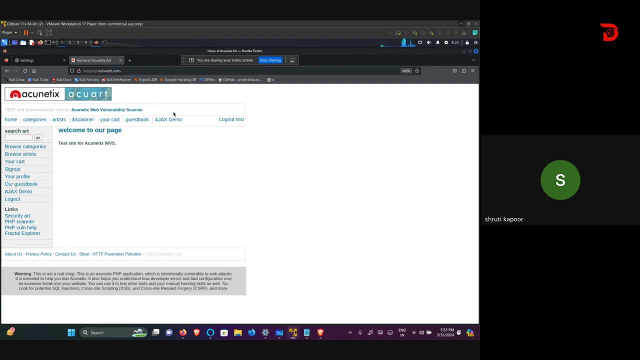 guess you can see. so, okay, so now we will do testing on this side and then we will see whether it's vulnerable to SQL injection or not. okay, all right. so how we have to proceed. so the first thing which you need to do is: so first we will. 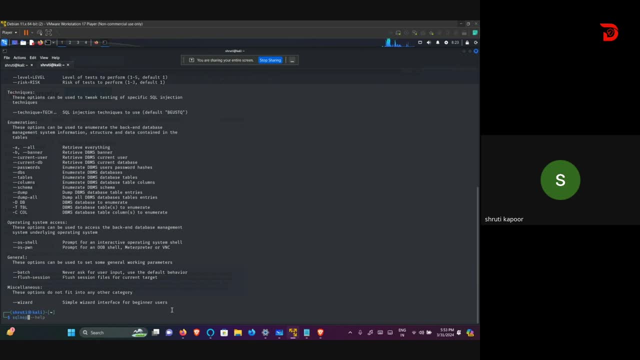 okay. so the first thing which you have to do is you have to type SQL map and then you have to type dash you. okay so. so how you have to write the query SQL map, space dash U. dash is for URL. okay, like what's ever URL you want to test? 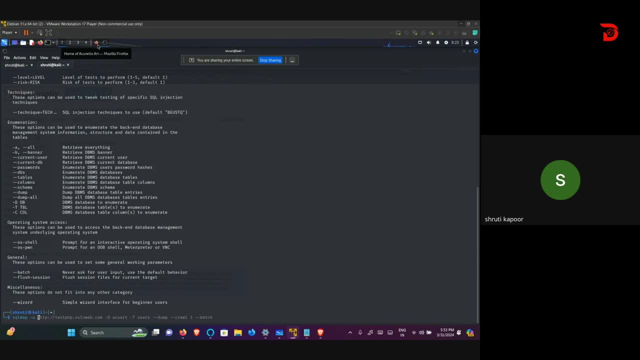 for. so okay, so now here we are. we are testing a URL whether it's vulnerable to SQL injection or not. you can also capture a request in Bob suit and then you can. you can check for SQL injection in that request also. okay, all right, so now we'll see. okay, so this was the side. so 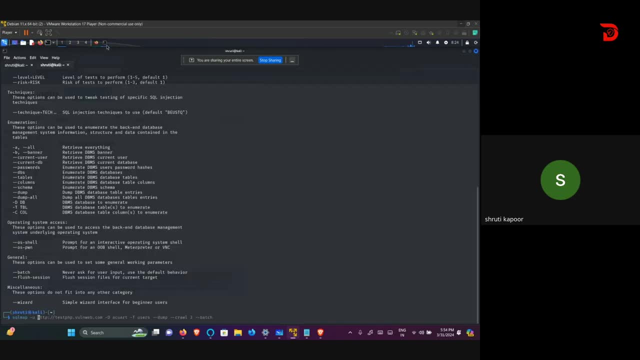 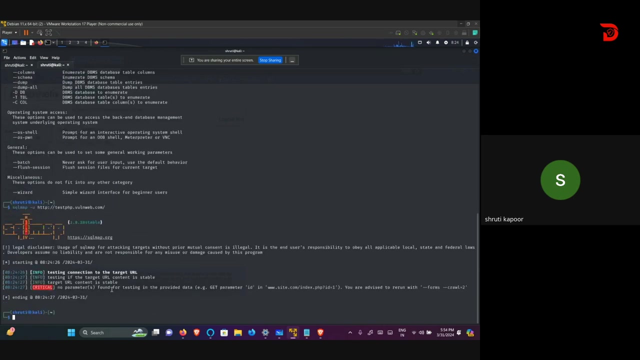 this is my URL. I am simply copying the URL and now here you can see I have pasted the URL. okay, so I pasted the URL now. okay, so now I press enter now. now you see that that I have not got enough information right, because to find the 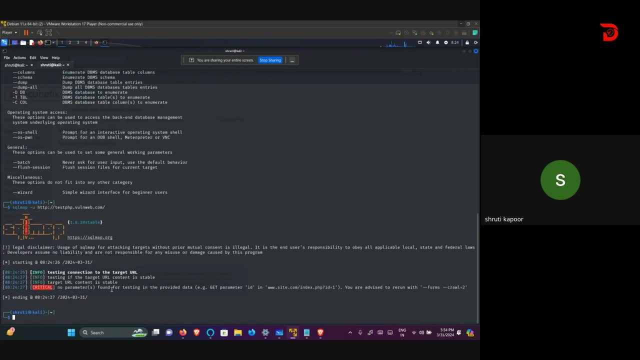 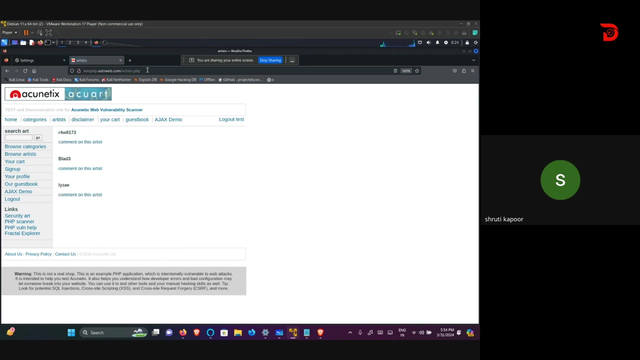 enough information. we need to. we need to either increase the crawl level or risk level. okay, so now what is crawling? so we? okay, so you know what all our directories. so directories are the endpoints. for example, if I take, take you to any website. for example, if it's a website and I am clicking on artist can. 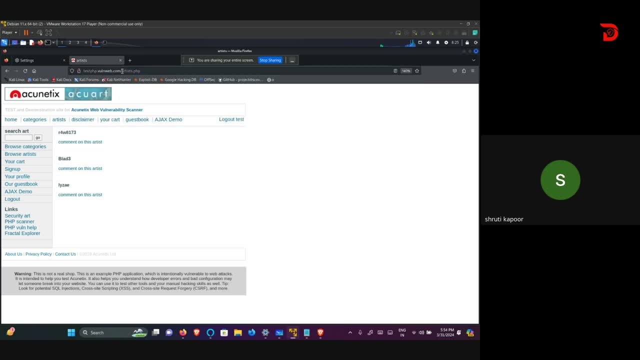 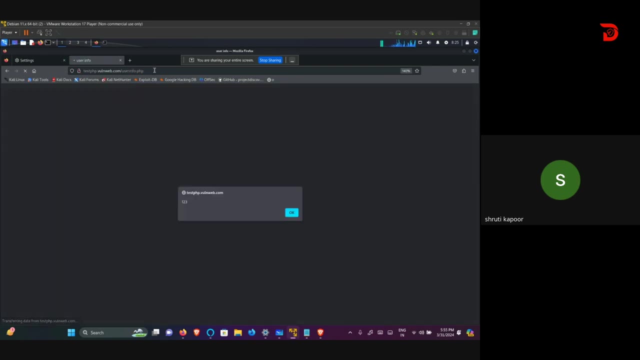 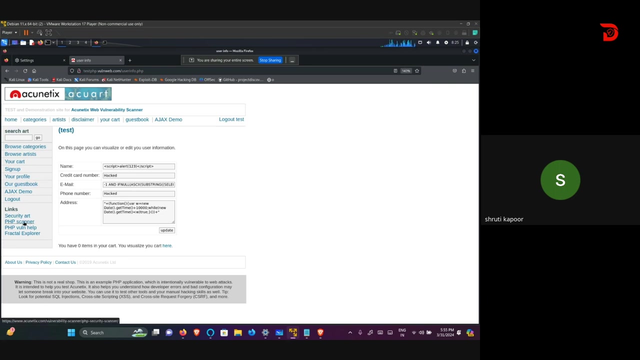 you see artistphp, so it is a, it is a directory. if I go to give guest book, it is a directory, okay. and if I go to this, okay, in this or guest book, your profile, so your user info, so all the sites, so they are, they are the directories okay. so here you can see PHP scanner, so can. 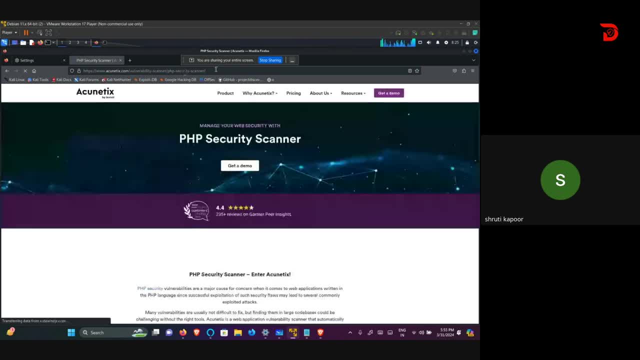 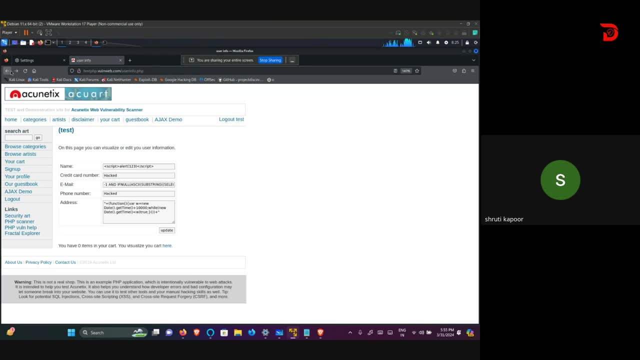 you see this thing: vulnerability scanner, PHP security scanner. so it is our directory. so all these things are. so all these things which you will see after flashes, they are the directories. so now when I am crawling, so by crawling I am increasing the number directory level that in this directory I need to go. so, for example, if this is our directory, 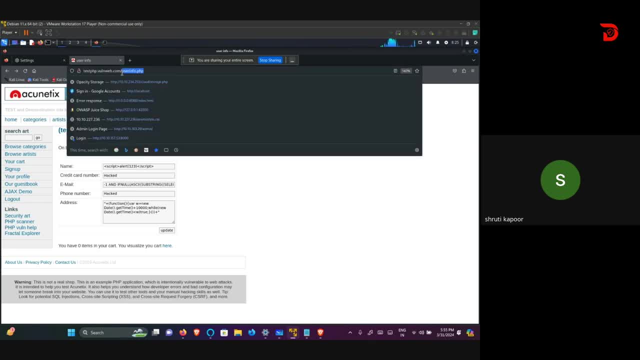 level. so it is crawl level 1 because it's only the first directory. okay, for example, if I want to go into more detail, I want to go in a more deeper way. I will type mean, for example, if there are some more directors over here, now for this. 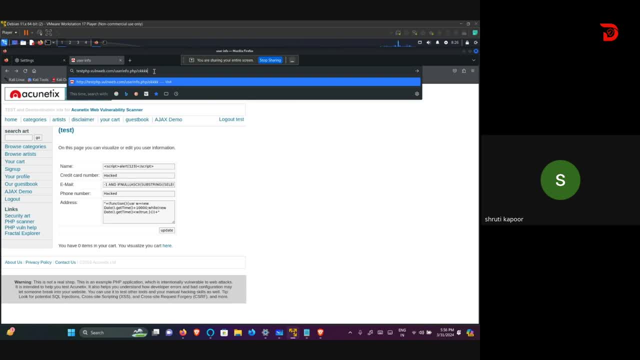 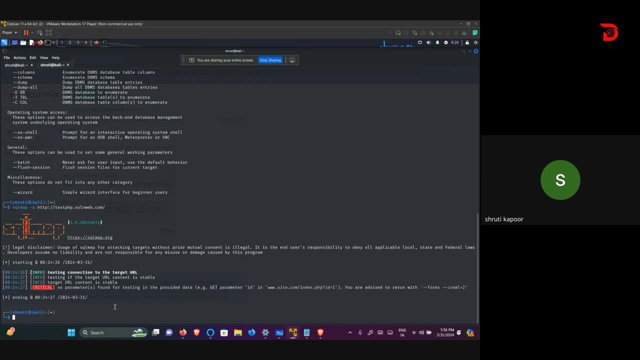 thing, I will make my crawl level 2 okay. and now, if there is something else also inside this directory, now for this thing we need to make the level 3 okay. so now a crawl 1 okay. so so by default, crawl has the value 1 by default. 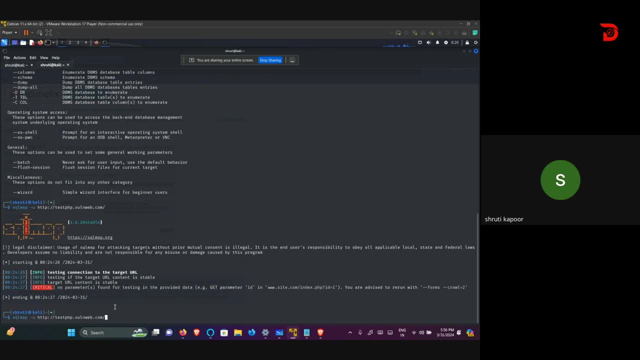 but but for this testing thing, I am showing you the level mean, the crawl value: 3, okay, so now, if you will see I am typing 3, okay, so when I will type 3, now my SQL map is doing the more detailed scanning. okay, this is scanning. each and every web page, whatsoever is whatever it's. 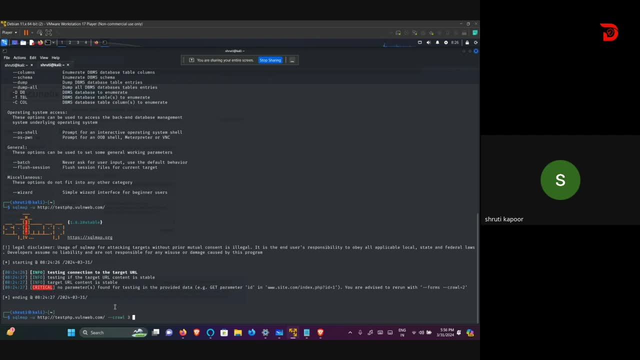 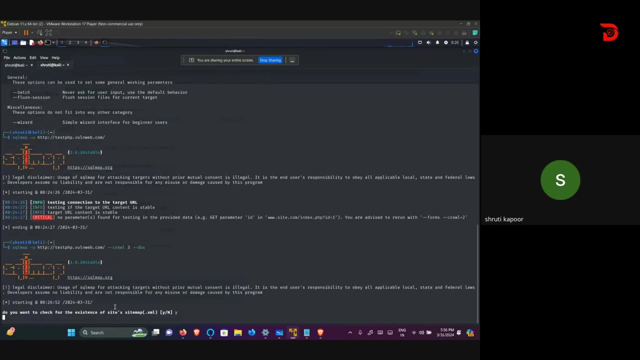 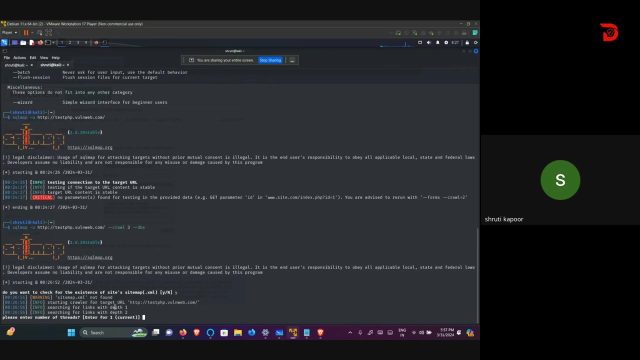 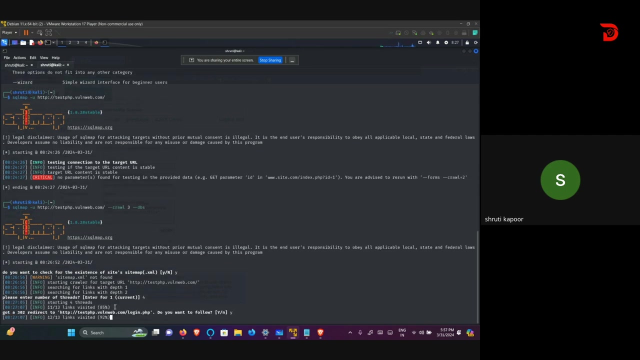 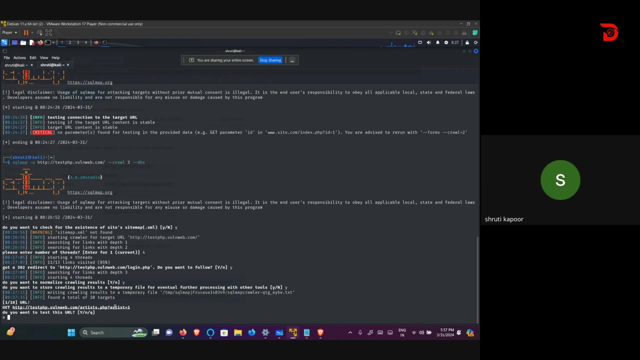 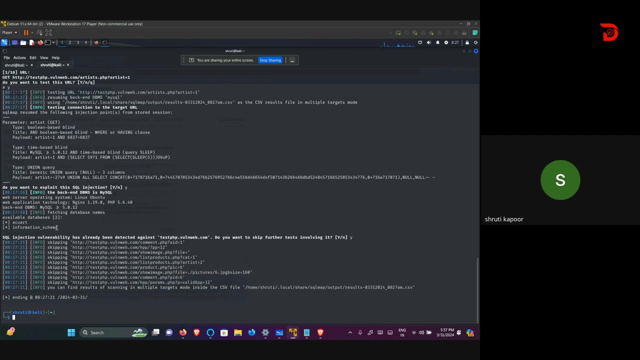 founding in each directory. okay, and now and now, if I will do DBS, okay and I'll type by. so now it's asking me the number of threads, so this is. so this will increase the speed, okay, and I am choosing 4. okay, so here can you see that I have got two databases, one a co-op, another. 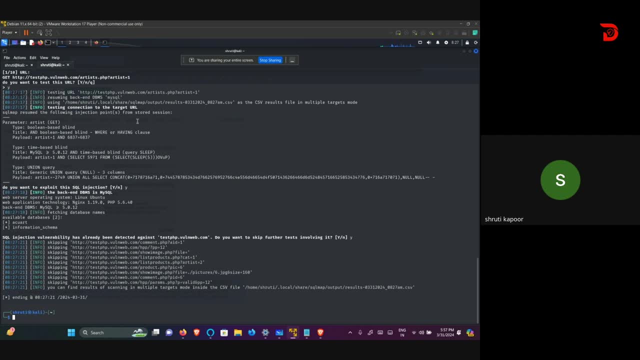 information schema. okay, so can you see that by using option dash dash DBS I can extract the information about the database? okay, so, by using a skill map, dash you and simply the URL, and then I did crawl, mean crawl, and I said the value of crawlers 3 and then I gave the option dash dash DBS. so by typing dash, 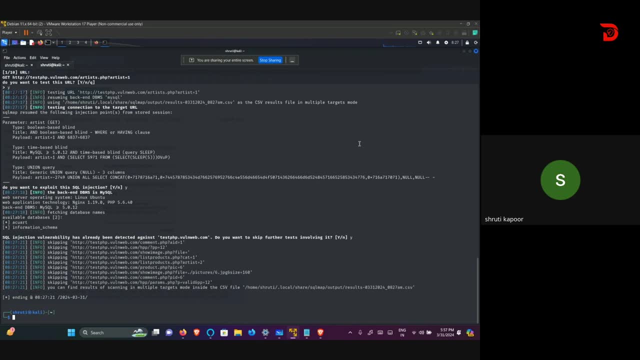 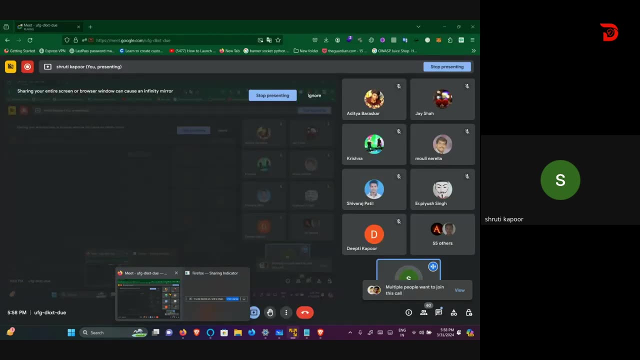 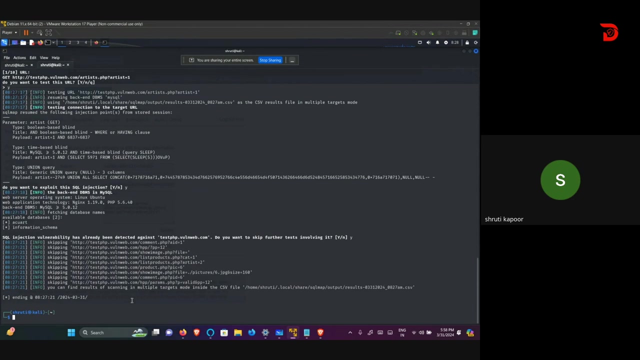 dash DBS. I can know the database structure, that what all tables are. then side the database. so till here, are the people getting that how we found out the database name. okay, alright, okay, alright, okay, so now we will. okay, so now I have. so now what is? 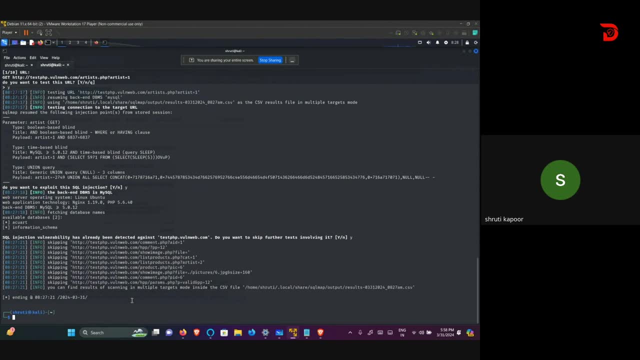 our database. our database is a collection of a lot of tables. okay, like you might have read in your childhood: what's the website? a website is a collection of web pages, right? and similarly, our database is a collection of a lot of tables. so now we want to know what all tables are there? okay, so 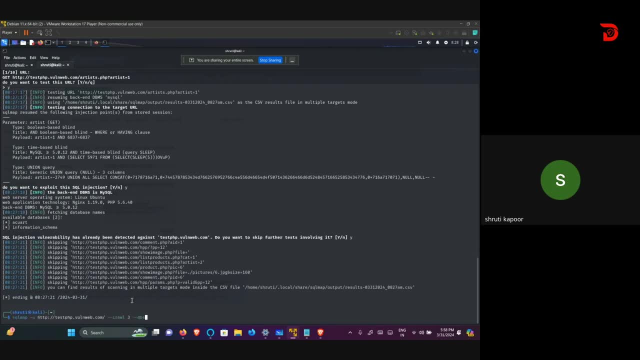 so now, how we'll find it? so first, okay. so now, since i know the, since i know the database name, so the database name is aquat, okay. now i want to know the tables which are there inside this database, okay, and now i don't want to see this. 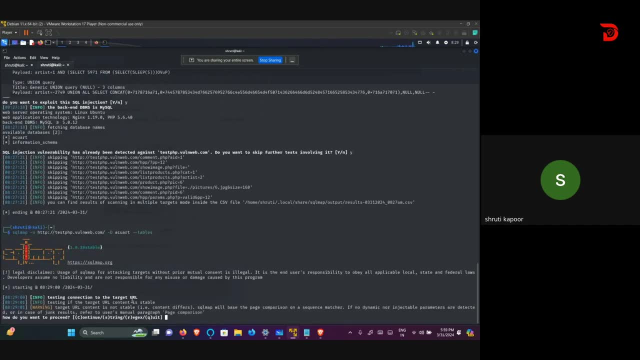 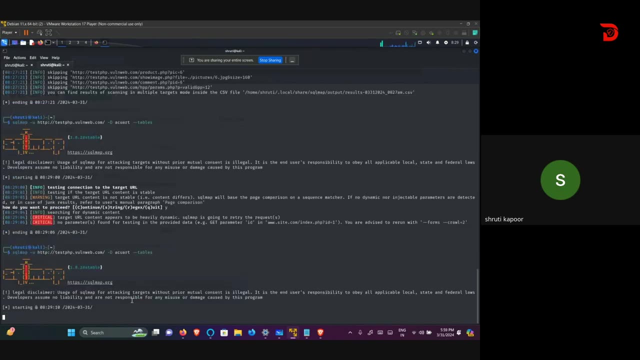 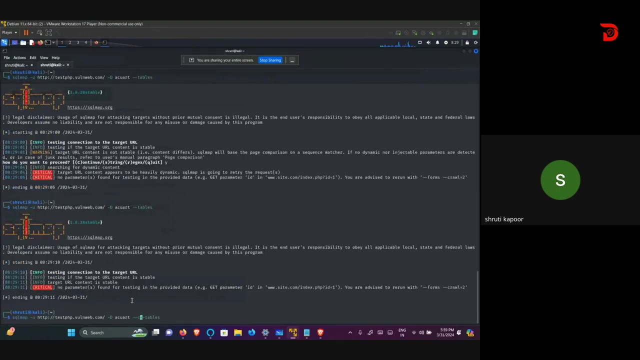 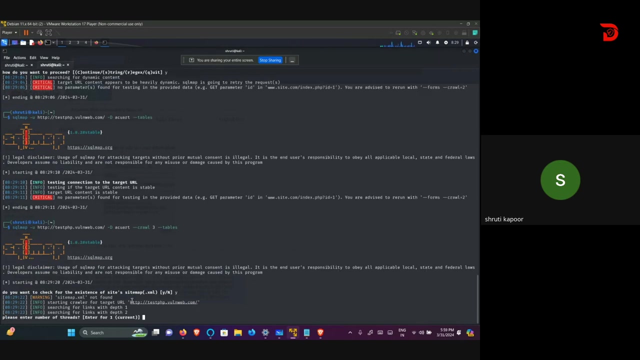 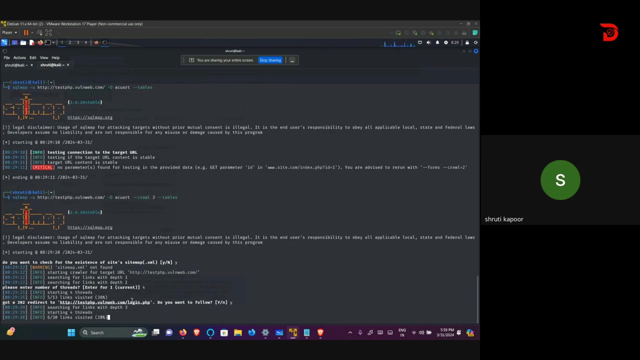 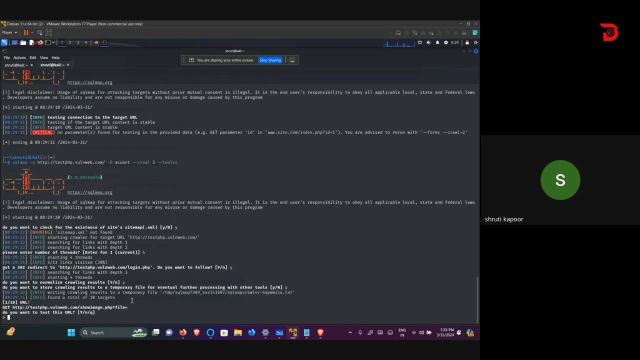 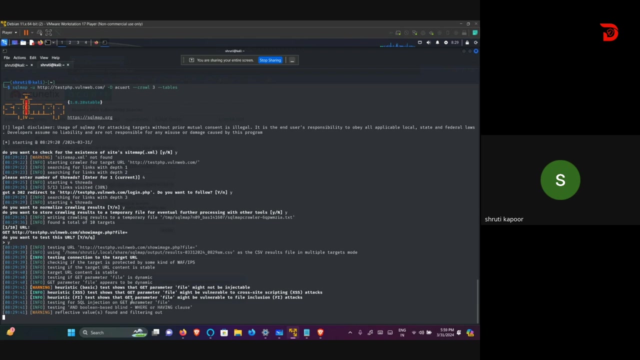 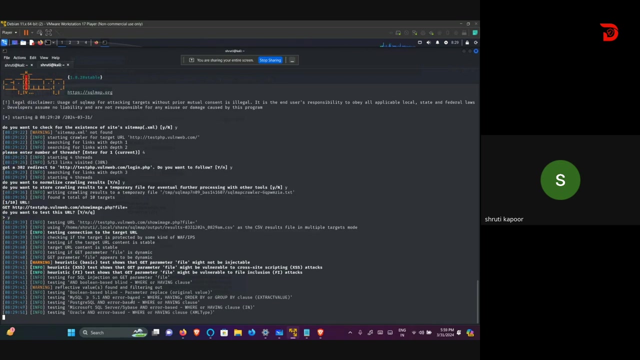 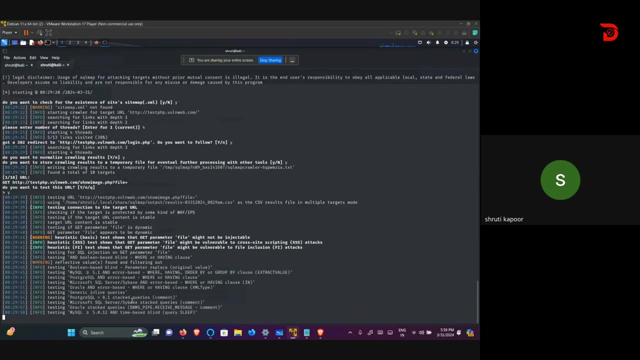 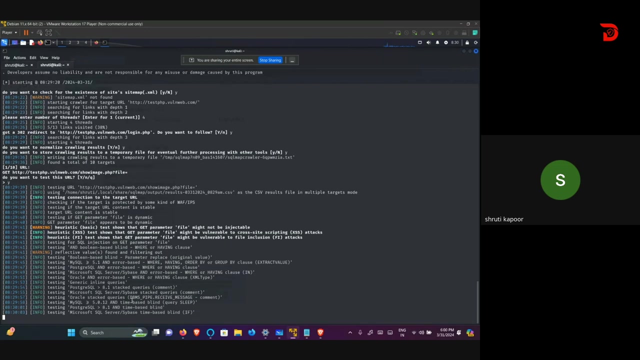 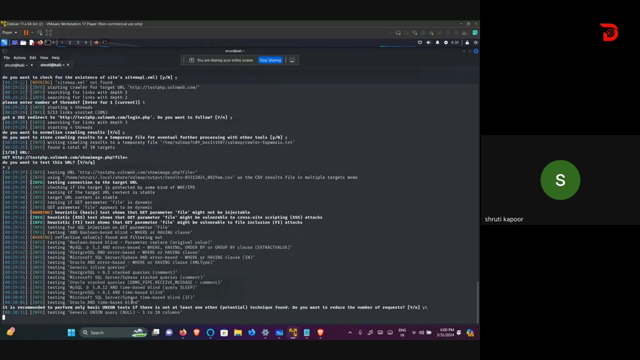 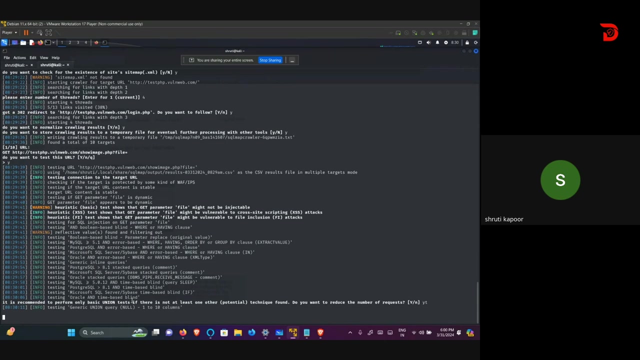 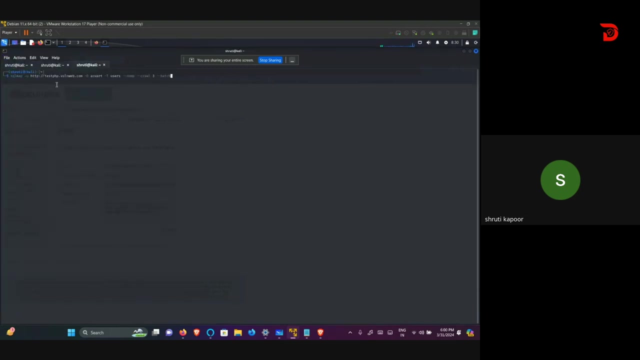 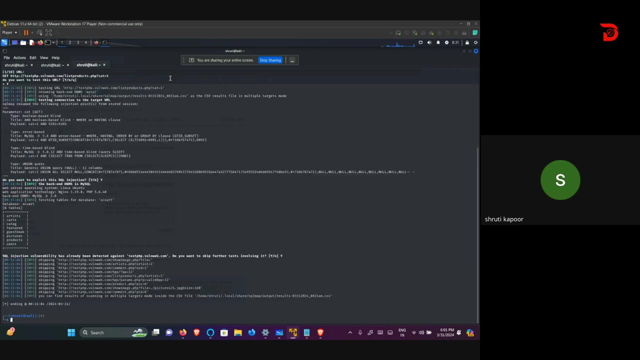 thing. so i'll do enter. okay, so we need to increase the crawl l2 you. This is taking a lot of time. I'll show you in this tab. Okay, so see, can you see I have used the option dash dash batch. So by using dash dash batch I have like. so I don't need to press enter or y every time. 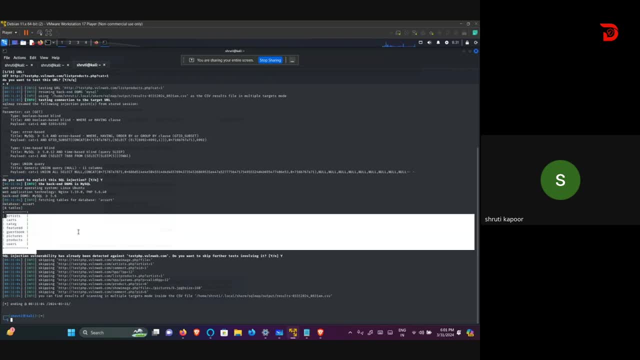 So here I guess you can see that I have got all the tables- whatsoever are there inside this database acquired. Okay, so now these all tables are there inside the database. So now, for example, I want to, I want to know information about a table which is users. 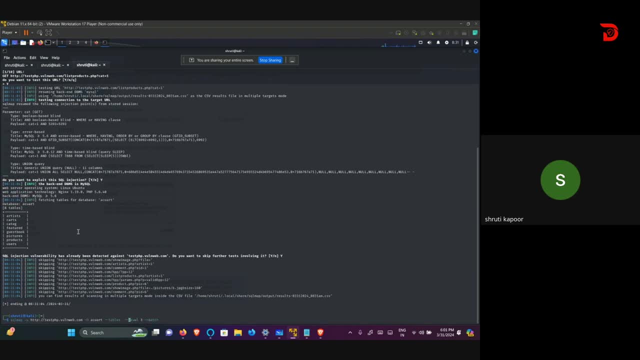 So how can I do that? So for that thing, I can simply write dash T, So dash capital T is to to go inside the table, is to know the data about the table. And now I'm typing users And now I'll do dash, dash dump. 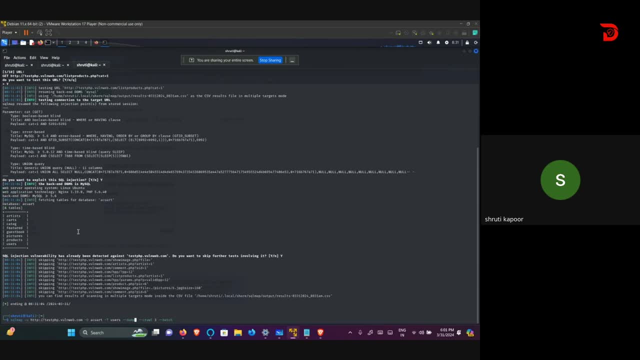 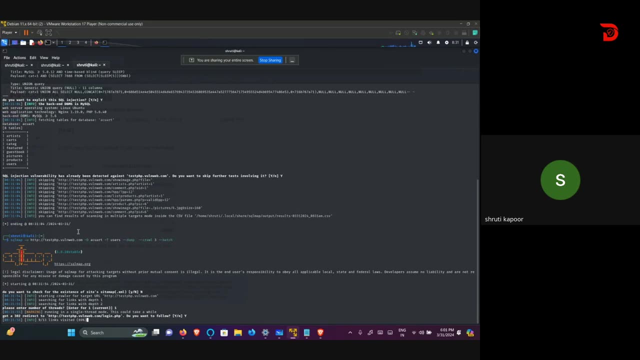 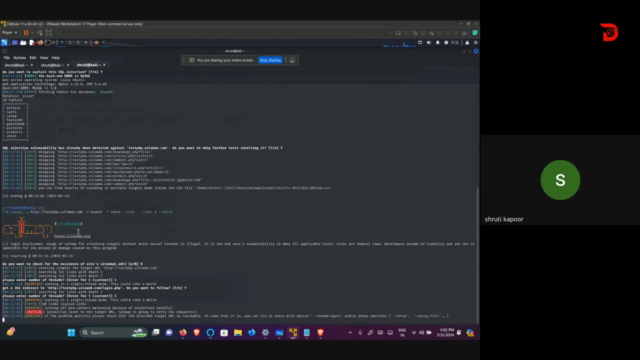 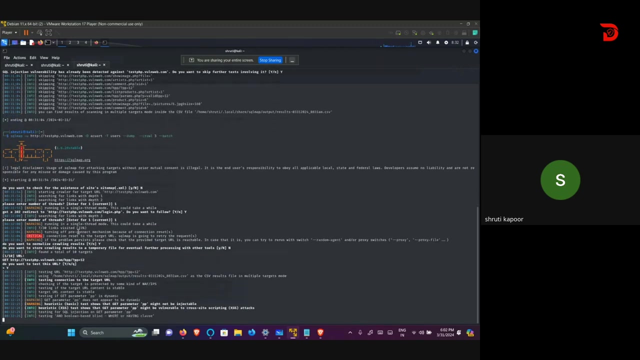 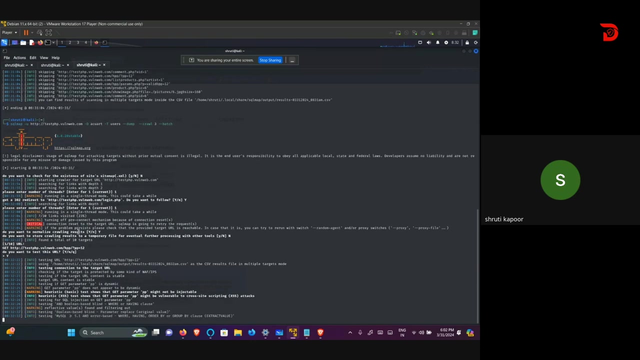 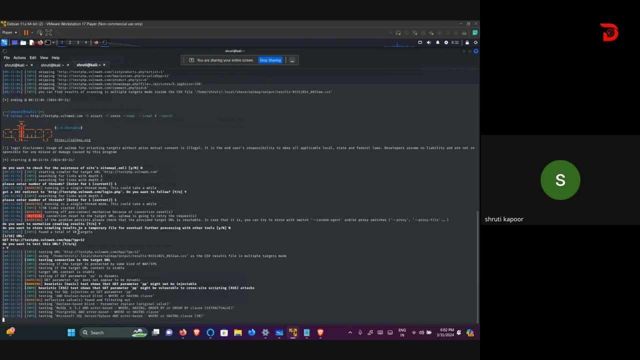 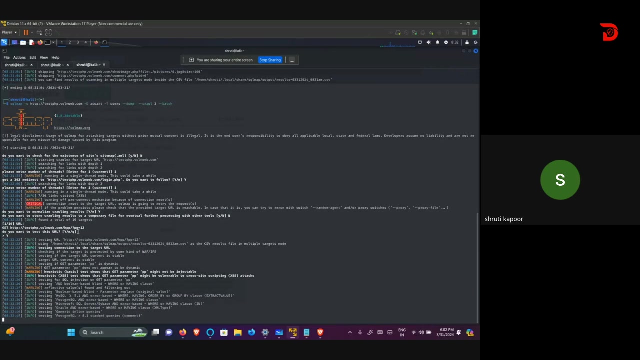 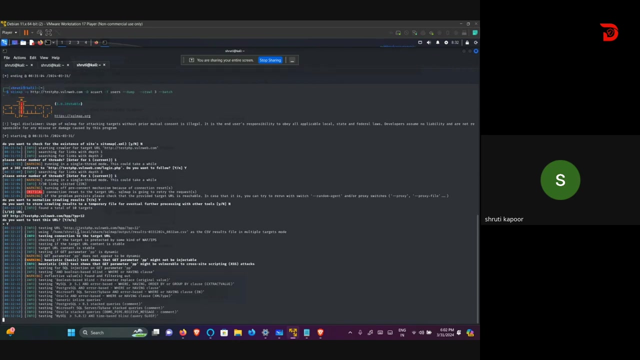 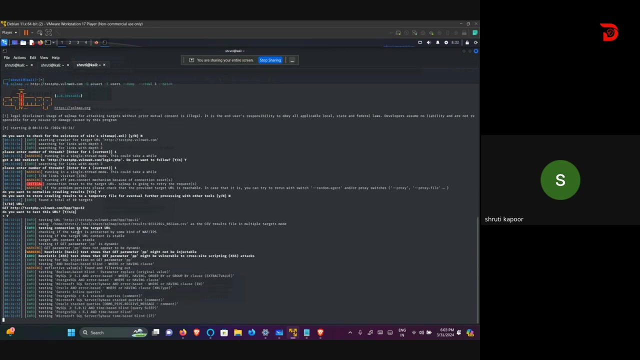 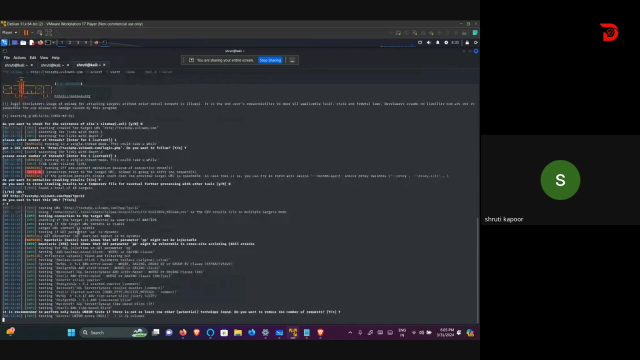 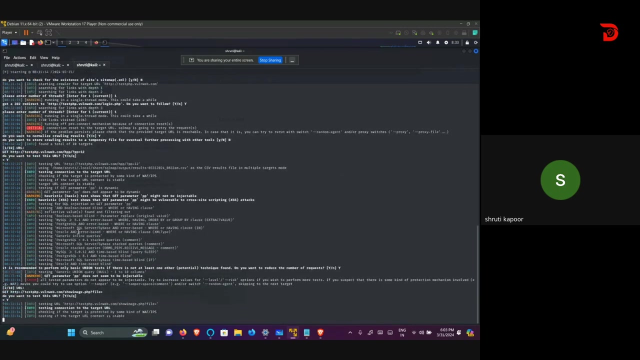 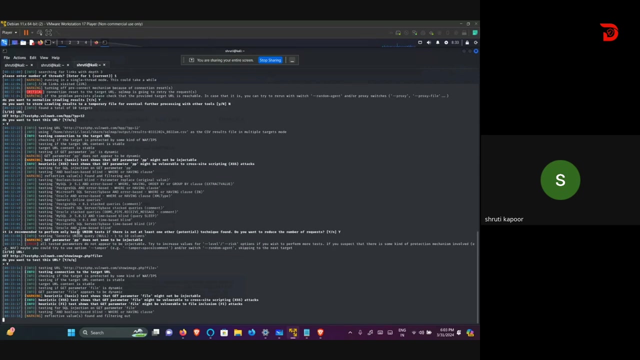 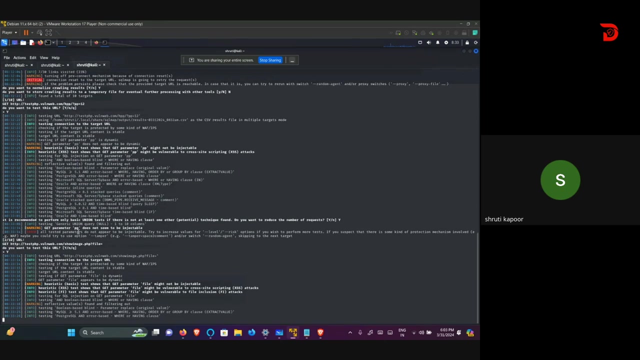 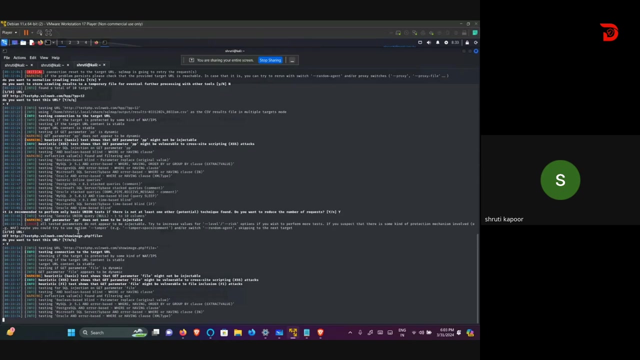 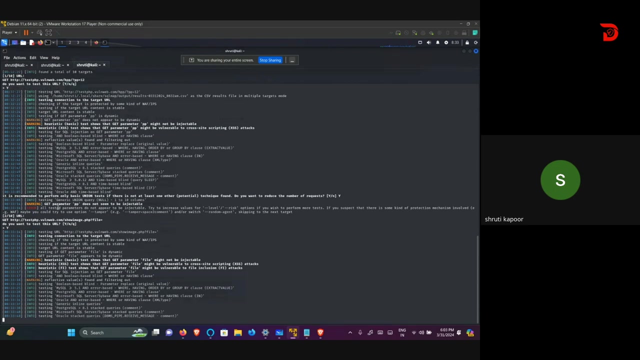 So dash dash dump, Okay, so now I have to do slash lower case value And now dash dash dash on, Okay, so I know what that look like, right? Okay, so now, if I click, enter you. Thank you, Thank you. 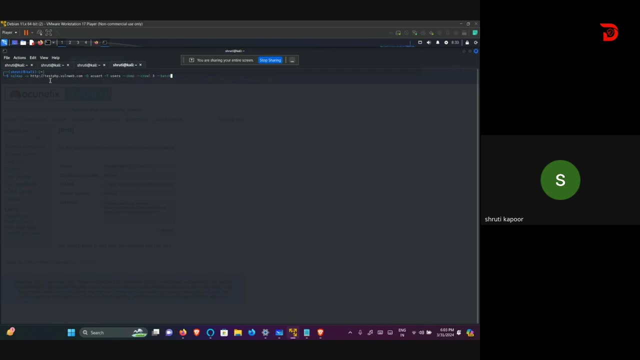 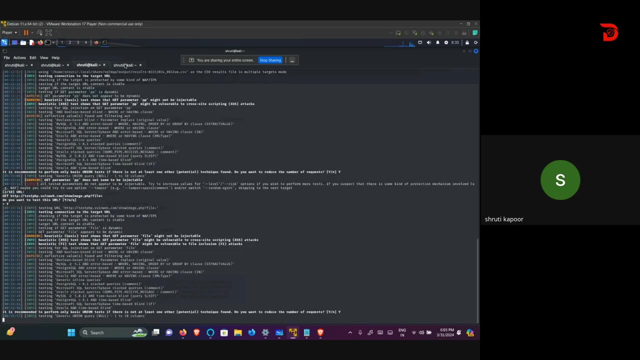 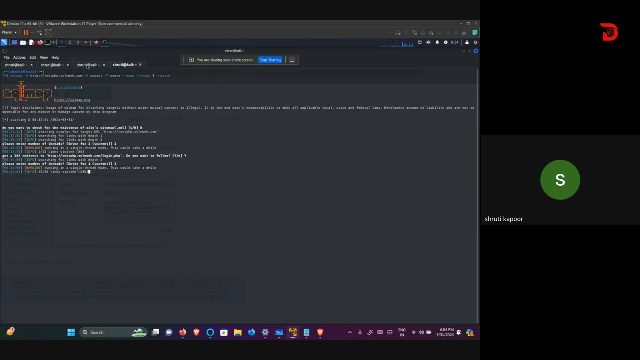 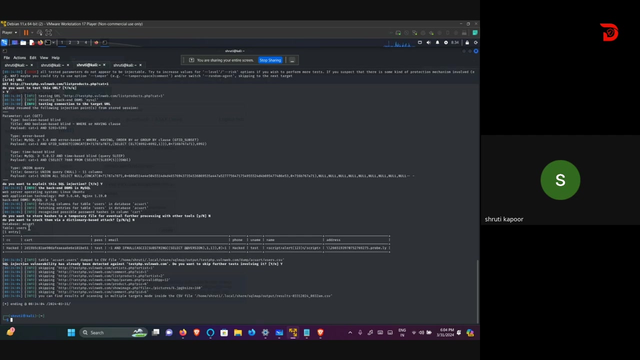 Okay, Okay. so here can you see that we have extracted the information which was there inside the table users under this database at one. So here we can see that the password is test. the phone is hacked means the phone number. somebody has changed the number. 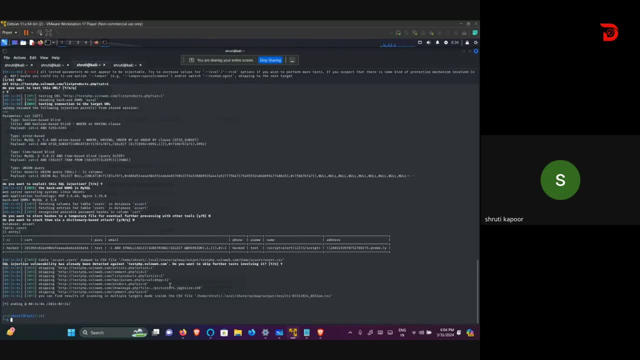 and then the username is test and here we can. so this is how we can extract the information whatsoever is there inside the table. So now, for example, I want to extract all the tables which are there. So for that thing, I have a simple command. 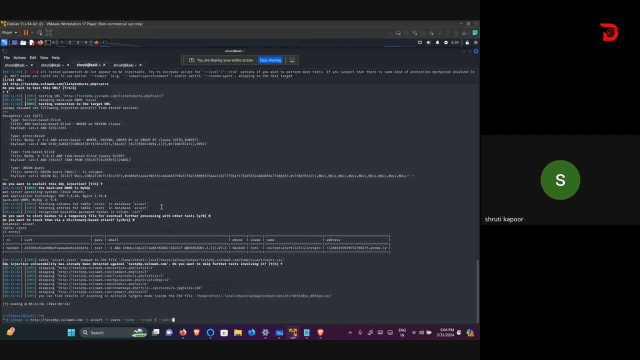 which is dump all. So by typing dump all, I can extract all the information which is there inside each and every table. Okay, but okay. So, for example, now I want to know information of any random table, So by same thing we can do that. 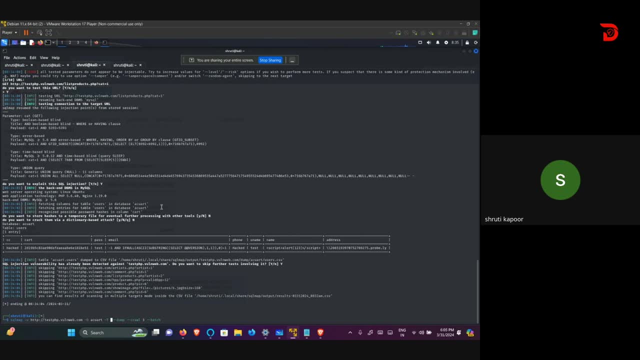 Okay, so this is how we can use SQL injection, We can use SQL map in this way. So here we did automated scanning, So SQL map automatically detected and exploited the vulnerability. Okay, because when we search for the, when we search manually, then it may also happen that 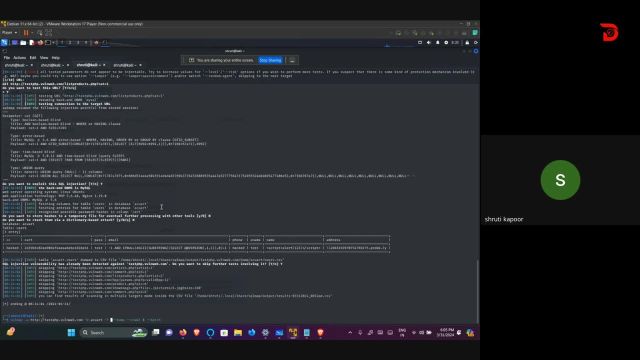 it will take a lot of time Because for that thing we have to. we have to check for a lot of payloads, be it for error based SQL injection and be it for the Boolean based. So this is how we should proceed. I hope you people have understood. 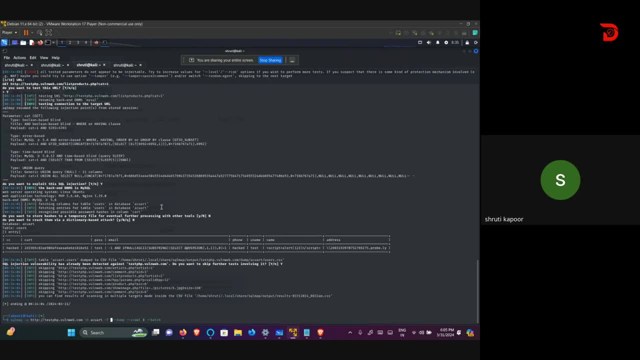 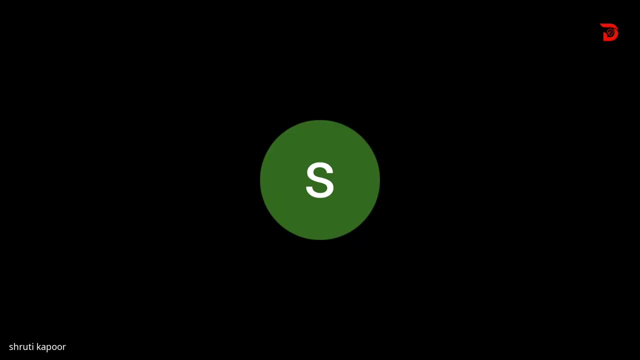 that how we can use a skill map to extract the information which is present inside the table in the databases. Okay, so anybody having any confusion or doubts please ask me. Okay, so can you see my whiteboard? Yeah, it's visible. 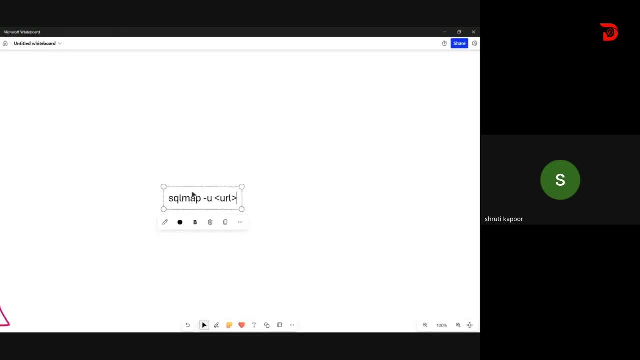 Okay, I have to type the URL and after that thing you have to set the. you have to set the value for the crawl. Okay, so we hear value. Okay, and after that thing you have to type DBS, and DBS is used to know the name of the database. 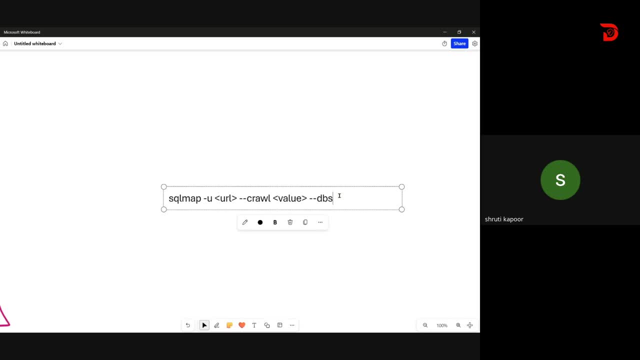 Okay, so this is how you have to use this SQL map And, for example, if you want to extract the, if you want to extract that, what? all tables are there inside the database. So that thing you can do by typing SQL map: dash U and then URL. 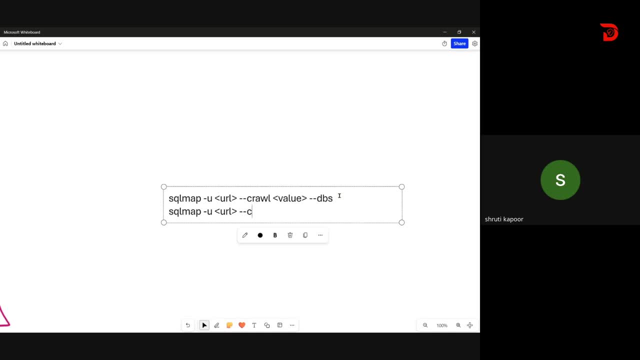 Okay, and then you can simply roll the value. Okay, crawling is important, Okay, and then you can. you can write dash D and then the name of database, name of database, and then you can do dash dash tables. Okay, By typing this query, you will be able to know the information. 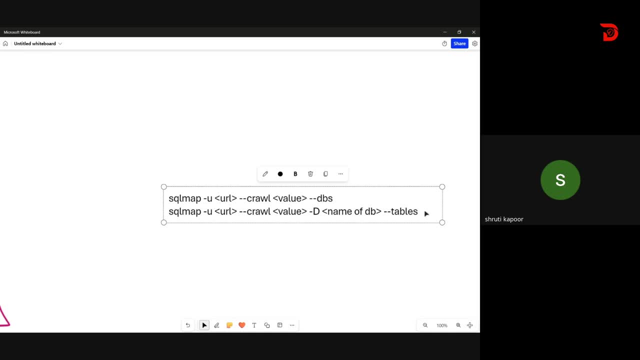 like what all tables are there inside this database? Okay, And now, for example, you want to penetrate inside the table, mean you want to extract what server data is there inside the tables. Now, for that thing, what you'll do. So these steps are common. 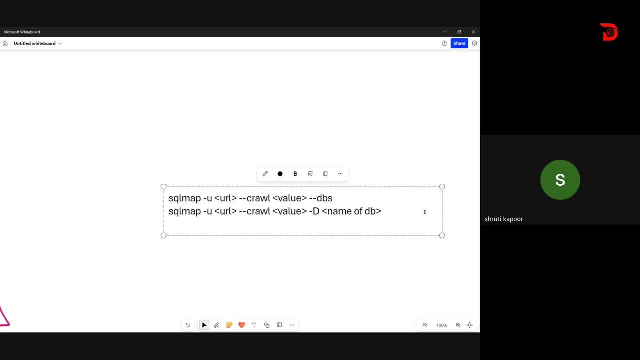 Okay, now for that thing you have to do dash D- the name of database, and then dash D- name of table. Okay, and then you have to type dash dash dump. So when you will type dash dash dump, then you will be able to extract all the information. 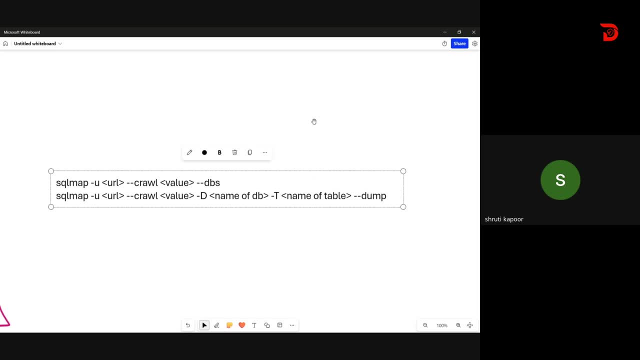 which is there inside this table. Okay, so have you understood now? Is it clear to you now syntax? Yes, So the next step is to explore the directories. Okay, All right, Okay, Okay, so this is the use of batches. 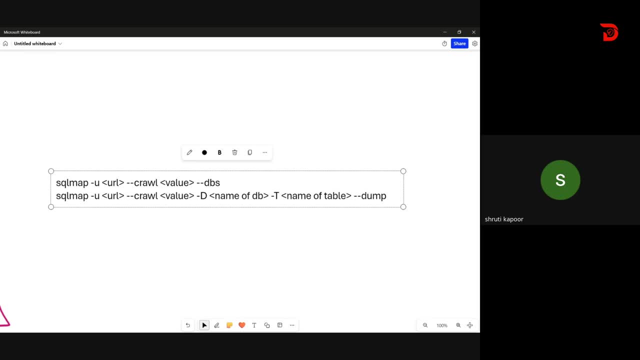 Let's see: earlier I had to manually type y and then enter, enter for each and every step. But now, after typing batch, now, now the SQL map is automatically choosing the default. like the default, things mean yes, yes, yes, and then enter, enter. 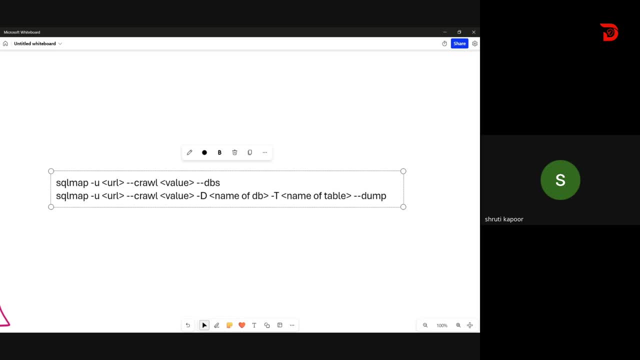 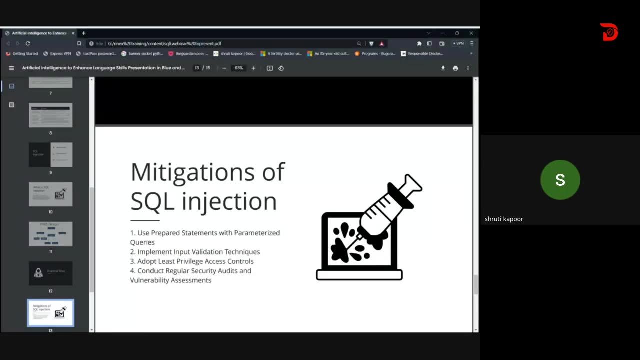 which I was doing manually. So, yeah, so it is reducing my efforts, Okay, Okay. so now we have done the practical. So now we have some mitigations to prevent SQL injection, Like we should use prepared statements with parametrized queries in place of normal SQL statements. 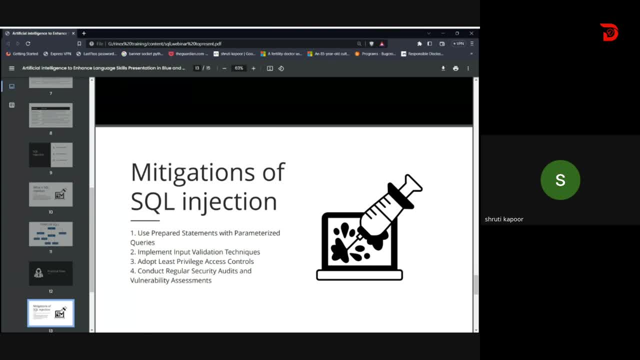 Okay, So, okay. so, in order to understand SQL injection properly, you should have at least basic idea of how SQL is working. okay, html is working and what are prepared statements. okay, uh, okay, so, okay. so now the next point is: uh, like we should use the input validation techniques. so now, what do you mean by input? 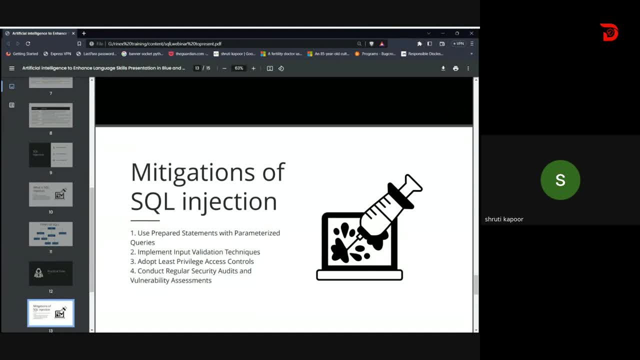 validation techniques mean whatsoever. inputs are being entered by the attacker in the entry points. now these inputs should be, uh, should be validated that, whether they're malicious or not. okay, so, but that thing, the developer, uh, whenever he's creating the application, he can, so, he can uh. so, yeah, so he. 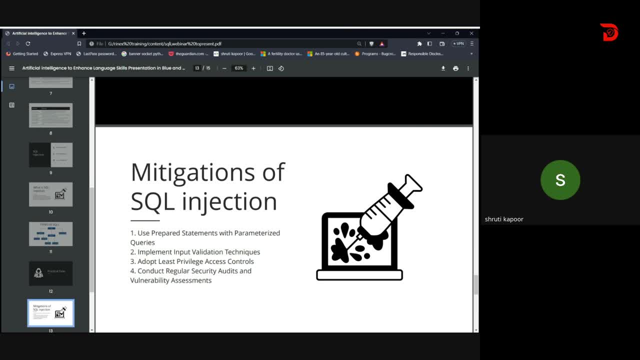 can validate, so he can add this feature to validate the uh input, whatsoever person is entering, or the or. the other thing is that a web application firewall can also be used to block such malicious payloads uh from getting executed. okay, now the next thing is adopt the least privilege access. 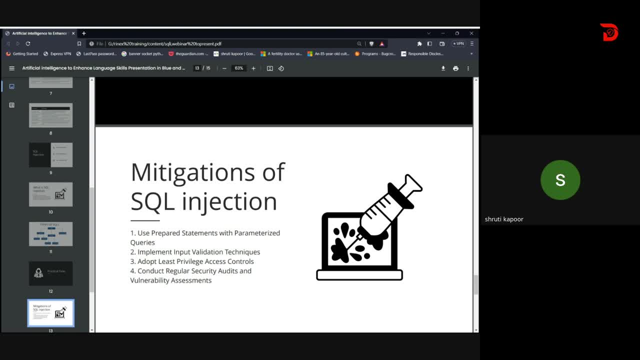 control. now, this means that, uh, that only a certain, only the minimum permission should be given to a person for for the task which he need to do. for example, if, uh, for example, if your task is only to read something, then i should give you only access to read. okay, then only the minimum permissions. 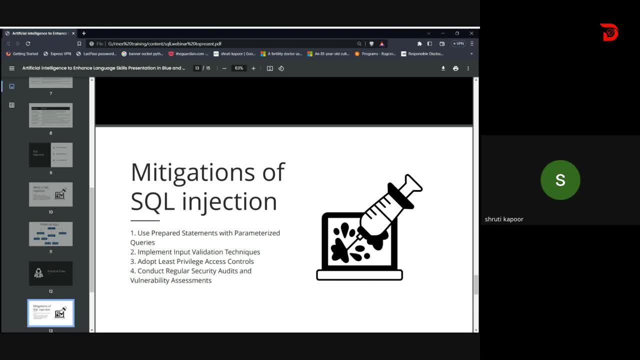 uh should be given to the person so that he will be able to do his task now. the next thing is that regular security auditing and vulnerability assessment is required so that we can get- we can get updated that whether a system is vulnerable to any of the vulnerabilities. 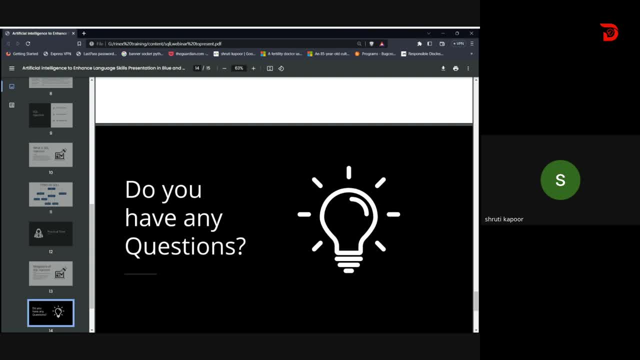 or not. okay, all right, so now. do we have any questions? now we'll address. so that was all there, uh, from my site for today. i hope you have understood something. so if you have any questions, so now we'll come to the uh answering the questions. okay, so now. 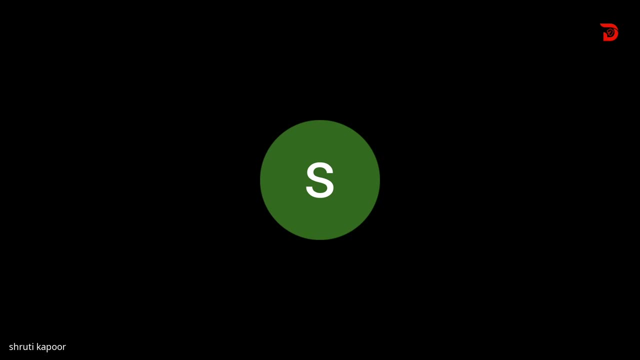 you people please start asking your questions now. you are open. uh, now i'll answer your questions. yes, okay so, yeah, so, uh, so we have, we have burp suit also and we have our zap also. we organization is a good tool because it has a lot of features. all right, no, okay, okay, so now. 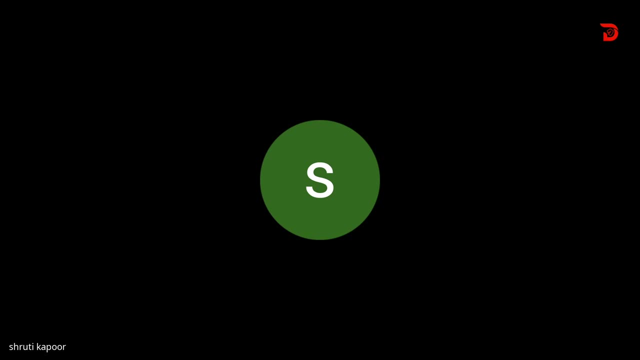 we'll come to job roles again. um, okay, so, jaeraji, i'll come to your question first. okay, so see, cyber security is a universe in itself. okay so, so, to be a cyber security person? so so it's not the case that every person who is employed in cyber security knows pen testing. no, it's not the case. 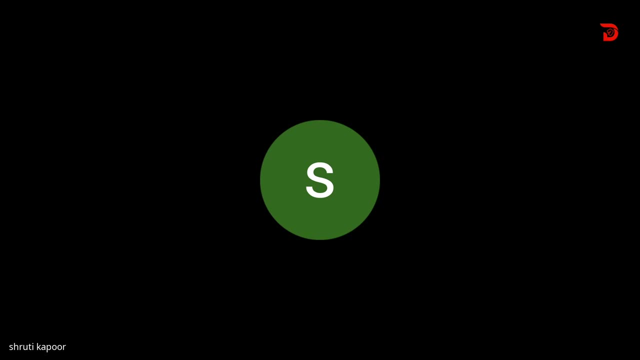 and even ethical hacking is not required for every type of role. there are so many roles uh like, like the security analyst role. so to be a security analyst, you should only know the basic, uh mean you should only have a degree in computer science and you should uh, and you should uh be. 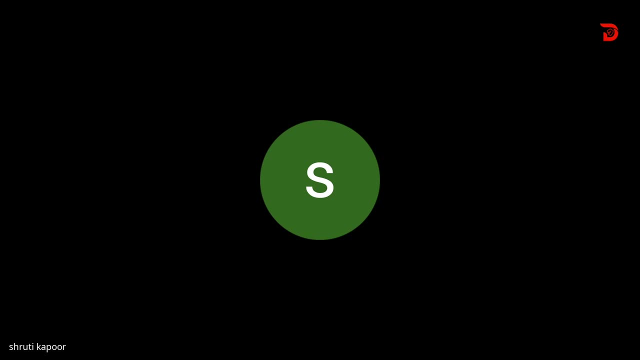 like, and you should be curious to learn something new. and you should have at least one certification in any domain: bhcc by isp square. even that certification is enough to uh, enough for you to get a job in cyber security. if you want to be a cyber security analyst, okay, um, all right, so uh. 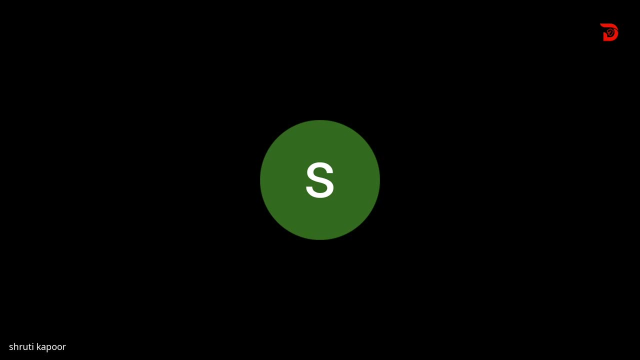 ravi. um, okay, so what you have not understood? okay, but i guess my screen size was fine with everybody. uh, now ramuda is asking: is degree from ip field is necessary? okay, so that thing also differs, uh, okay. so, uh, i had a friend, he did his bcom with 6gpa, okay and then. but he is oscp certified and he has done a lot of great certifications and he is placed in google with a package of 40 lpa okay. so there are a lot of uh exceptions companies. they want you to have a degree in cyber security. but even if you do not have that and you have a special degree in cyber security, i 기대 that. 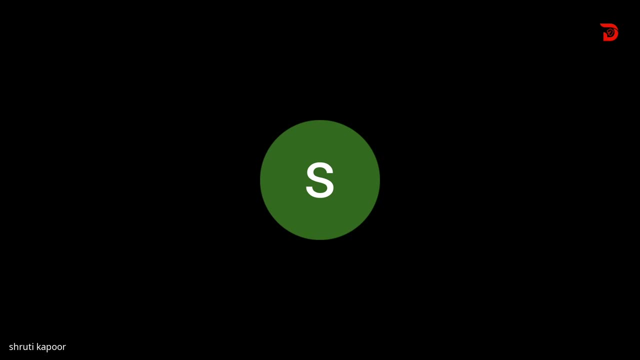 you have degrees in cyber security. but even if you do not have that and you have a special degree in and you have a specialization, you have a great knowledge of any domain- company will will yourself- I mean company will themselves- come to you and will offer you a. 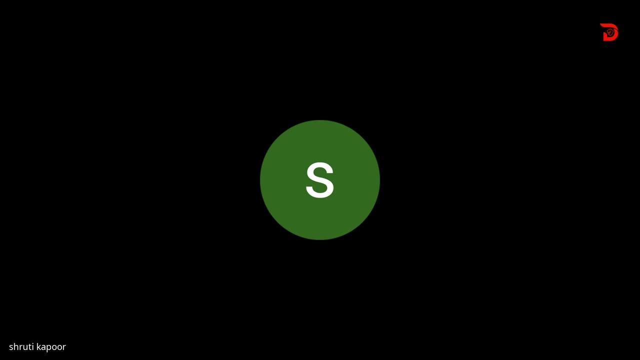 great package. okay, so now. somebody is asking how to inject SQL on any sql website. okay, so that, so. so steps for that thing is also same, okay, so see. okay, so now. okay, so now. but first I'll answer this question: can SQL map take down a website? yes, SQL map is also generating a lot of packets, see, that's why we are not randomly. 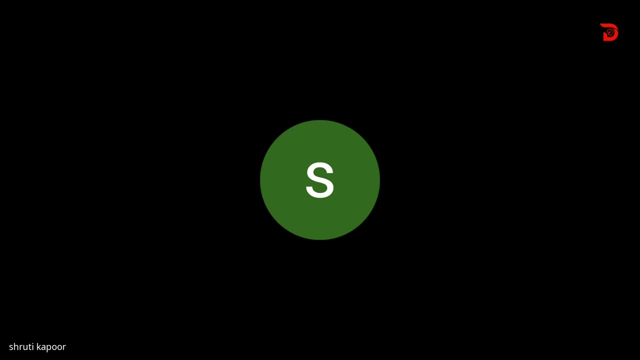 testing on any website. okay, we are only testing on that side, which is a domain site and is there for testing and whenever we will do testing on any site. so first we should have a written permission from the owner that you can do testing on this side. okay, like, because it. 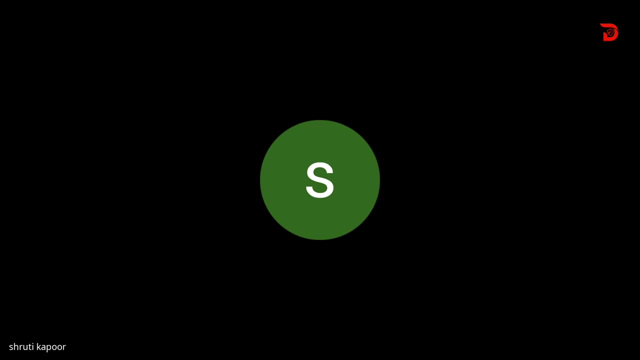 may happen that there is a weak site and if and if, like, yeah, at SQL injection, SQL map is also brute forcing the payloads right, so it may happen. that's why you should never test on any random website. first take the permission of the owner of the site and then do the testing work. uh, okay. so 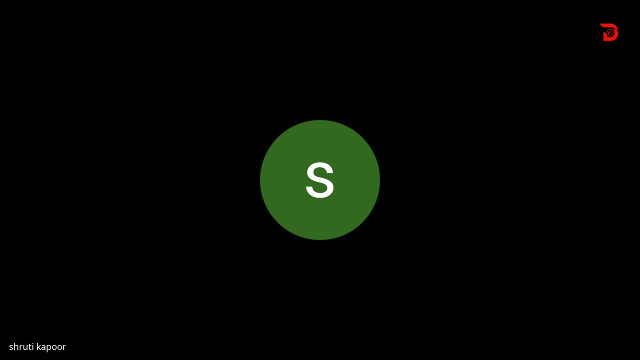 now the highest position in cyber security is of us. so or he can be a cto also. uh, now Vicky is asking: I have completed my 10th, not interested in science today. commerce will affect BTEC, okay, Vicky, see BTEC and DCA. so see uh, degrees, 80 degrees at. same level these days. okay, even there are a lot of universities who are, who are like, who are giving their detects for uh means a huge uh piece, but but still the packages which the people are getting they are. I mean, they are average only. so BTEC and BCA has no difference. these days you can go for BCA also. 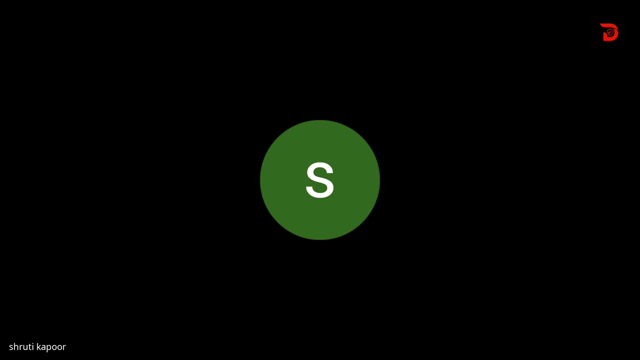 because, see I, because I personally feel BCA is better, because when you do BCA, uh, you will like your mind will go into a lot of directions, means you will have enough time to learn a lot of things. okay, um, so now HYCKR is asking: I need a job ready training because my degree completed after two. years. so probably it'll take me 3 or 4 years to complete a Direct atau you know, I don't know uh day and time. so in the meantime, if you are in an industry like civil, See, I am a freelance cybersecurity consultant and I am doing freelancing since past more than 10 months. 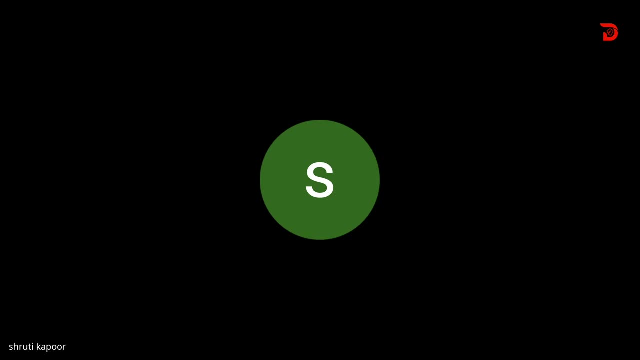 Okay, and I have a lot of clients from Singapore, Malaysia, So we can do freelancing work too. It is easy when you are in the cybersecurity domain, Okay. so Soham is asking CS or EGPT, Okay, so see, first you decide what's your interest. 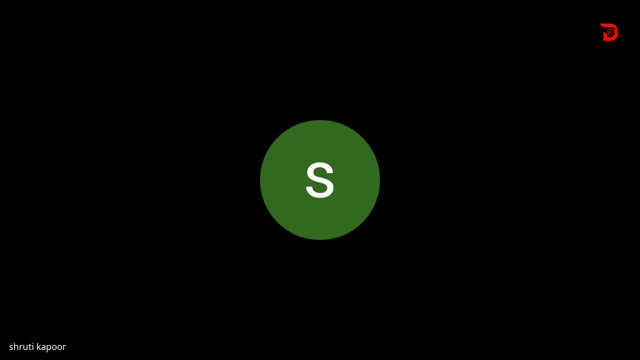 Don't rush behind EGPT, don't rush behind CEH. First you have to understand that where your interest truly lies, Because, like I told you, it's a very huge domain. here we have plenty of opportunities in cybersecurity, So you can start exploring a lot of domains like what's there in SOC theme, like what all are the same tools over there, what's there in consulting. 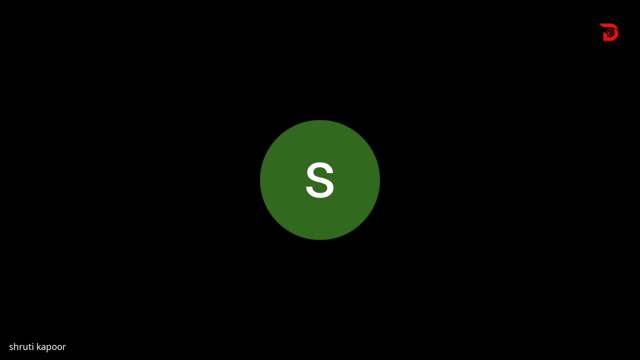 So first you should understand a lot of things- Even, for instance, CS is a good domain in cybersecurity- and then you choose your niche. Okay, so first understand basics of every domain, Ganesh. okay, so earlier certifications were very, very important to get you a job. 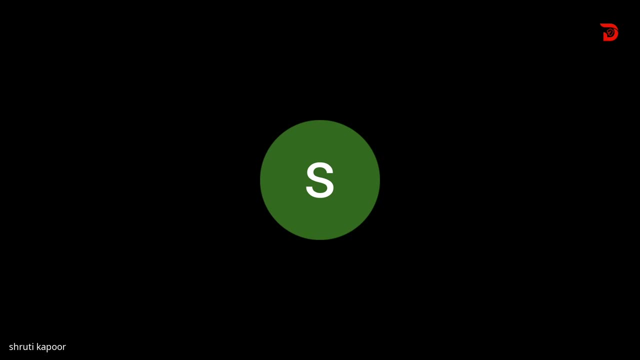 But these days certifications are important for resume and shortlisting, but companies, they have a separate test. Okay, for example, if you're applying for the role of a pen tester or any other role now, or a security analyst Now, in the second round you will be given questions on that thing. 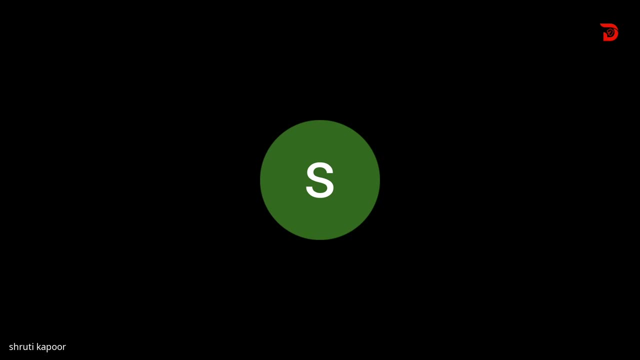 Okay, like if, for pen tester, you will be given a CTF on machines to solve, or if you are into analysis part, then they'll give you some scenario-based questions. Okay, Ganesh, Yes, BCA is a good option. 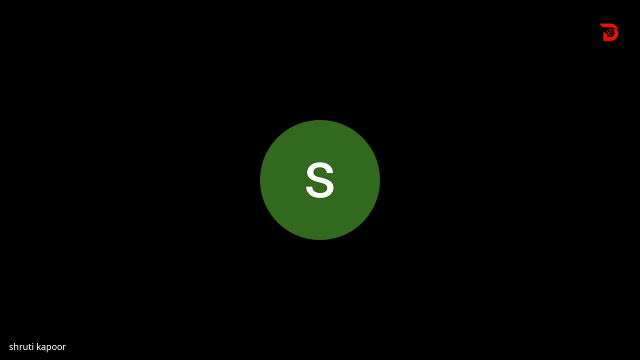 Okay, so for recording, I last saw, because I have no idea. Shruti ma'am, you have given a lot of interviews for corporates and cybersecurity companies, So can you tell them, like, what was your interview? work like interview, like steps, like what was the steps that was involved in your interview? 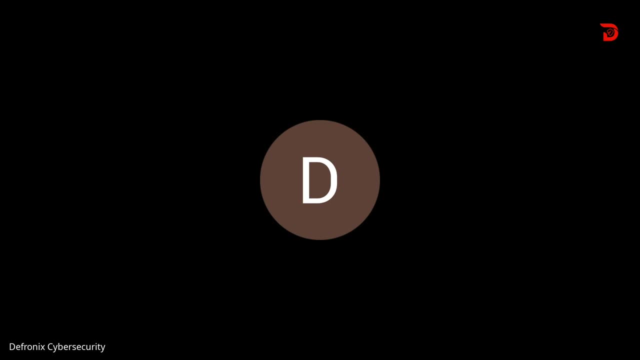 So that they get to know about the process, like from applying and to getting shortlisted and getting inside the company. Okay, sure, Okay, So, okay, Yeah. So the first thing is resume. So you should have a good resume where you should have the experience for the role you're applying for. 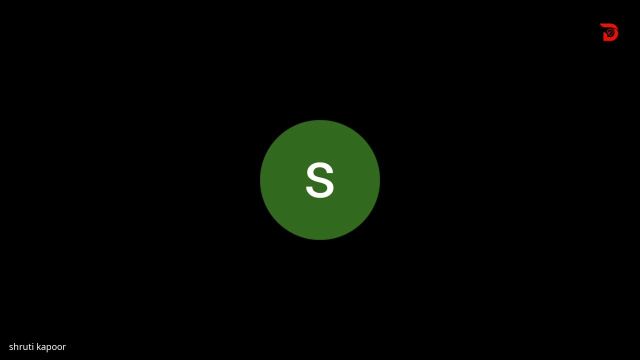 For example, if you're applying for the role of pen tester now, now in your resume you should have something which will tell that you are into pen testing- For example your certification. or if you are into bug bounty, then you should write that what all vulnerabilities you have founded and what all Hall of Fame SWACs you know what. 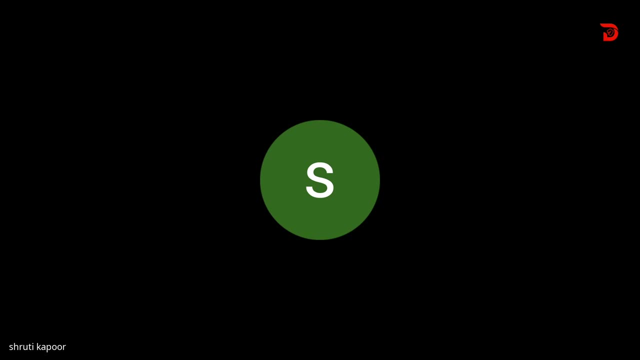 So that thing you have to mention in the resume, Because it is very hard in today's day that your resume will get shortlisted. So that's why you should write everything into your resume. And then the second: okay, now, now let's move to the rounds. 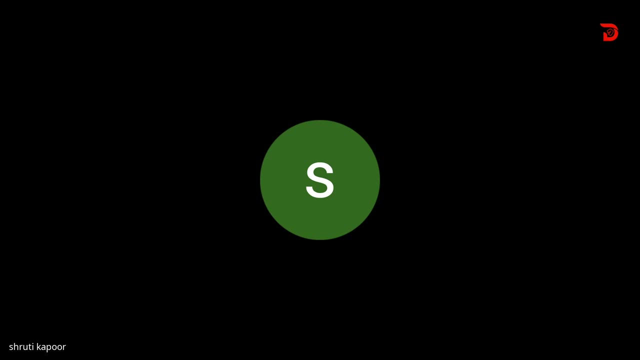 So okay, So so rounds differs from the company to company. So till now I have given a lot of interviews for a lot of positions, So okay, And now like so now I got selected in most of them, but in some of them I got rejected too. but I have experience of things. 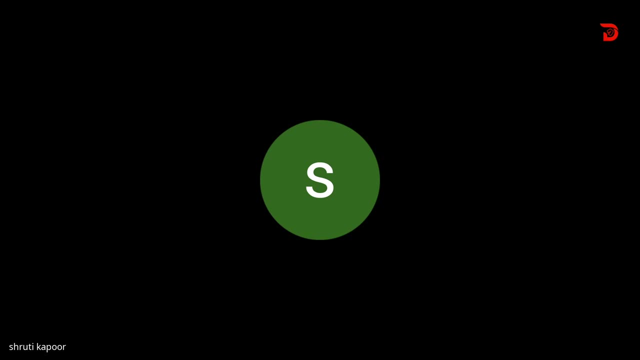 So now okay. so now to be okay now. so first discuss that how an interview for a security analyst is okay. So now to be a security analyst. the first thing, the first round, is our technical round, where they'll ask you the foundational questions like mean some basics of cybersecurity, like what is cryptography? 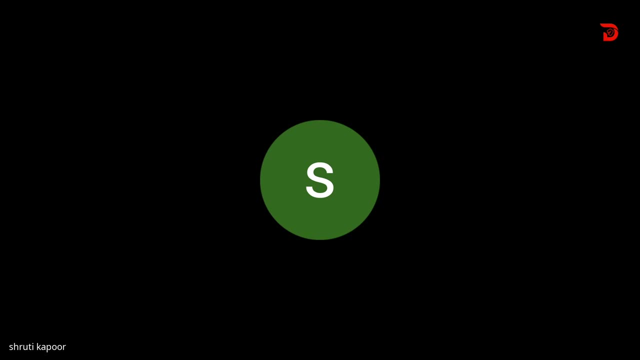 What is like? what do you mean by malware? What is ransomware? What you will do with ransomware will affect your system. So, like this, Some questions are being asked. Okay, And now. okay, And after that thing, there is a round two. that is also a technical round. 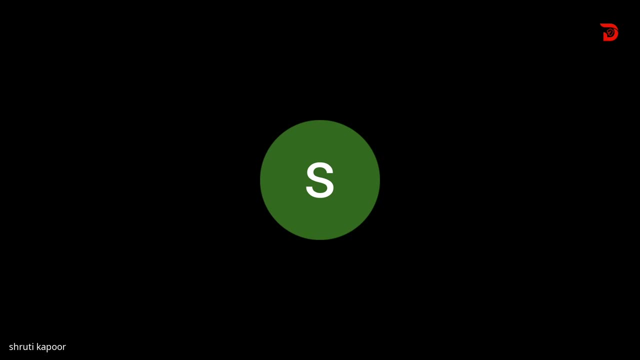 So they're. so they're like some team leads or technical team leads. They'll ask you the questions and that will be more detailed as compared to the previous round. Okay, And then, after these two rounds, we'll have a third round, and that will be a round with the director. 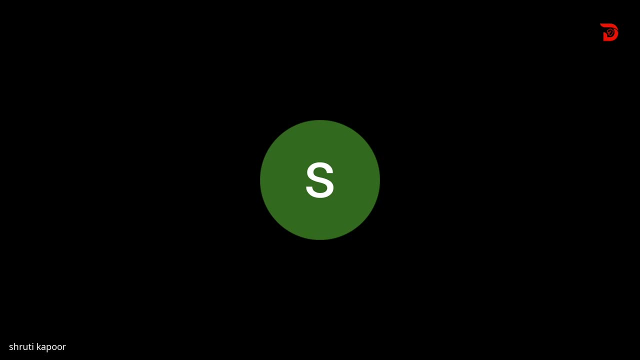 So that will be a managerial round. So in most of the companies it's the same flow When you talk about The job role of a cyber security analyst, So so, so they're basically. we have the three rounds, two technical rounds. 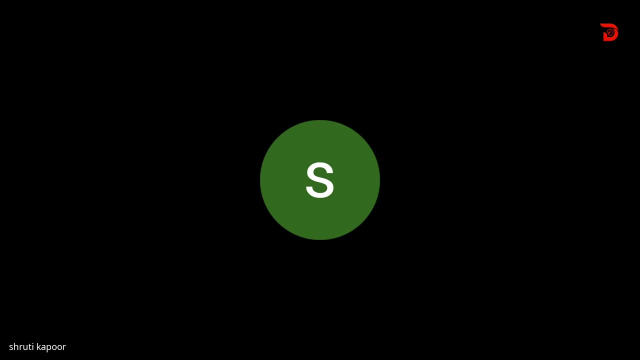 And then one is a managerial round where the manager will will ask you the questions that why you are into this. Okay, And I can. some normal discussion takes place in the last round. So this was for the security analyst. Now the second type of role is a pen testing role. 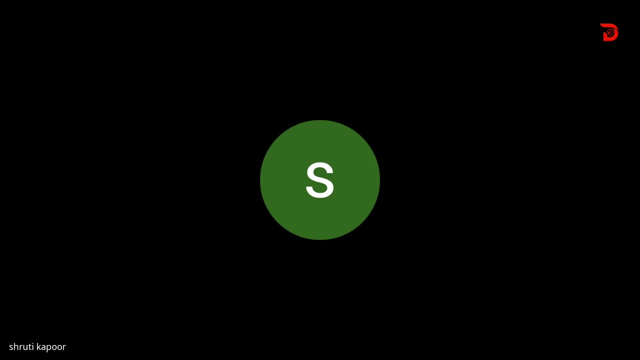 Now for pen testing role. The first thing is the okay. So now the first interview is a normal interview, Like we are. the technical questions are being asked about your experience. that that means whatsoever thing you have done, What's your project you have made. 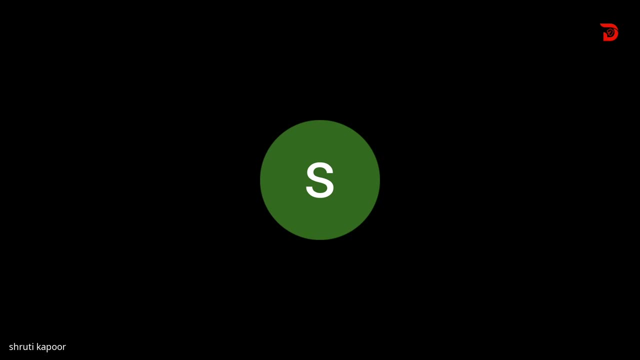 So, but that thing, the questions are being asked. And now in the second round you are given a CTF challenge When you are given a lot of machines to solve and you are given time of five to six days. So so it depends on company to company. 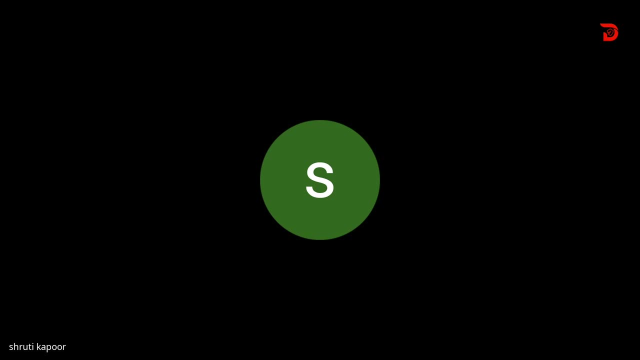 And then you have to, and then you have to solve with machines, and then you have to create the report because company You want to assess how are your reporting skills too Okay, And after that thing you have a third round. That is also the technical round. 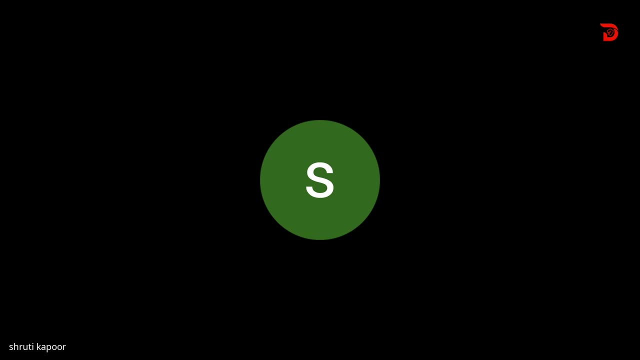 They are. whatever you have reported, That thing is discussed with the company And now the last round is around with the director. It's a managerial round here, where it's a simple one, where you, where manager, will only interact with you And the last act why you want to be like, like what fascinates you, to be a part of this company and like this. 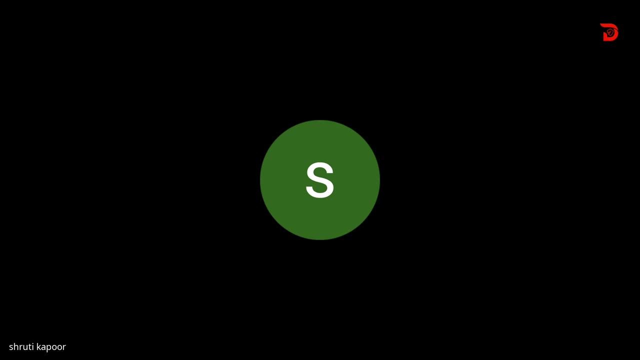 So it's a normal discussion Like: so they are the basically four rounds to be a pen tester, now, Okay, So now the third type of interview which I gave was to be a security consultant. So they are okay, So yeah. 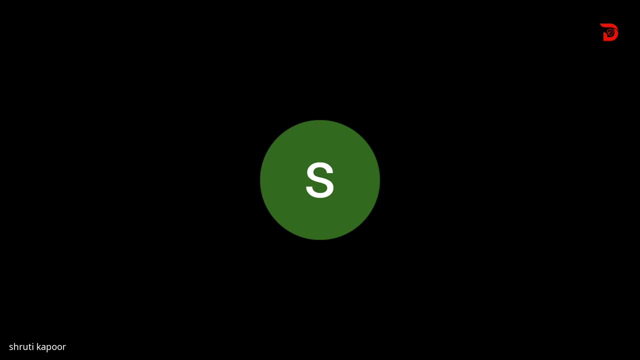 So far. so to be a security consultant I had. I had two rounds of interview. The first was the technical round And second one was also was the technical round, but that was with the CTO, And they also gave me a task like to write a security advisory, for that thing. 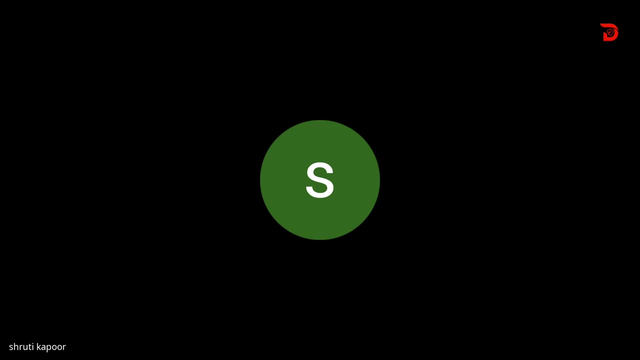 Okay And like, and they asked me whether I'm into research or not, So, so such type of things are being asked when you want to apply for the role of a consultant. So this is how my experiences were for for like, for working for a lot of companies. 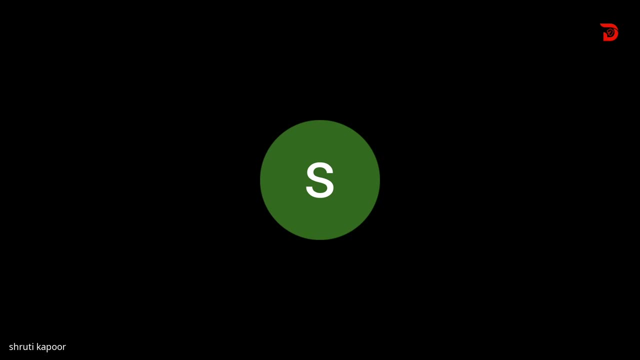 Yeah, So that's all about my experience. Yes, I'm from UPS. Okay, So to go into digital forensics? Okay, Yeah, So I don't have much experience of forensics. now for forensics, I guess, sir, we'll be able to guide you. 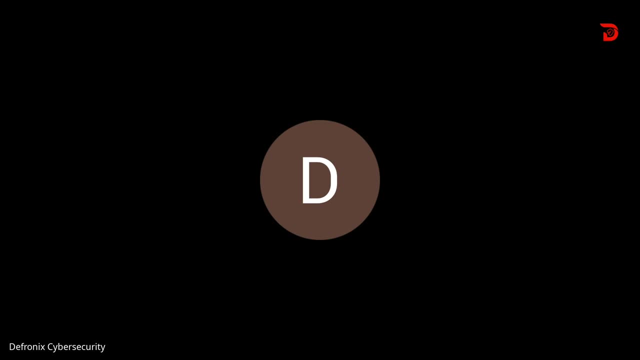 If you want to ask any question. like we will be ending the session soon, So if you want to ask, please ask. as a bug Hunter, can I focus only one or two vulnerability deeply or focus on or all vulnerability? Focus on all the vulnerabilities. 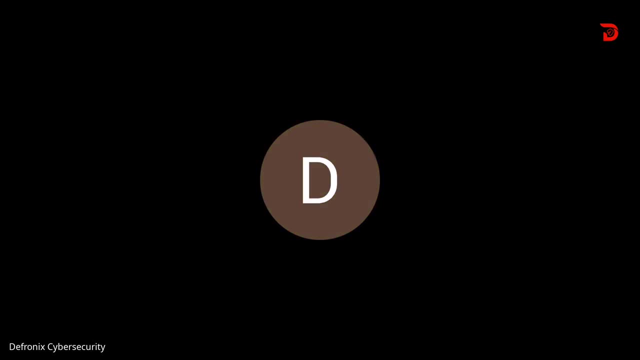 Yes, sir, Did you like the webinar? Did you like this webinar? Please let me know, Please let me know Everybody. You like the webinar by Shruti ma'am? If you like, if you like the webinar, then that's great, because we had a very limited time and we tried to deliver you all the like knowledge, all the things, all the information that we promised in the announcement video, and someone was asking for a training session. 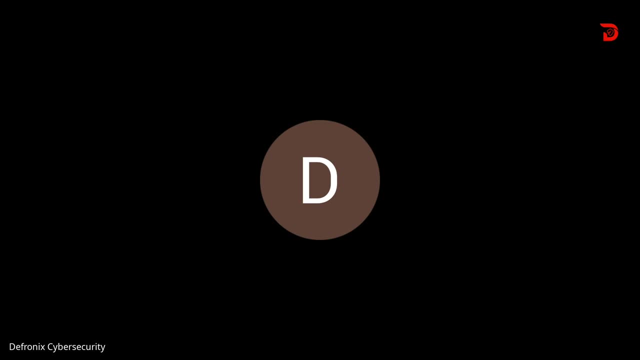 So yeah, we are going to bring a training session also, So don't worry about that. Like someone who was who was asking for the training session. So who was asking for the training session? Please let me know, Please, Please tell once again. 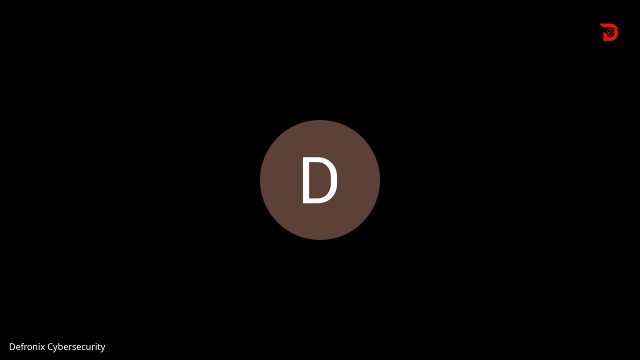 Someone was asking like, for a training. Okay, hiker, hiker V, great name, hiker V, So hiker V. Yeah, Vivek. Okay, Vivek was asking for a training session, So don't worry about that. I will be introducing you for with that also. 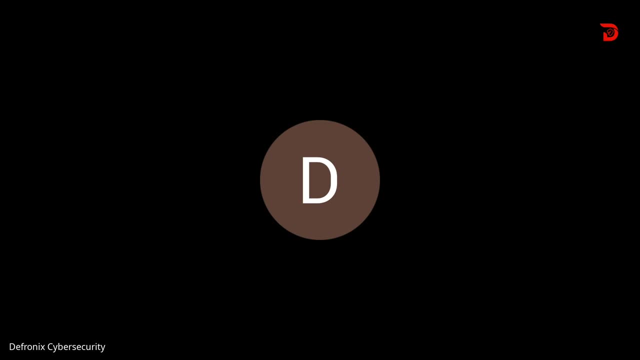 So so see guys, Shruti ma'am is has the Is doing like Masters, right, and I, if I'm not wrong, she is doing a like mtec, right. Am I right, mtec or MCA? No, no, So mine is MCA. cybersecurity forensics. 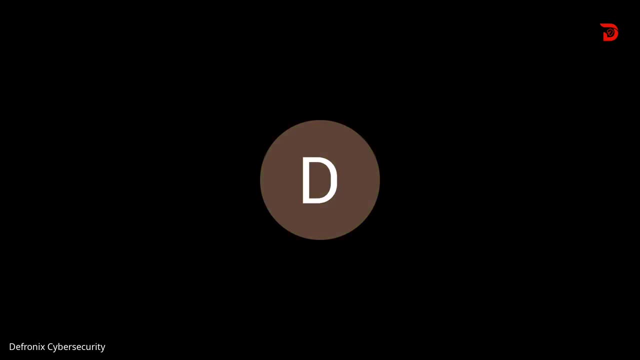 Yeah, So she is doing MCA- cybersecurity and forensics and- and she is an easy PT you all might be knowing, and she has been giving training to a lot of students already and she has also worked in Corporates. So we are thinking to start or launch a complete, complete, detailed cybersecurity training in English. 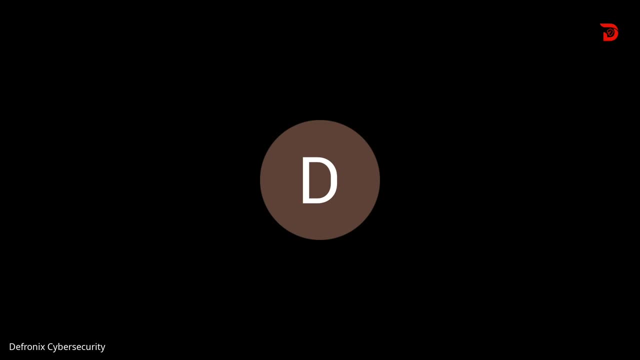 Yeah, totally in English. for all the students who are very much comfortable in English because the fronix has been delivering content from a very long period of time, Like when we were metaxone solution in name of a taxon solution. We are on the technical Navigator YouTube channel. 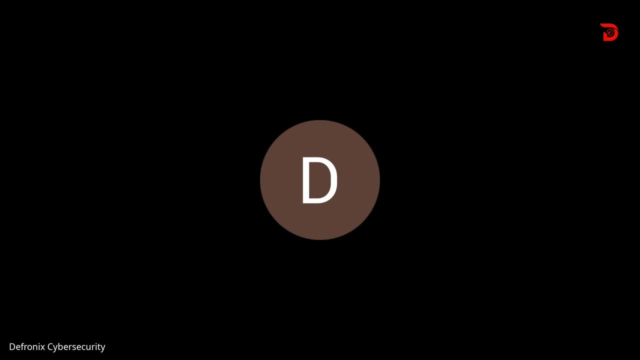 We all, we all were giving you all the contents in Hindi language. Okay, so we thought to bring the separate training, or very in-depth training, in English, because live training, it will be a live training. Just listen, just listen Whatever I'm saying, and everyone, everyone here. 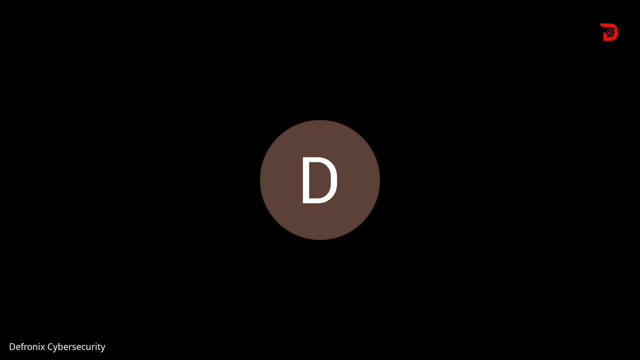 I'm giving you an, a security, like whatever training you are going to get, It will be like a, like a you out of your imagination, Like you can. you can just say it like out of your imagination, Like what? beyond your thinking, whatever you can say, live or record, 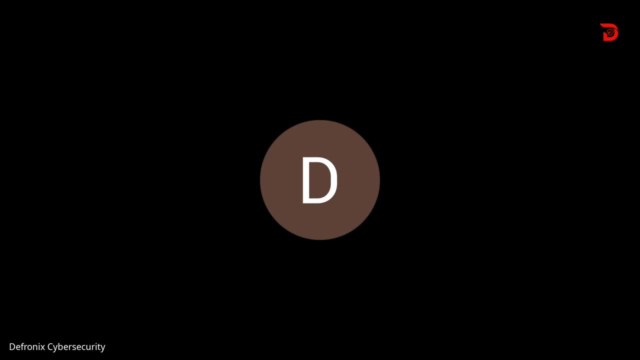 It will be live. It will be live, Okay, it will be completely loving. it is love you, peyote. So it will be completely live and it will be given delivering. It will be delivered by your shooting ma'am. So this is a type of DCSP program. 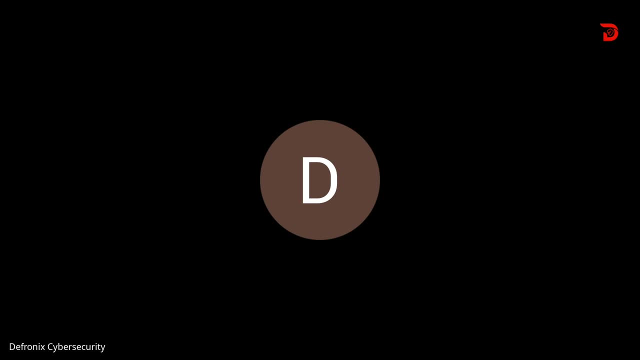 This is a type. This will be a type of DCJSP program defining certified junior security professional right. This will be a type of DCJSP, but in the English version. Okay, so see, let me share my screen once. Let me show you, please, then. 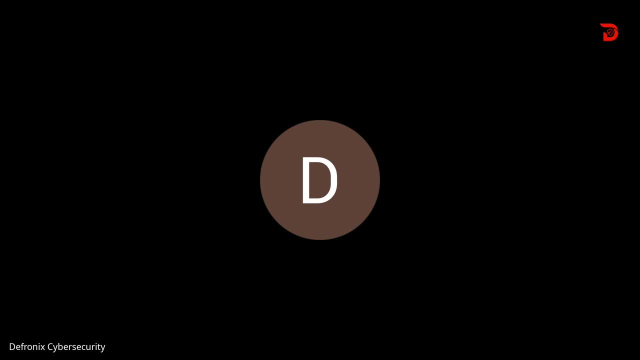 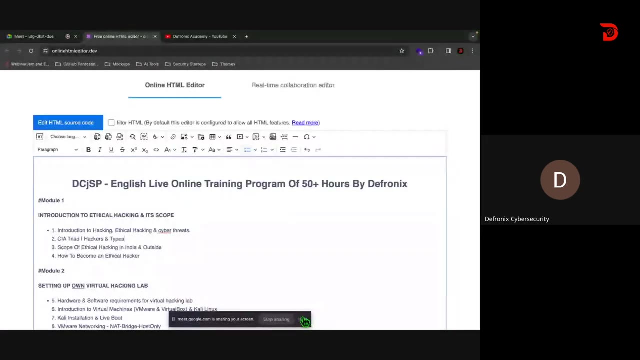 I think you will be better getting. let me show you the screen, my screen visible. guys, Everyone, please Let me know my screen visible. Yes, sir, Okay, Okay, Okay, Thanks. So see, so this is the training that we are planning to deduce. you all see. 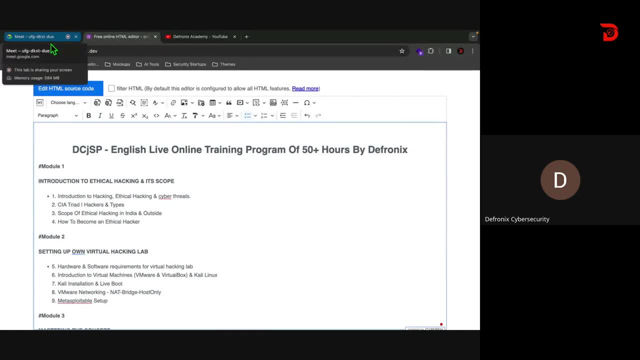 You all have to just stay in the group only for getting all the details about this training. We have not announced this training the date or like starting date or anything, but it will be a DCJSP English version live online training program of 50 plus hours. 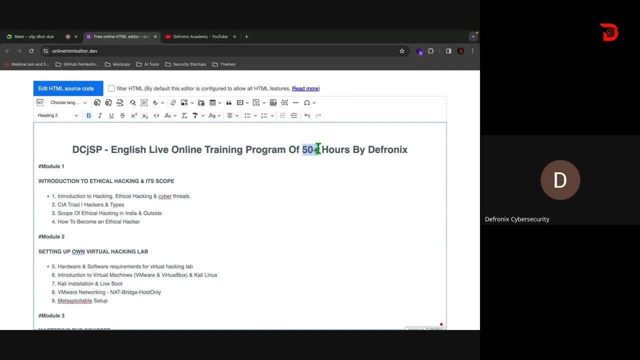 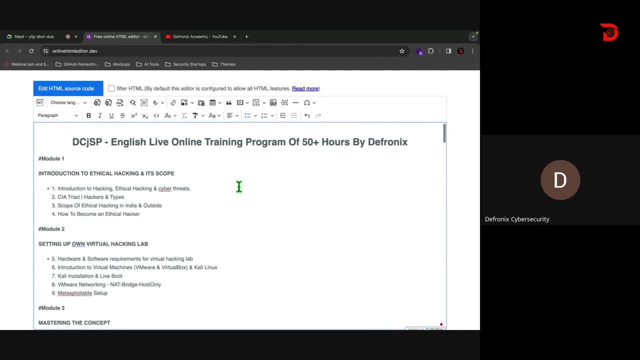 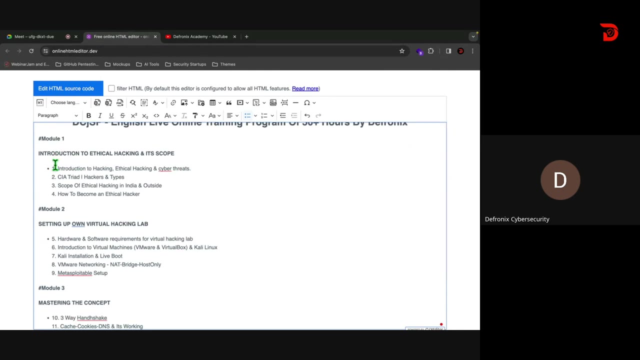 Like: this is a tentative hours that we have given you like, but around 50 you can assume right. So we will have a lot of modules inside this training and this will be taught by Miss Sruti Kapoor and this way, This is the module. like: this is a list of modules. 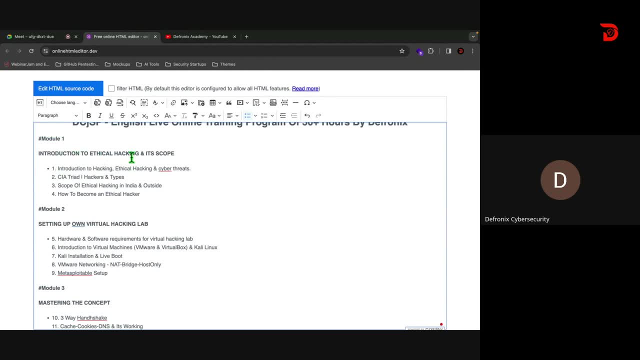 You can see here, like module one will be like: introduce introduction to ethical hacking and scope. module two will be like setting up your own hacking lab. three will be mastering, consume some of the concept that are listed here and some more can be introduced for will be like Kali Linux: from basic to Advanced there. 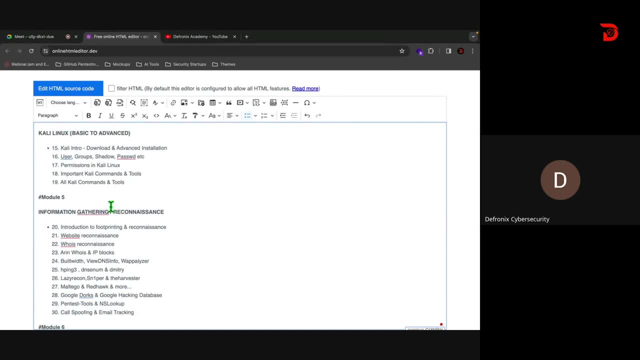 You will be understanding and getting information about all the Kali tools and all working of the Kali commands and all everything. then there will be Reconnaissance, there will be how to become anonymous, how to maintain anonymity using Tor proxy chain- like some intro to the Tor and dark web- and etc. 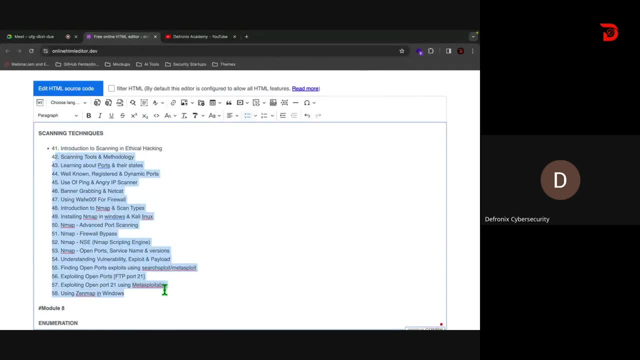 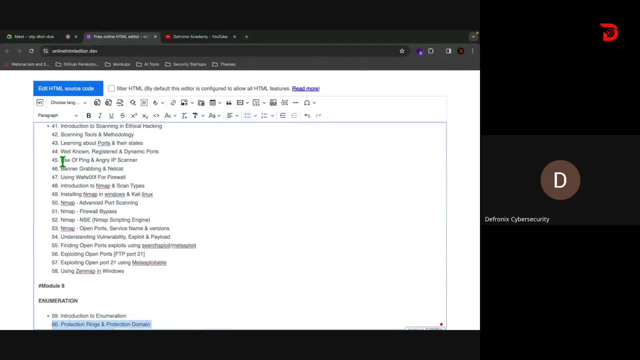 Now there will be scanning topic, like scanning topic. All these topics will be covered. Then we will have the enumeration: These are the hacking- phases of hacking. These are the phases of hacking, that that everyone have to go through. like whenever you are hacking or target, you have to go through these phases. 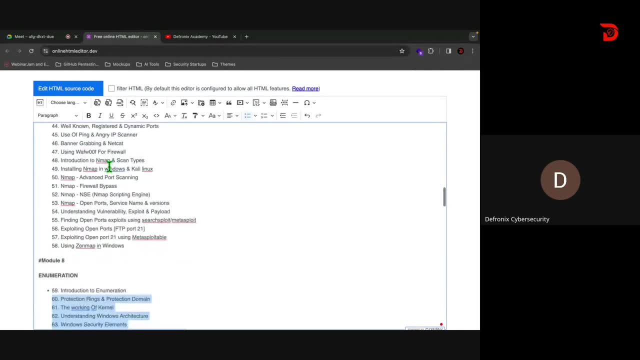 Okay, you will be doing Scanning, you will be enumerating, you will be fingerprinting, footprinting, everything to all the stages are introduced in this training. So after scanning, we will have enumeration. all these topics will be there. after that, system hacking will be there, password tracking will be there, and then you will be introduced. 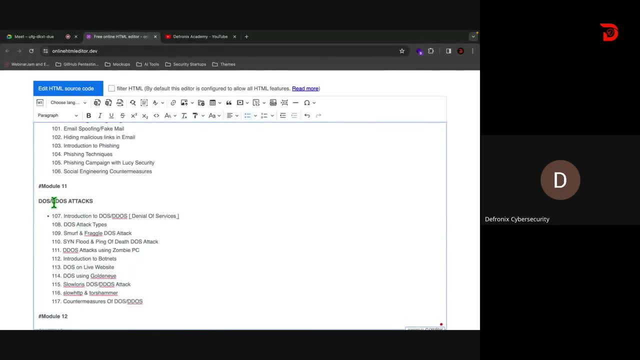 to social engineering, fishing and all. then we will have those and those tags and all the practicals part. then we will have the sniffing all the modules are like, filled with all theory and practical both, so you don't have to worry about that. then we'll have 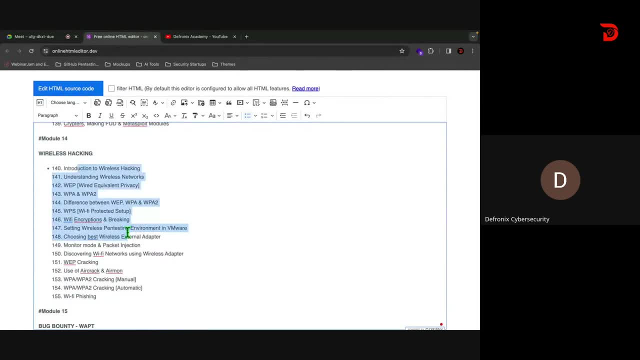 Metasploit advanced, and then we will have wireless hacking also and at the end we will have the bug bounty WAPT. like we'll be focusing on web application penetration testing for now. So we'll be covering a lot of vulnerabilities here, mainly from OSP top 10.. 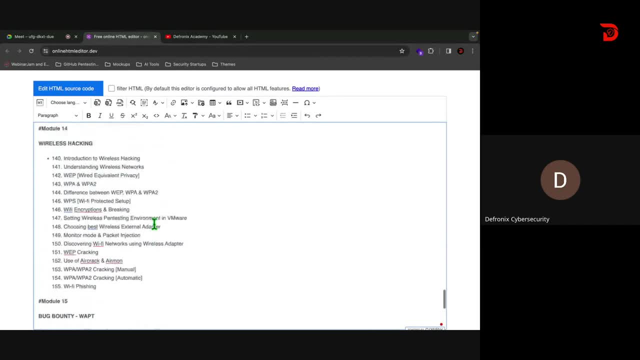 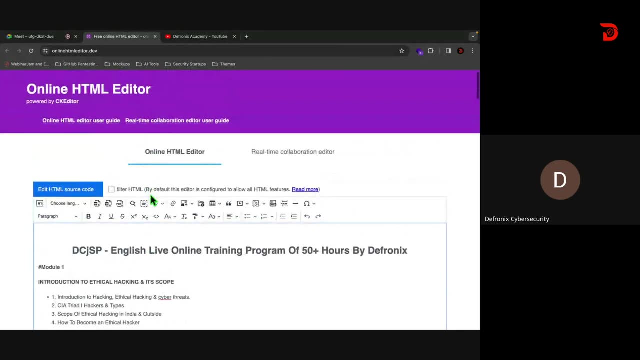 Okay, so we will be majorly covering OSP top 10 in this training program. Okay, so everything that is being given here will be taught to you- The training- in a very detailed, because we had maximum 90 minutes for this webinar, right. 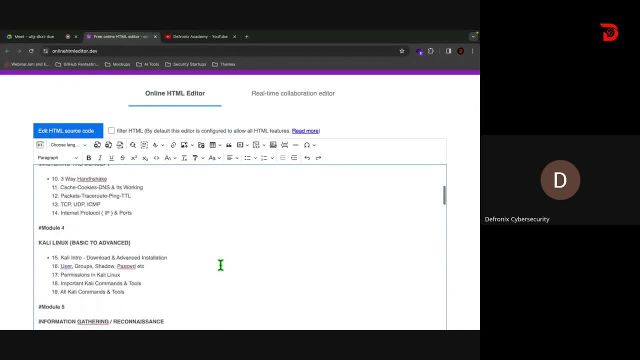 And in 90 minutes we cannot read or we cannot clear all the concepts, We cannot go to in depth for all the topics and all. so we have a plan, this training for you all in there, because many of you guys are already like, we're already demanding that. 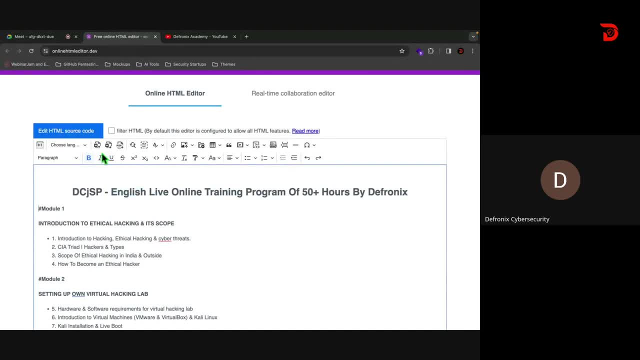 please bring the training session in English because we are more comfortable in English. We don't know or don't understand Hindi language, So we are bringing it right on your demand only. and this is the certification program name: DC GSP, like the foreign certified junior security professional. that certification you will be getting after. 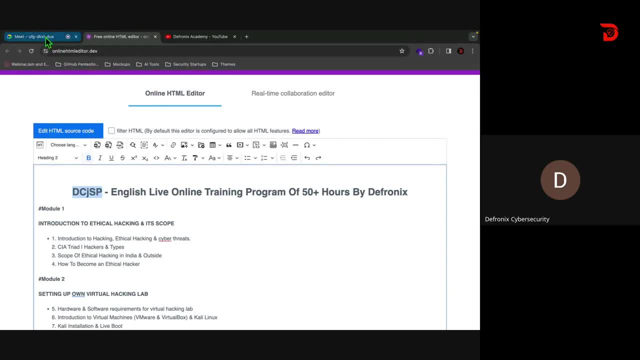 completing this training. Okay, so there will be a short exam after this training, or MCQ based exam, that will be related to your training only, and after that you will become a DC GSP. Okay, So, yeah, that's the training part. 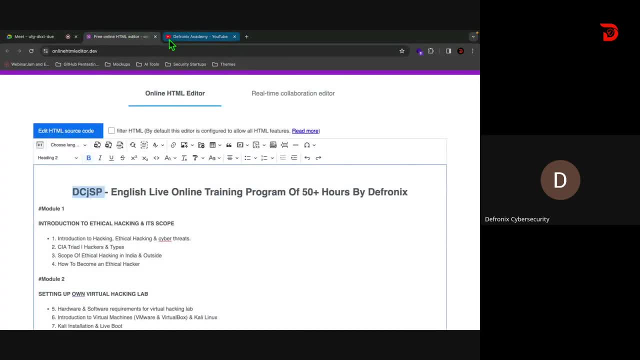 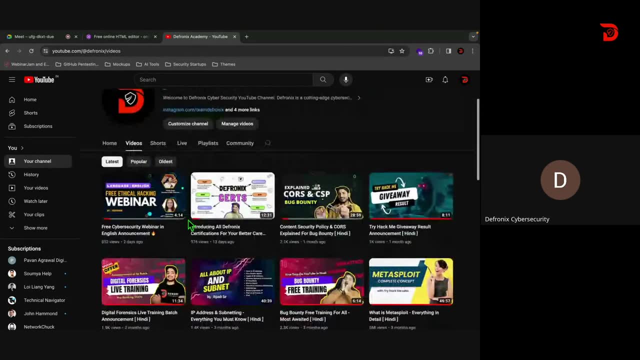 That's the announcement of the training part and the announced detail announcement. batch start day: It and the any fee structure or anything will be coming to the phonics Academy YouTube channel. Okay, and the tattoo and on our defronics Academy YouTube channel also.